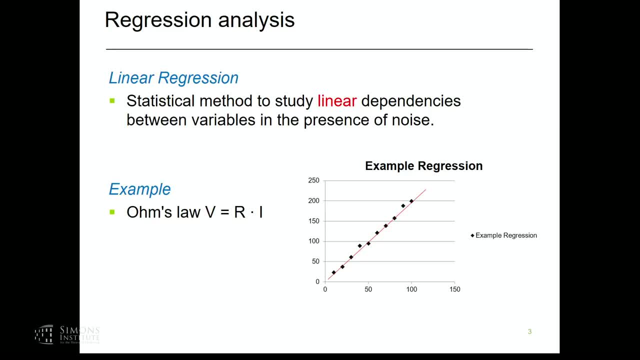 So here it's just the unknown slope or the resistance, And there are many different notions of what it can mean to best fit something. Oftentimes there's no line that goes through all the points. I mean you have noisy data, etc. 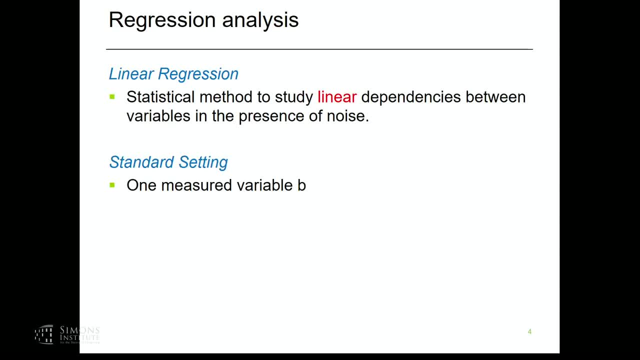 Okay. So just to set up some notation, in the standard setting we typically have one measured variable, b- This was the voltage on the previous slide- And we have some number of predictor variables, a1 through ad. Okay, so d was equal to 1 on the last slide and a1 was just the current. 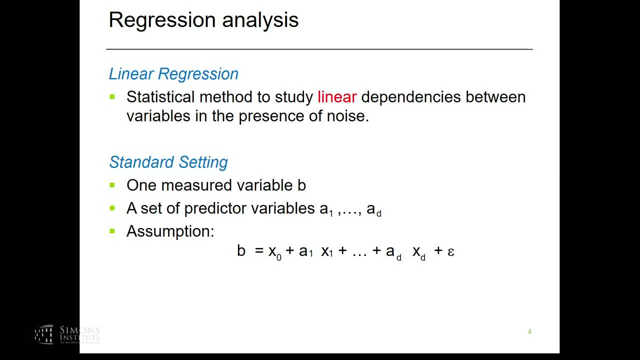 And the assumption is that these variables are linearly related up to some noise. So we have the relationship that b is equal to some unknown x0 plus a1, x1 plus dot, dot, dot, ad, xd plus some noise- epsilon. Okay, And so we're trying to learn these values xi, which are sometimes called the model parameters, and 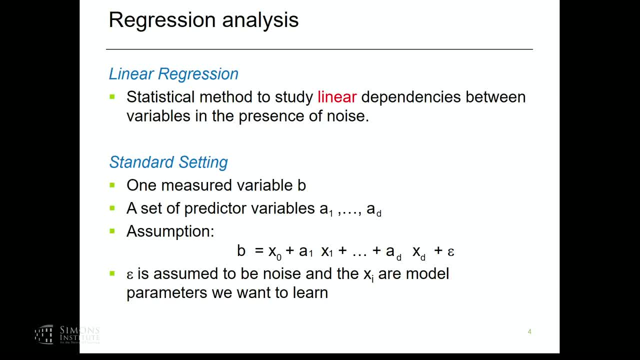 we don't want to make assumptions about this noise epsilon if we don't have to right. If we can get more robust algorithms that work for, you know, arbitrary noise settings, this would be ideal. Via standard transformation, you can assume that this x0 term is equal to zero. 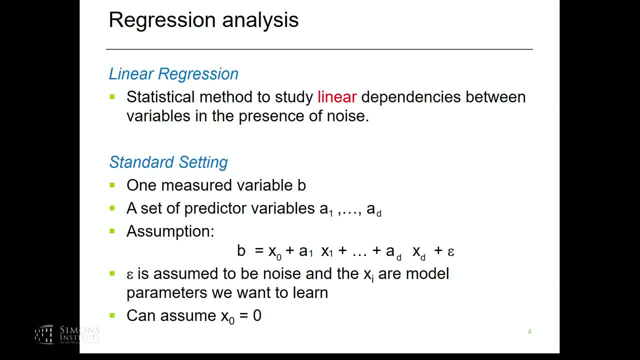 So to do that, one thing you can do is you can replace d with d plus 1, and you can have- imagine an a0 term here which is always equal to 1.. So let's just forget about x0.. And we don't just get one observation. in regression, We had all these points in the Ohm's law plot. We get n observations. 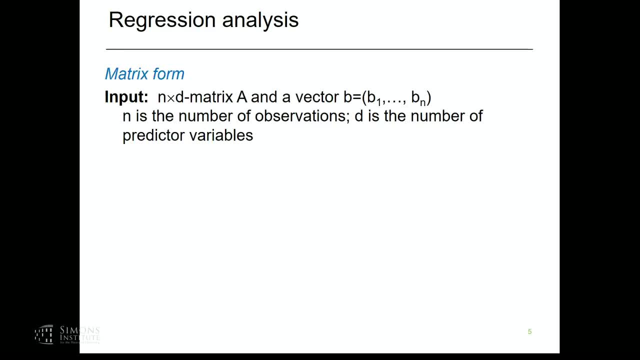 So let's write our problem in matrix form, So we can think of being given an n by d, matrix a: the rows correspond to examples or observations and d is the number of unknowns. We're also given this n by one vector b of observations. 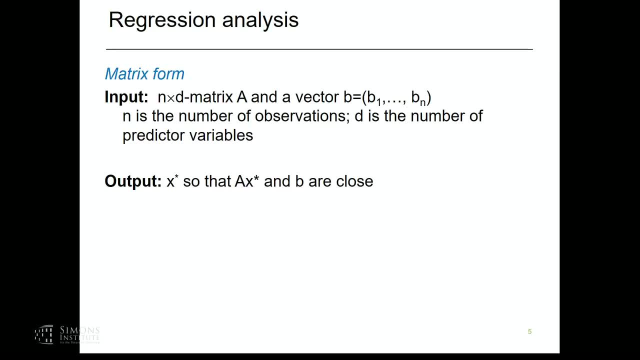 And the regression problem just asks to find this d-dimensional vector x star, so that a times x star a is n by d, so this will be an n by 1 vector. a times x star and b are close under some notion of closeness. 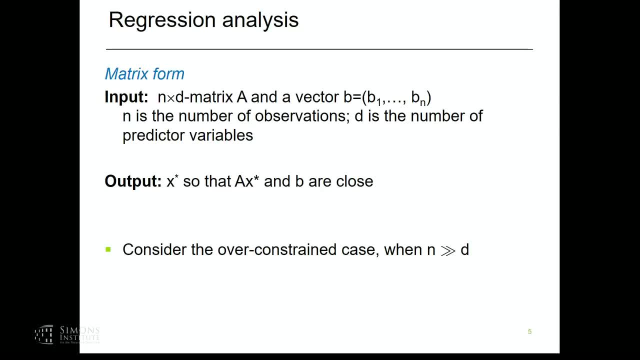 Okay, We're going to consider the over-constrained case when there are many more examples than unknowns. N is much larger than D. A is a tall, thin matrix. So, yeah, what does it mean to find the line that best fits the data. 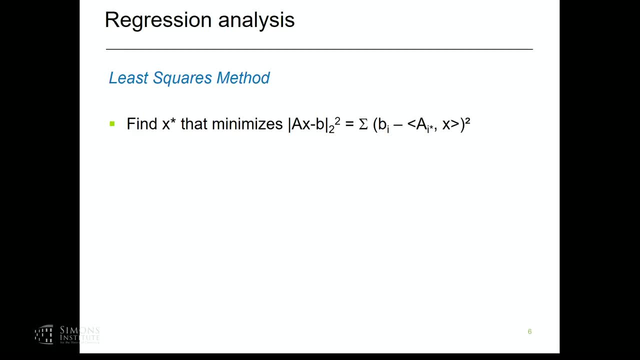 So let's first look at the least squares method. So here what you want to do is just find this vector x, so that the Euclidean distance between AX and B is minimized, or equivalently, the squared distance. Okay, so this is the sum over the observations. 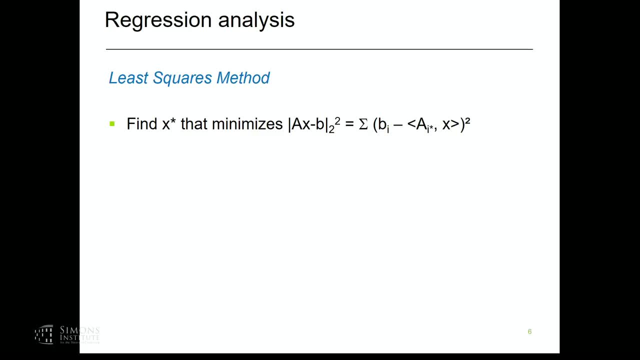 of what you observe, minus you can think of as what you predict. okay, the inner product of the i-th row of A and your chosen vector x, squared. Okay, so this has certain desirable statistical properties. For example, if this noise epsilon being added. 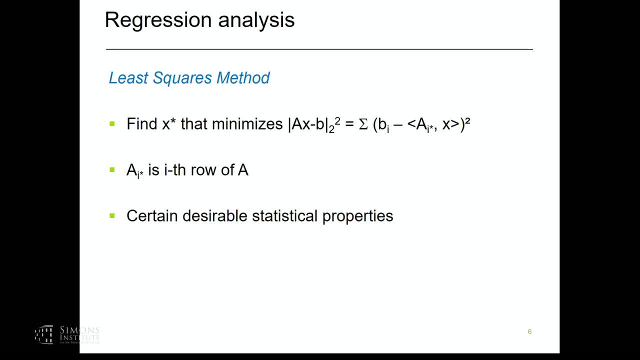 to each of your observations were IID Gaussian noise, then actually finding the x that minimizes this objective function would give you the maximum likelihood estimator. Okay, It also has a nice geometric interpretation, right. So the least squares objective function. we can write A times x, as you know. 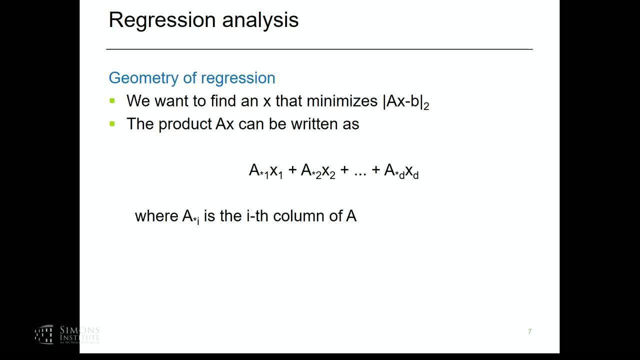 linear combination of the columns of A right. So as I range over all x, I get all linear combinations of the D columns of A. I can think of this as a D-dimensional subspace of R to the N, So D is. I'm sorry. 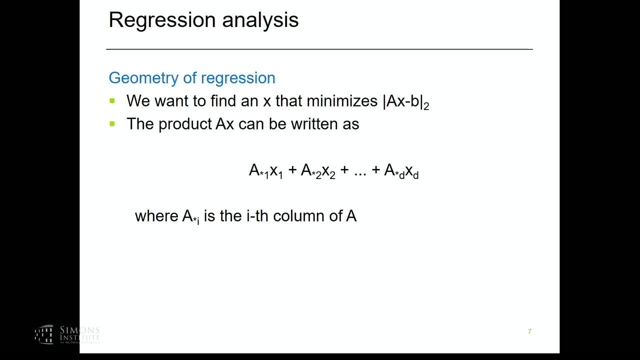 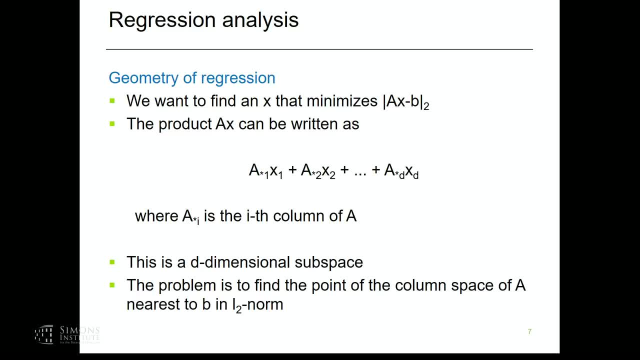 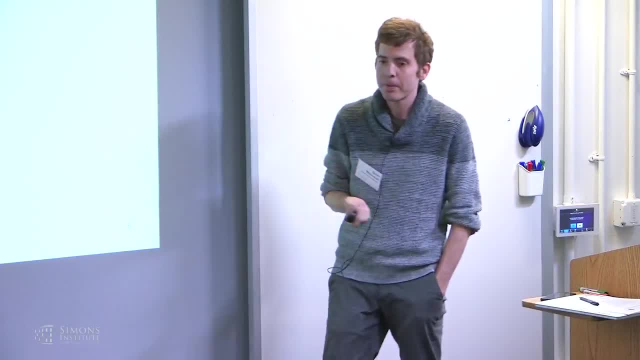 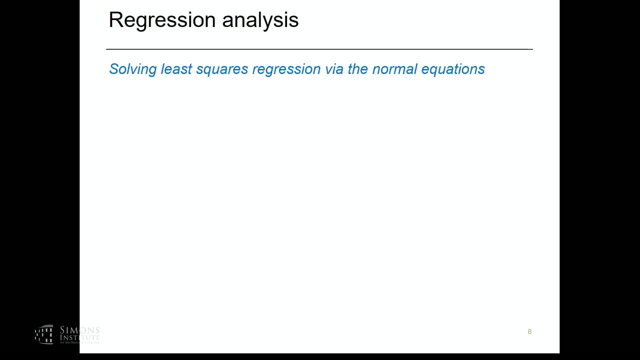 which is closest to B in Euclidean norm, right? So it's just the projection of B onto the column span of A. Okay, Another nice property about least squares is that there's a nice closed-form solution So we can solve. we can solve least squares via the so-called normal equations. 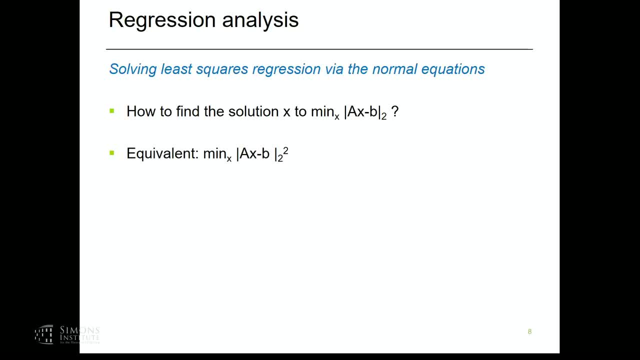 So how to find the solution? Well, let's look at the least squares: objective function or, equivalently, the square. So let's write our vector B of observations as A times x prime, for some x prime plus B prime, where B prime is orthogonal to the span of the columns of A. 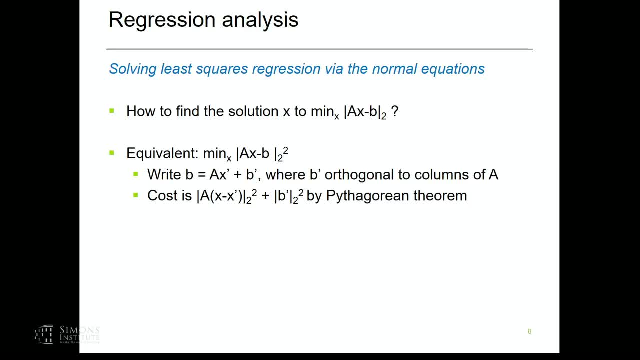 Then the cost by the Pythagorean theorem is just the squared cost of A x minus A x. So we can say x prime plus the squared norm of B- sorry, of B prime. And so for any solution, x that you might choose. 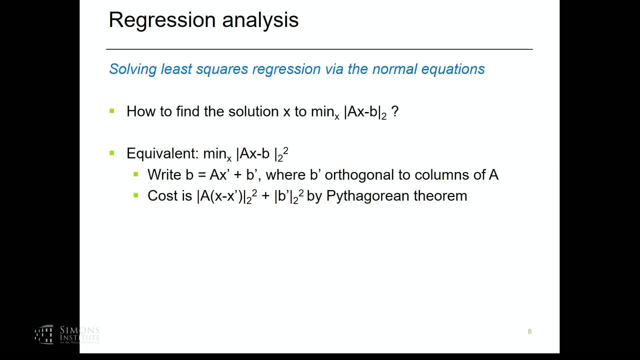 you know, any x you choose, you're going to pay this projection distance, the norm of B prime. So really, what you want to do is, you know, just make this first term equal to zero. And so x is optimal if, and only if, it satisfies. 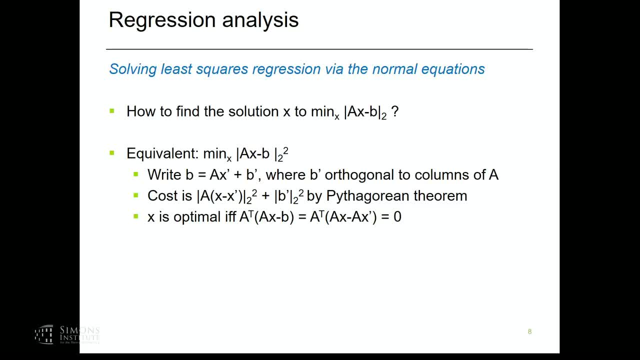 the so-called normal equations. Okay. So what this means is you know. so let's look at A transpose times: A x minus B. okay, And I can substitute in this expression that I have for B, And so I'll get A x minus A, x prime minus B prime. 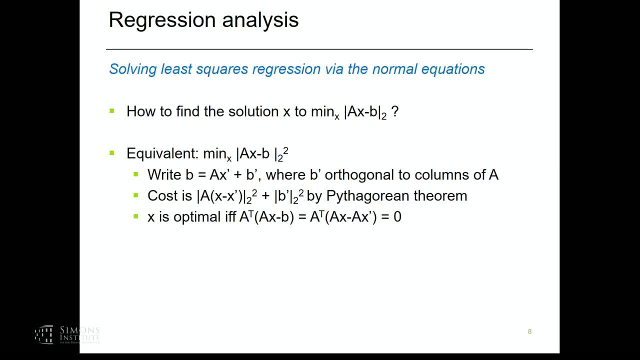 And we know that B prime is chosen to be orthogonal to the columns of A, so orthogonal to the rows of A transpose. So this is just equal to A transpose times A x minus, A x prime. And we know that if we're optimal, 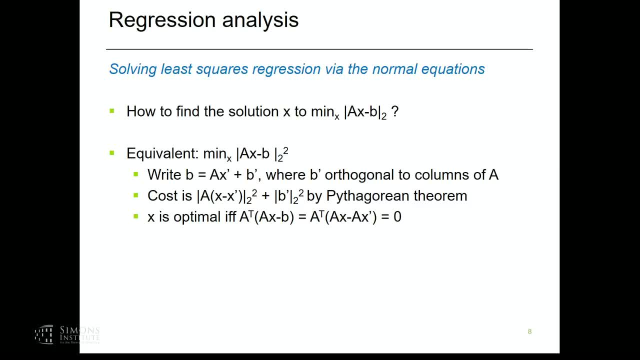 that this A x minus A x prime, this norm should be zero. Okay, so A x minus A x prime is zero and we get zero, And conversely, if it's not zero, if A x minus A x prime is not zero. 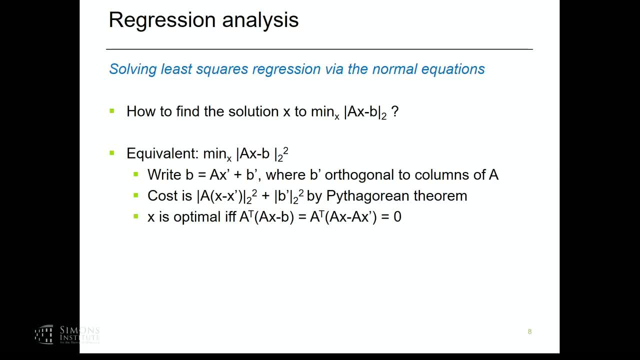 since it's inside the column span of A. you know, it has a non-zero dot product with one of the rows of A transpose and this would be non-zero. Okay, So the normal equation is just that A transpose A, x equals A transpose B. 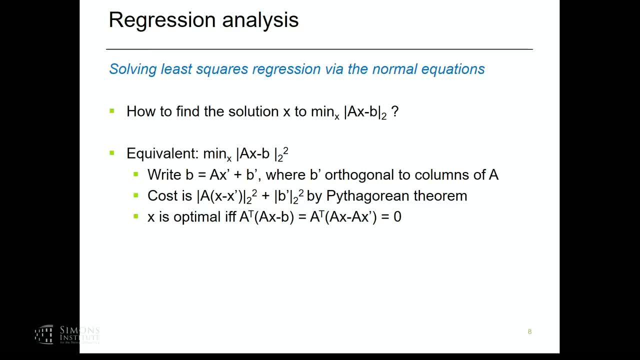 Okay, I mean equivalently. you know: A transpose A, x equals A transpose B. Okay, Okay, Okay, Okay, Okay, Okay, Okay. So equivalently, you can think of this as looking at the gradient and setting it to be zero. 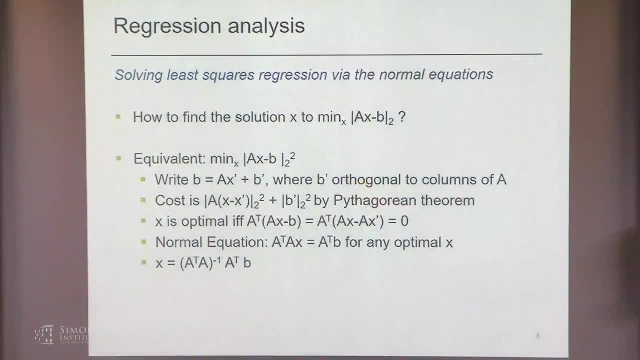 Okay, So that's the normal equation, And the nice thing is, if the columns of A are linearly independent, then I can just write down a closed-form solution for x. All right, It's A transpose A. inverse times A transpose B. 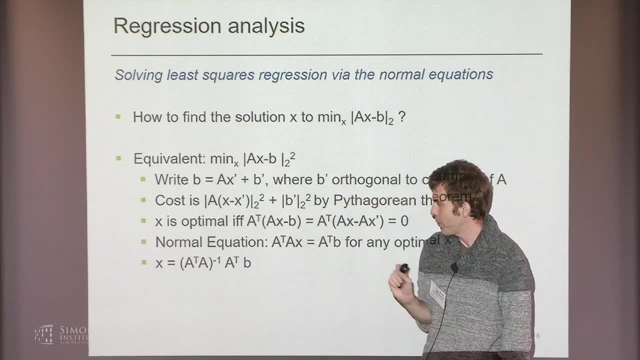 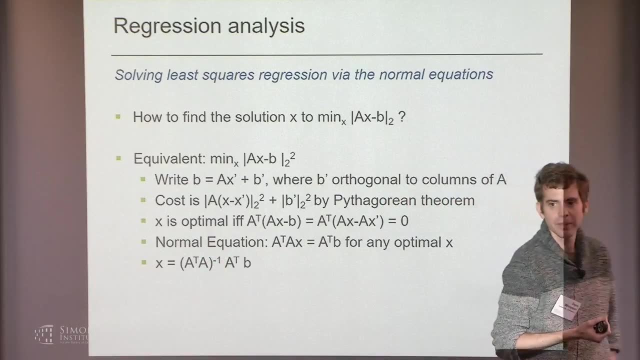 So the problem with this is- you know that I'll get to more- is with computation. So, as Ravi was discussing, you know computing A transpose B. you know computing A transpose A is expensive for large matrices. Okay. 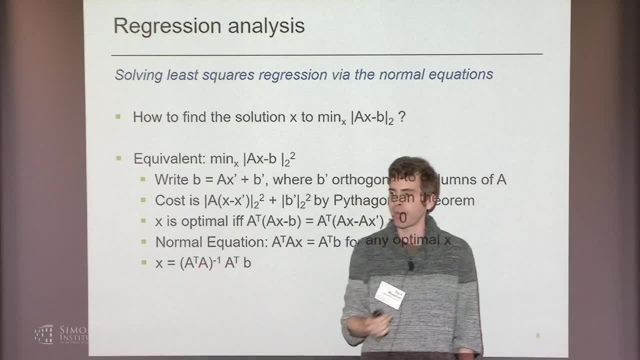 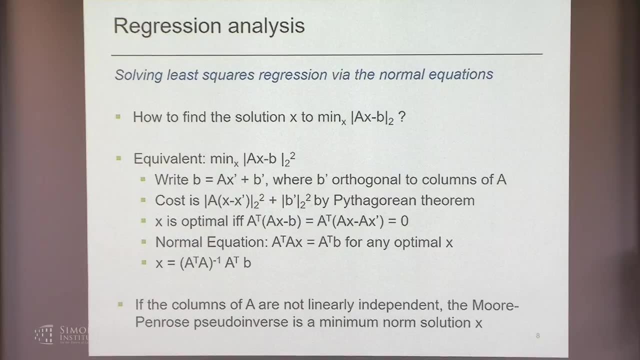 So naively. this takes n d squared time. You can do a bit better with fast matrix multiplication, but we want to do much faster. Okay, Just one thing to note here is if the columns of A are not linearly independent, then there's more than one solution. 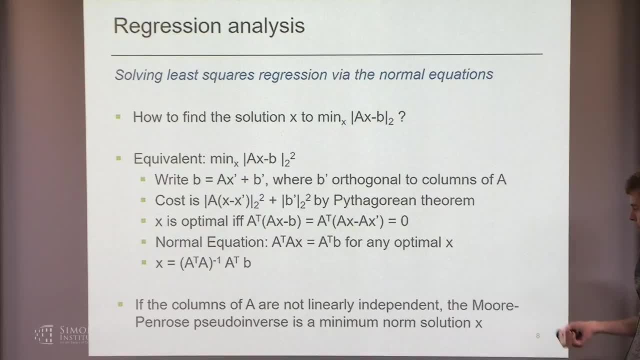 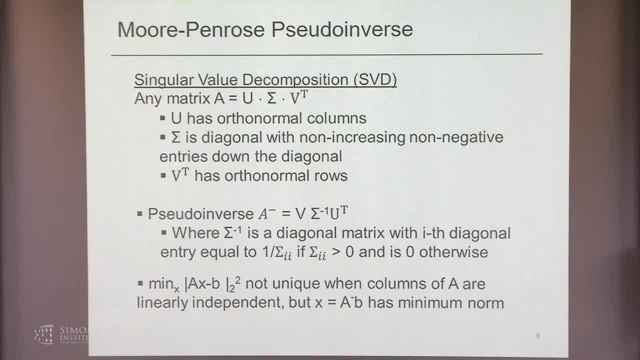 Which I think Ravi mentioned in a response to a question, but I don't think it was formally defined, so let me just say it. So recall the SVD that Ravi mentioned, that every matrix A can be written as U sigma V transpose: 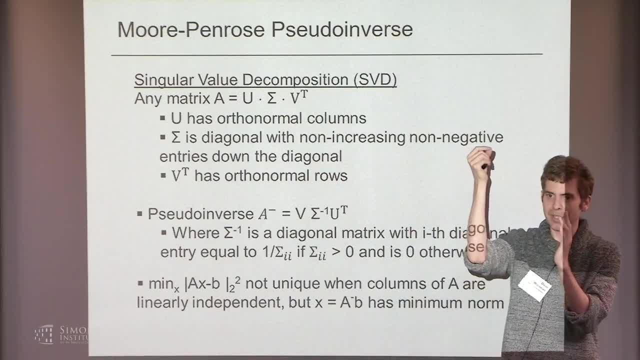 U as orthonormal columns. sigma is, you know, non-negative diagonal, and I'm non-increasing as I go down- and V transpose as orthonormal rows, Then the Mohr-Penrose pseudo-inverse, A superscript, this minus. 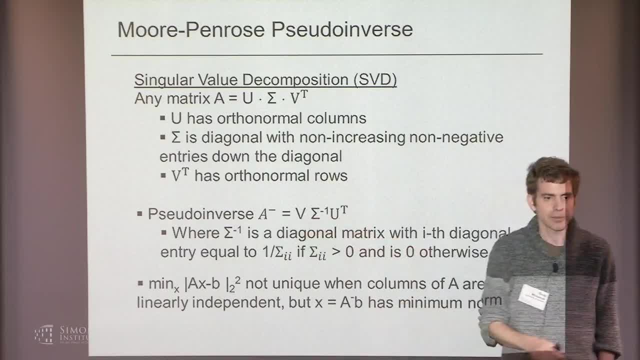 then the Mohr-Penrose pseudo-inverse: A superscript, this minus. then the Mohr-Penrose pseudo-inverse, A superscript, this minus. there's just V, sigma inverse, U transpose Where what is sigma inverse? Well, it's a diagonal matrix where the i-th diagonal entry. 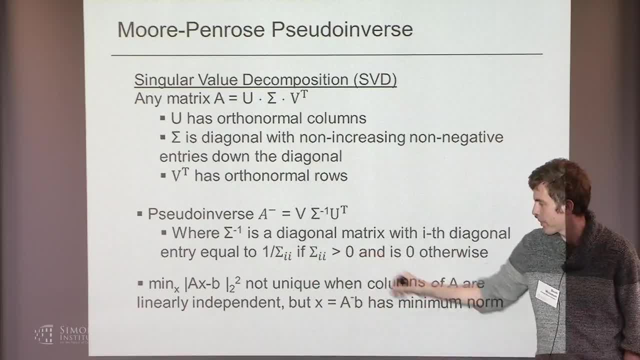 is, you know, 1 over sigma i i, if sigma i i is greater than zero and otherwise it's just equal to zero. Okay, So, yeah. so if you, if you write X to be the pseudo-inverse of A times B. 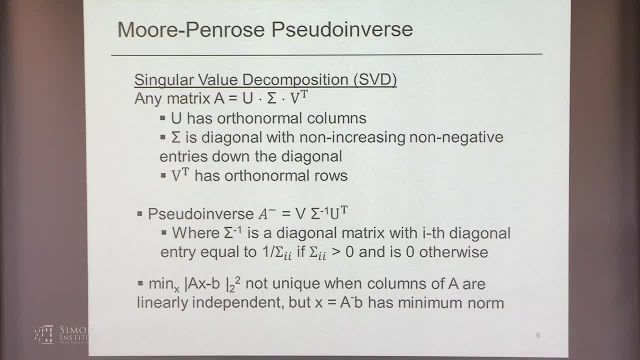 then this is a solution with optimal cost, with minimum norm. Okay, Okay, Thank you. Thank you Now. computing the SVD also takes, you know, n d squared time, or you can use fast matrix multiplication for that as well to get a bit better. but we'd like to do a lot faster than this. 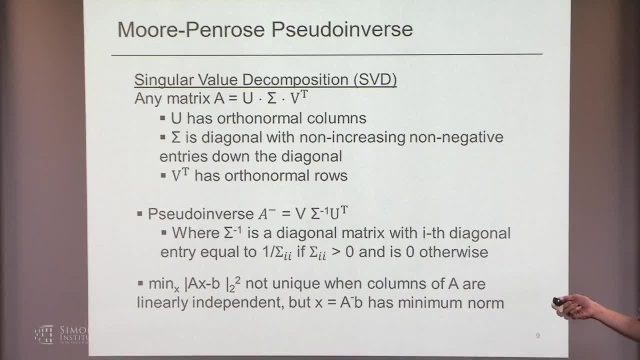 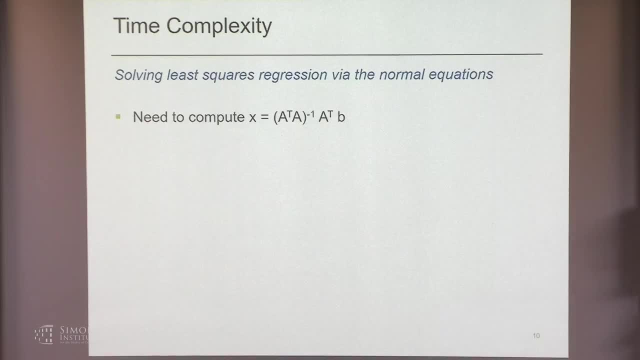 Okay, Any questions? just feel free to stop me. Okay, Yeah, so the time complexity, just to put it on a slide, is we need to compute this: x equals a transpose a, inverse a transpose b. It takes n d squared time, or n d to the 1.376 with fast matrix multiplication, and we want a much faster running time. 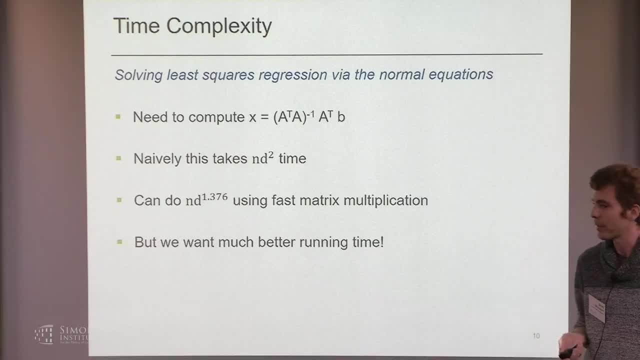 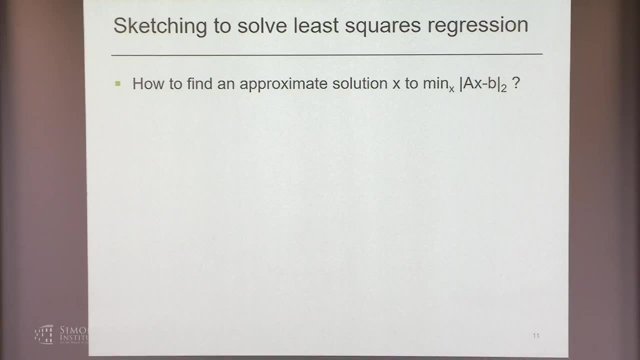 So this will lead us into the technique that I mentioned of sketching, or dimensionality reduction. Okay, so sketching dissolves these squares. Let's first relax the problem to allow for outputting an approximate solution. Now, what does that mean? 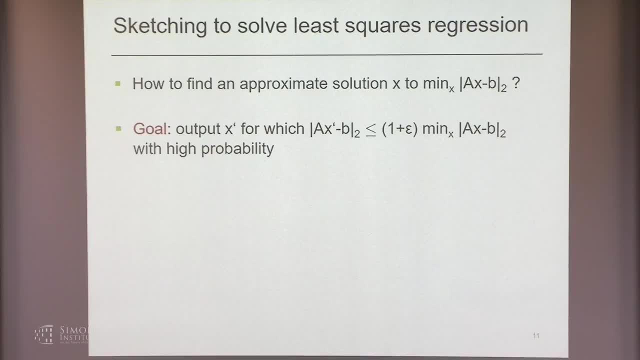 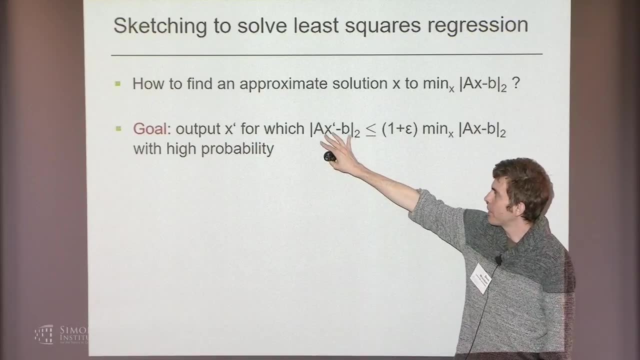 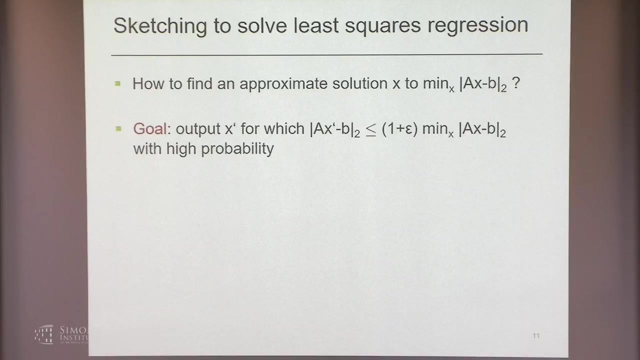 So we'll look at this from an objective function perspective. So instead of outputting the optimal vector x, let's output an x prime for which the- you know- Euclidean distance between a, x prime and b is at most 1 plus epsilon times the optimal cost that you would get, say, with the normal equations. 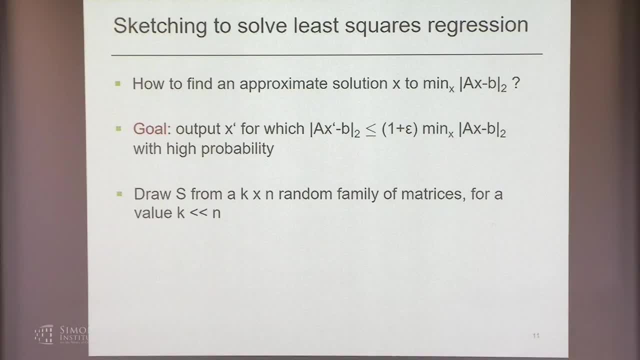 Okay, with high probability. So here's the sketch and solve paradigm if you haven't seen it before. So the idea is to choose a random matrix, S, from a certain family of random matrices. I'll get into different families. An important property about S: 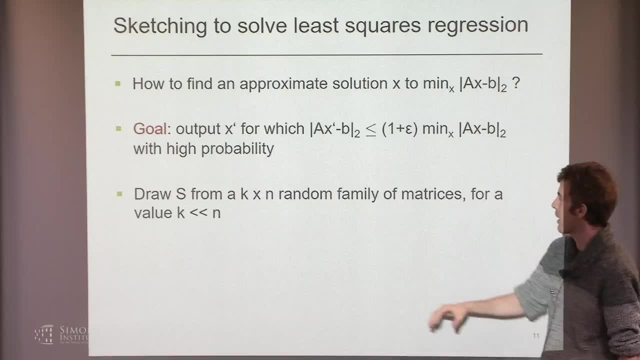 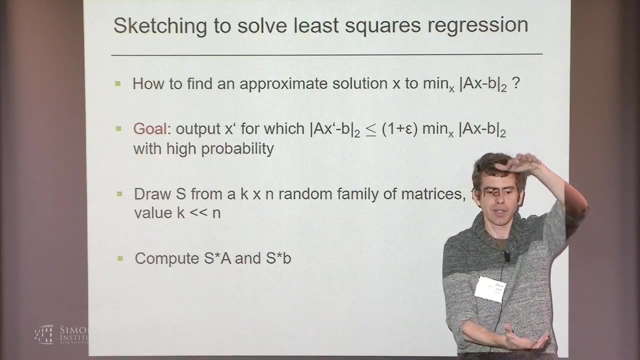 It's very wide and fat, Okay, so it has a very small number k of rows, typically much less than n, and, you know, often independent of n. Then the idea is to compute S times a, which will squash down this tall n by d matrix into a very small k by d matrix. 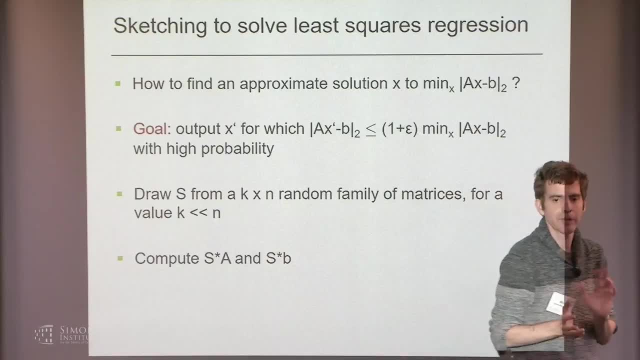 You can think of this k as being roughly order d or d over epsilon squared. I'll specify it more precisely in a moment. But roughly S times a is a small squarish looking matrix. S times b, instead of, you know, being n dimensional, is now only k dimensional. 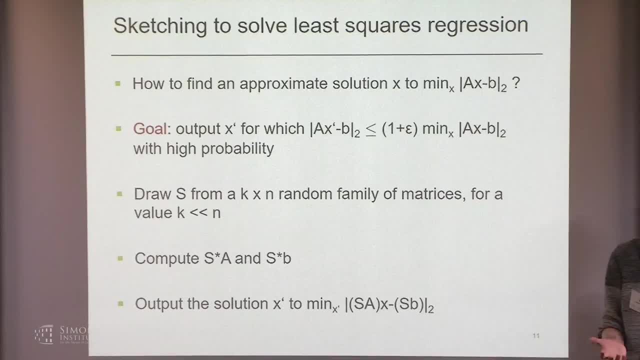 And now all you do is you have a black box reduction of the original least squares regression problem to a smaller instance of least squares regression where you've replaced a with S times a and b with S times b, And now you solve this small version of regression, which can now be solved efficiently, say with this closed form solution that I described, independent of n. 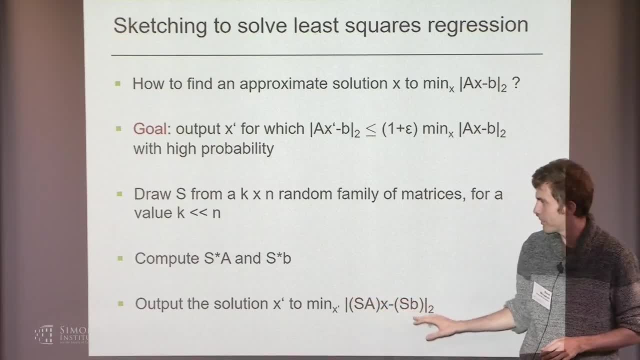 You know, if k does not depend on n, So you can solve this in time, which is like k times d squared. If you think of k as being roughly d, this is roughly d cubed time. Okay, So you know. the goal is to choose families of matrices S for which this sketch-and-solve paradigm works. 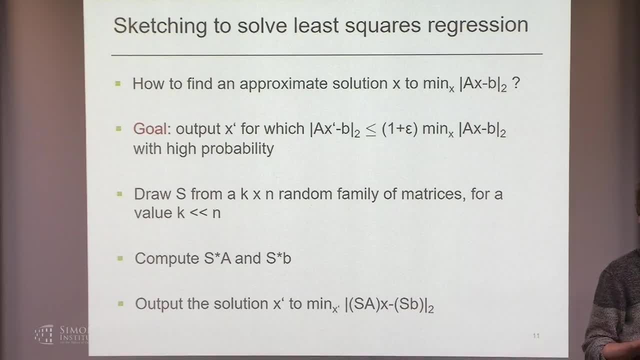 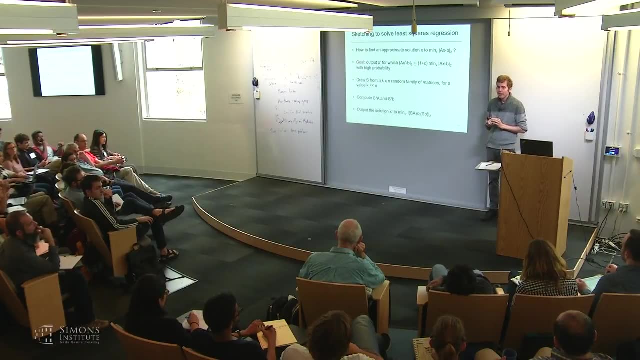 Any questions? Yeah, So I mean the resistance as an example, we could have just thrown away most of the observations, just picked a you know handful of those k of those and then solve the system. Is this going to be better? and what's next? 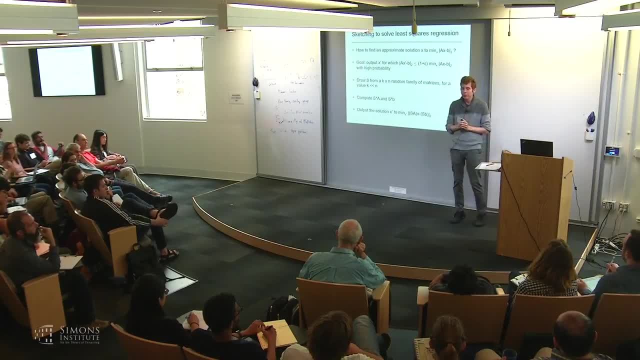 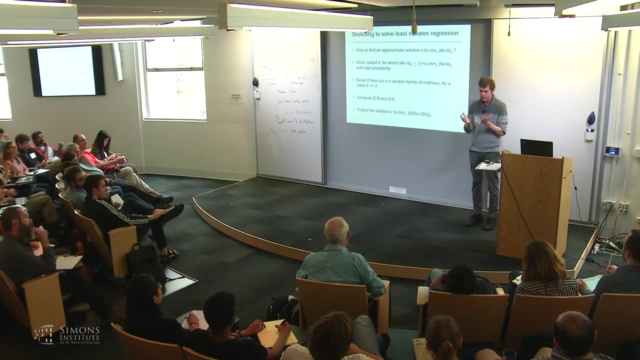 Yeah, so that's a good question. So I think the question is about random sampling. Can I uniformly sample a small set of or yeah, So uniform sampling will not give you the kind of relative error that we want. You can imagine, say you know in general for regression, you can imagine you know missing a very important example if I just uniformly sample. 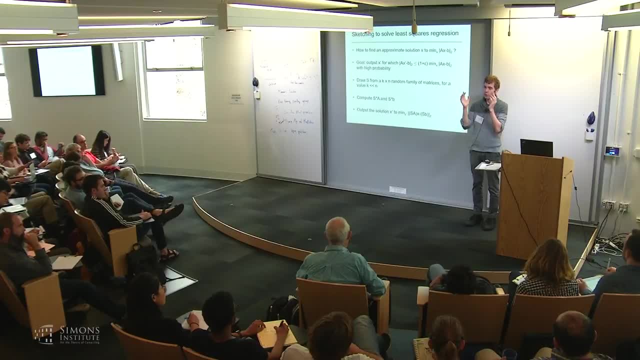 You could think about doing things like squared norm sampling, like Ravi was discussing, But that's also not going to give. That's not going to give you relative error. You know, you can imagine something where you have a matrix- say this is your n by 2 matrix- and imagine all of the rows have the same norm. 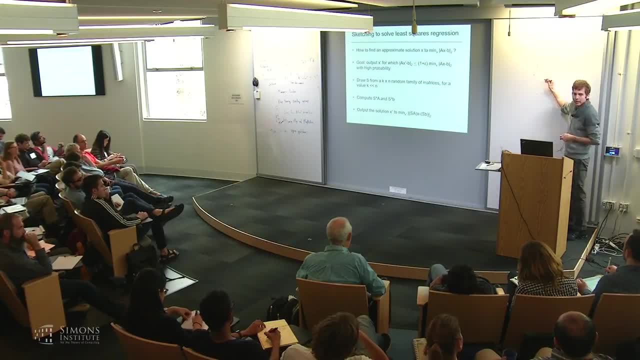 They all look the same, but for one of the rows you have a 1 minus 1, okay, And if you just sample by norms or sample uniformly, you'll never find this 1 minus 1.. But this 1 minus 1 might be very important for fitting your data. 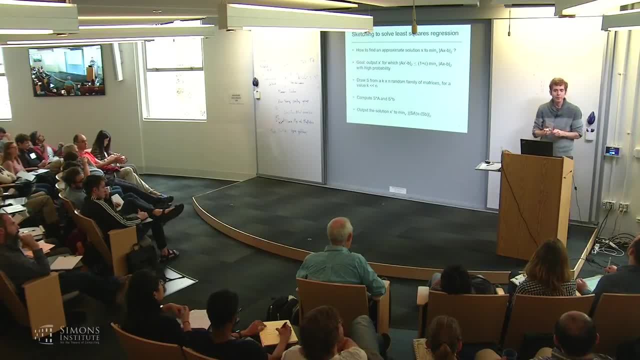 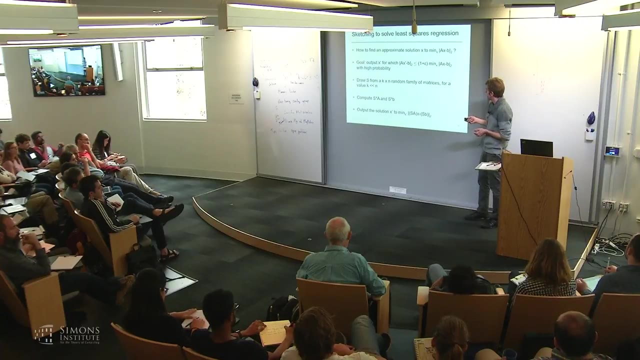 I mean, the sample will have rank 1 versus rank 2 in the two cases. Yeah, So yeah, Uniform sampling is not going to give us a relative error, and neither will squared norm sampling. Any other questions? Okay, Okay, so how to choose this matrix S? 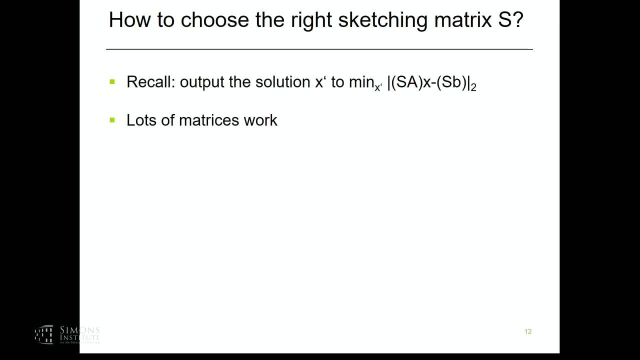 Yeah, so lots of families of random matrices work. The first that might come to mind is a matrix of IUD, normal random variables. So it turns out that if you choose S- the entries in S- And you choose each one to be IUD and you choose each one to be a standard Gaussian, there's a scalar factor I mean multiplied by a scalar. then this works. 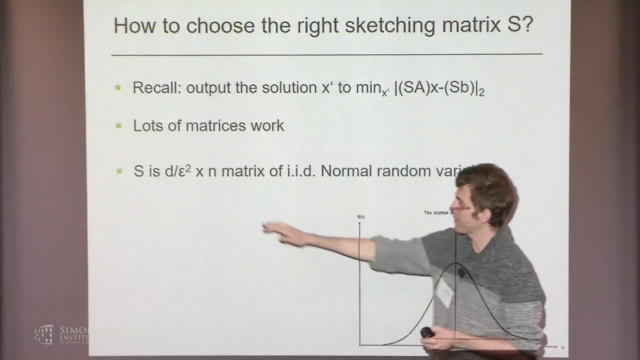 So the sketch and solve paradigm works. If I choose the number of rows in this matrix S to be order D over epsilon squared, okay, so I just replace A with SA, B with SB for this matrix S, I solve the small problem. I'll get a 1 plus epsilon. approximation relative error. 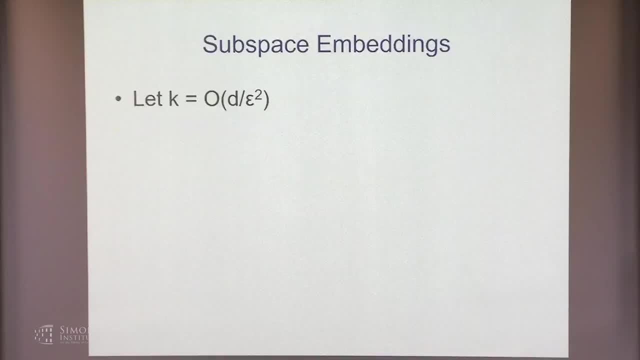 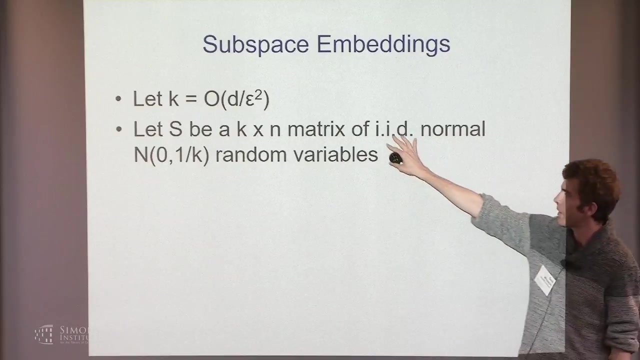 Okay, let me say a little bit why, and to do so let me introduce the notion of a subspace embedding. Okay, so let K be order D over epsilon squared and let S be this matrix of IUD: normal random variables. 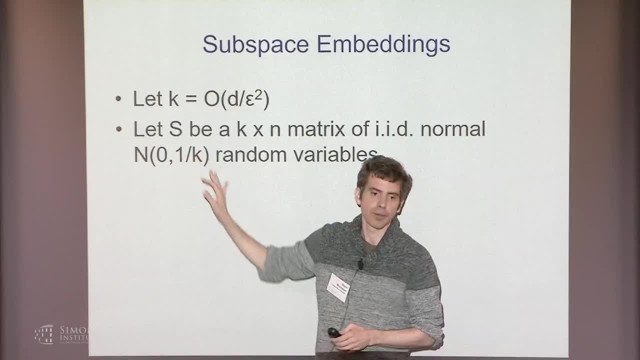 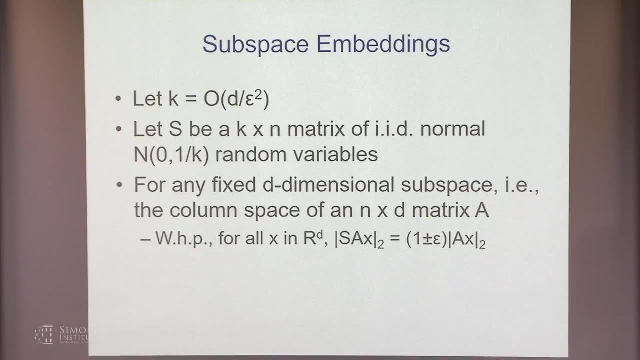 So, as I said, they're not standard normal, the variance is 1 over K. Okay, this is like this 1 over root K normalization factor that Ravi was mentioning, Okay, Okay, so what we like is the following subspace embedding property which is, for any fixed D-dimensional subspace, for example, the column span of an N by D matrix A. we have the following property for all vectors X and RD: 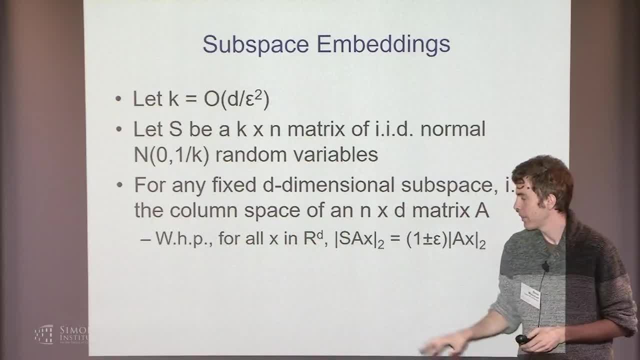 So, with high probability, simultaneously, for all vectors X. the Euclidean norm of SAX is about the same as the Euclidean norm of AX. okay, up to a 1 plus epsilon factor. Okay, this is the definition of a subspace embedding. 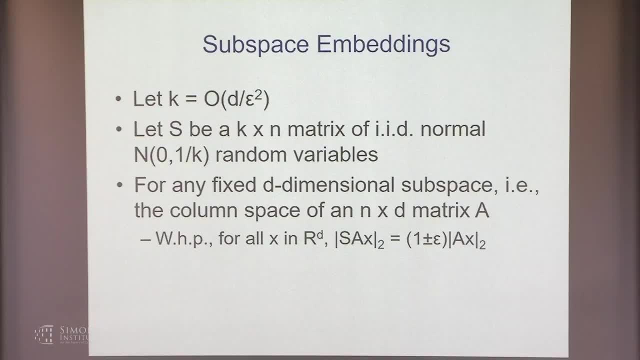 Okay, so notice the quantification that it's over all vectors simultaneously. Now, what is the proof that a Gaussian matrix, a matrix of IUD, normal random variables, with this number of rows D over epsilon squared, gives you a subspace embedding? 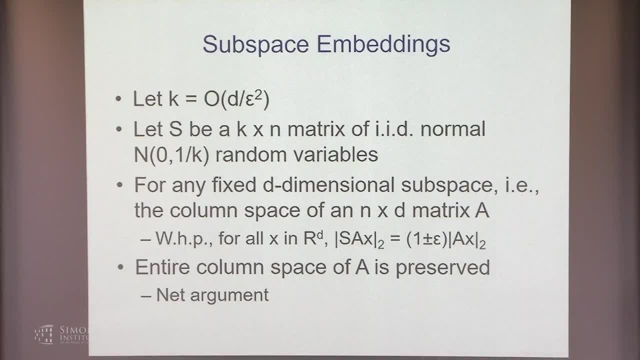 So this is via a net argument I'm going to. you know I don't have any slides on this, I'm just going to skip it, but the rough idea is to take your D-dimensional subspace, the column span of A. 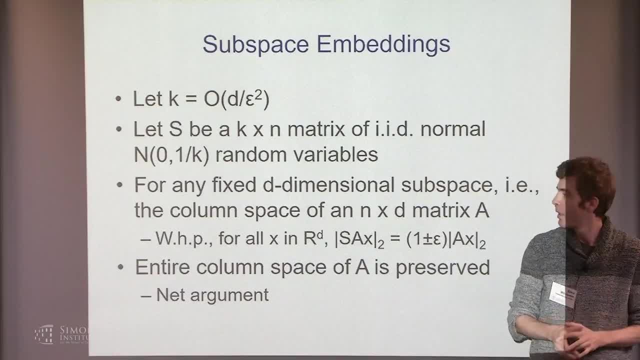 and to discretize it with a sufficiently fine net, So to find a finite set of points, roughly 2 to the D of these points. in the subspace you find this set of points. you show that this matrix S preserves the norm of all of those points. 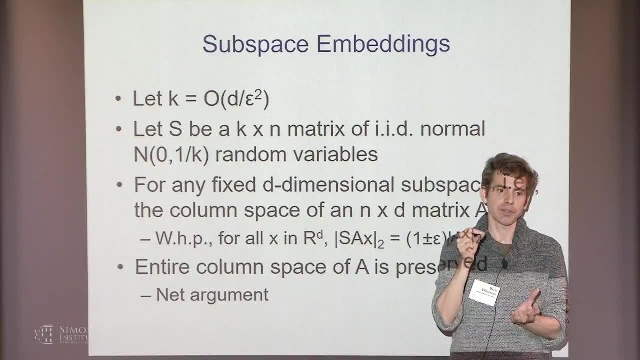 and since those points are sufficiently fine for any other point in your subspace, it's close enough to one of these points, and so therefore this holds for all vectors in your subspace. Okay, that's the rough idea. So it's like 1 by epsilon to the D. 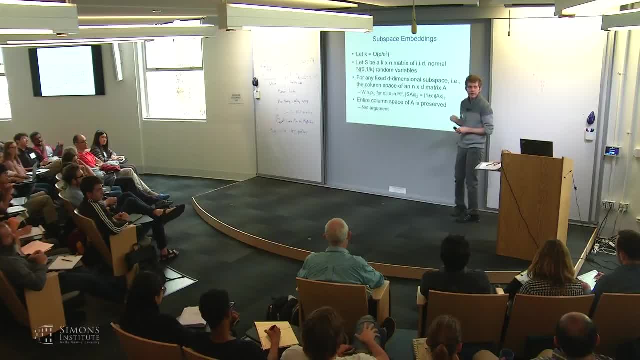 So the size of the net can actually be 2 to the D. you just need to choose the distance between the points to be constant and then you can sort of if you argue that for all the net points you preserve them up to 1 plus epsilon. 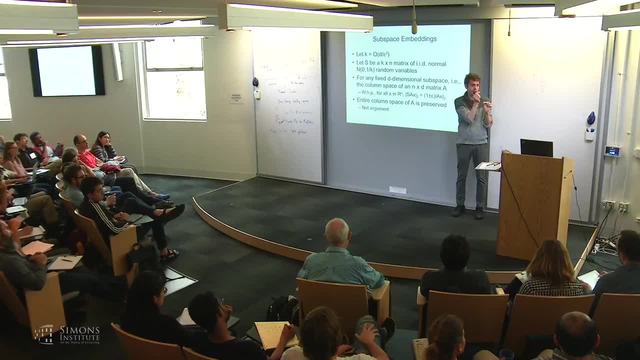 you can do like a chaining argument, like I preserve this: I take an arbitrary point, I write it as this point and then I plus a difference and then I look at the difference and I approximate the difference with a net point as well. 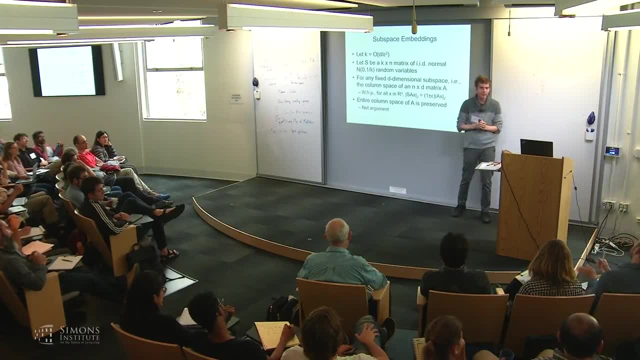 and then I look at the difference of that approximate with a net point and I can do this chaining kind of argument. So you save a log 1 over a Epsilon when you do that. yeah, Any other questions? Okay, 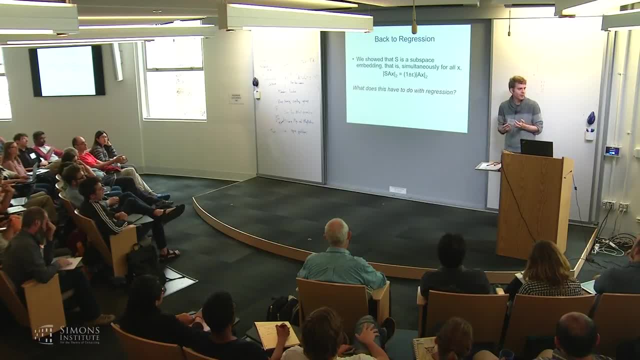 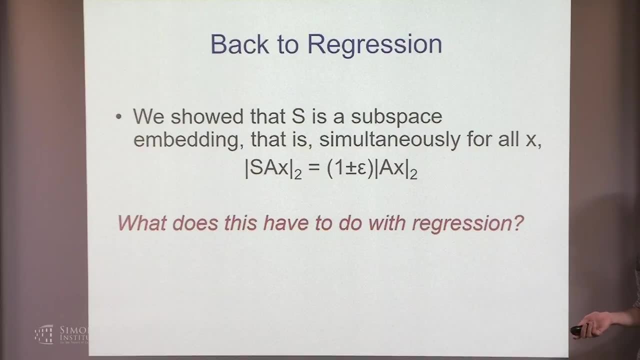 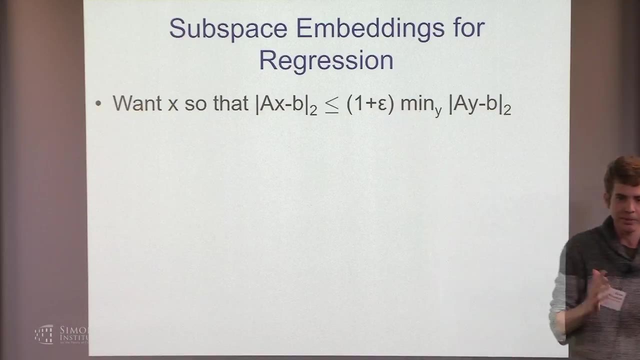 So what does this have to do with regression? What is the Why are we looking at subspace embeddings? Yeah, so this was the definition of subspace embedding and for the application to regression is the following: So recall for regression that we want this: 1 plus epsilon approximate solution in objective function values. 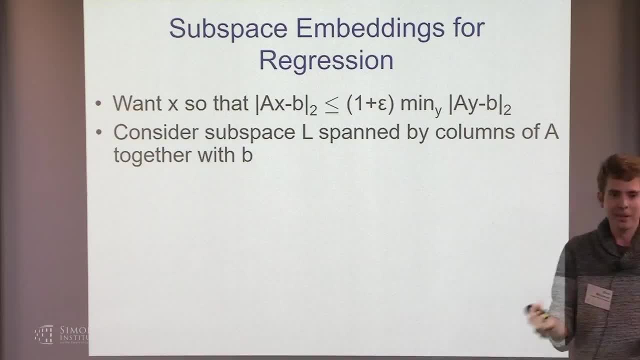 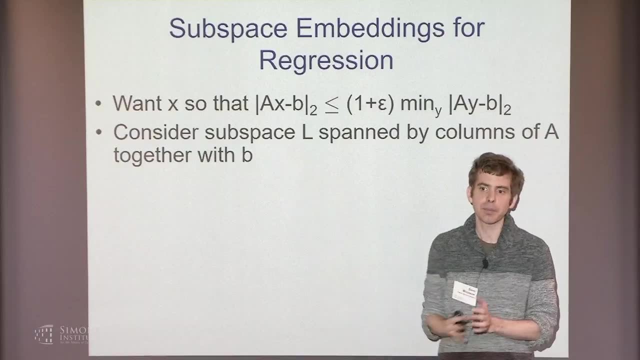 so let's just, it's a very, you know, direct application. consider the subspace spanned by the d columns of A together with your vector B: It's d plus 1 dimensional instead of d dimensional. This doesn't change any of the bounds asymptotically. 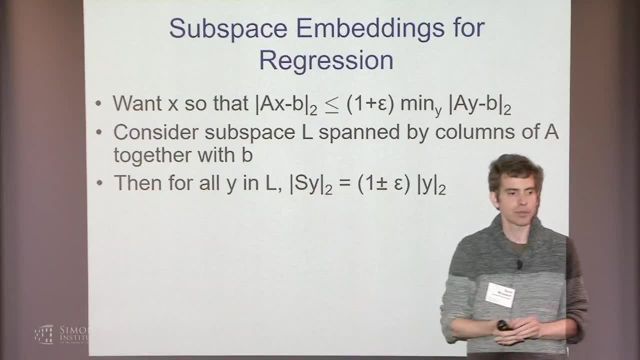 And then just apply this subspace embedding S to this d plus 1 dimensional space. so we'll have that, you know, for all vectors Y, its norm is preserved up to 1 plus or minus epsilon. So in particular, if we look at you know a candidate solution to the regression problem, it looks like AX minus B. 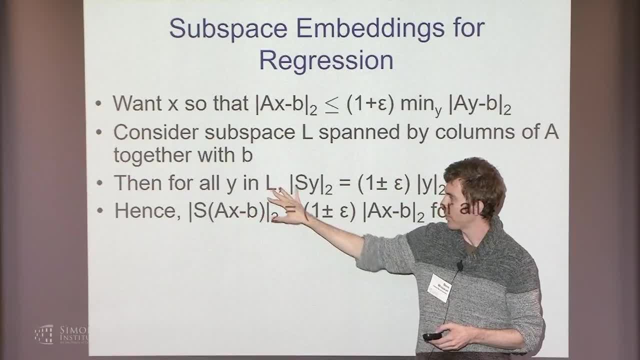 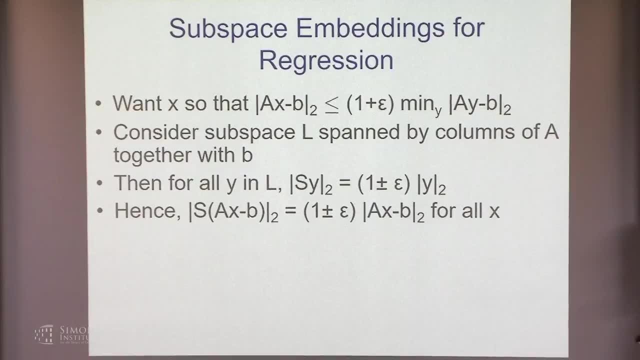 you know, it's inside of this d plus 1 dimensional space that I'm calling L, and its norm is preserved up to 1 plus epsilon. so all solutions have their value preserved up to 1 plus epsilon, which means that I can just solve. 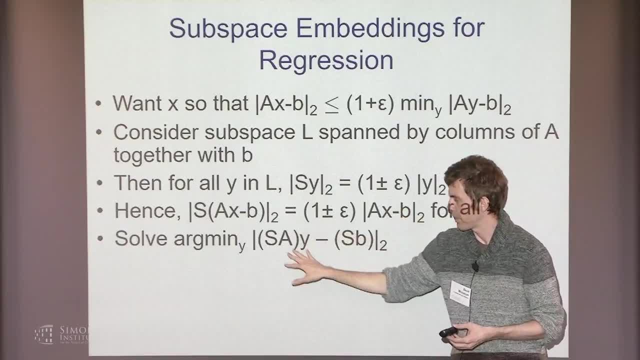 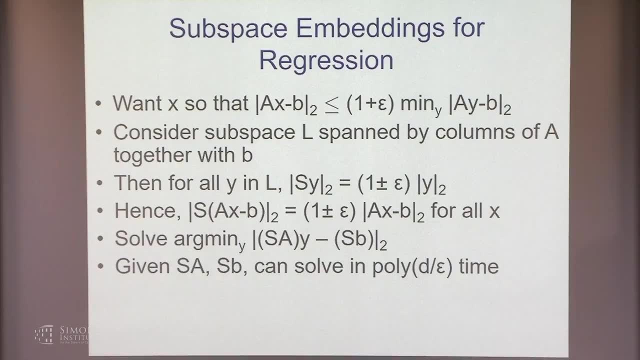 you know this smaller version of regression now, where I've replaced A with SA and B with SB. Yeah, and, as I said so for normal random variables, the number of rows of S, which I was calling K, is d over epsilon squared. 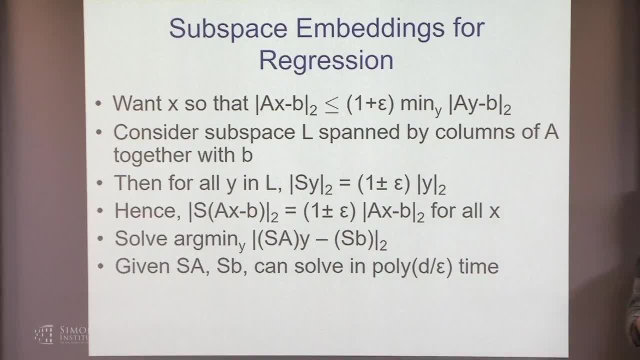 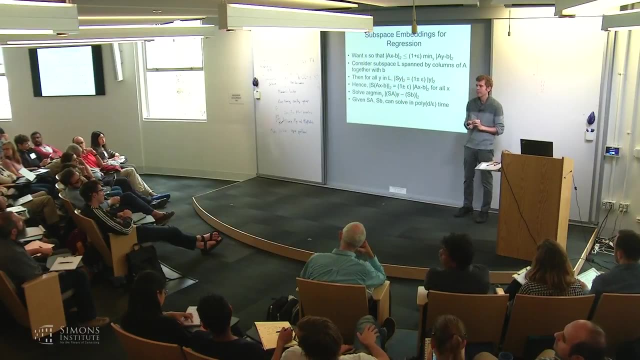 so the time to solve this small problem is roughly d cubed over epsilon squared, and you can accelerate that with fast matrix multiplication. Any other? any questions on this? Yeah, I'm not pretty clear about this high probability. you're saying so if for a specific S this holds, and then 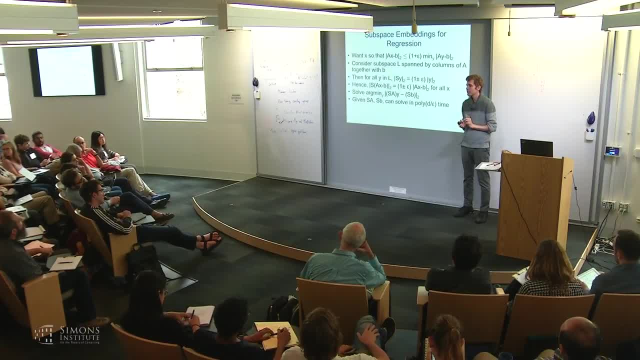 Specific A For all the samples this is holding. so What? how the union changed, you know, Yeah. so I wanted to just stress that we make no assumptions on A. You give me an A For any given A. 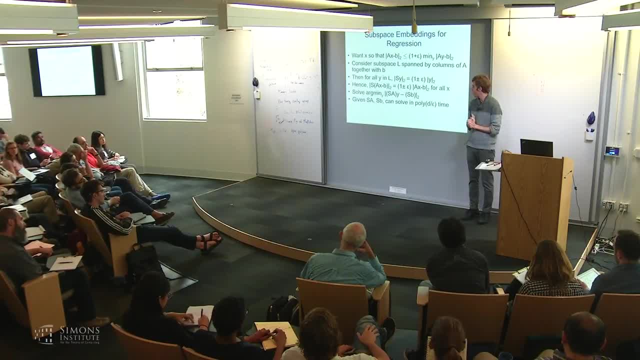 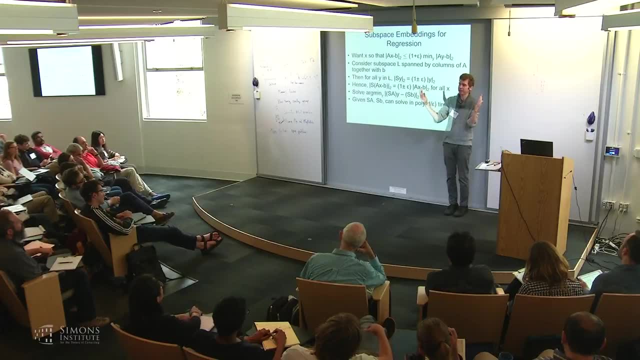 I sampled this random matrix S and I have the property that I preserve, you know, the entire subspace, the entire column span of A together with B, so I preserve the entire regression problem. with some good probability, What is the probability? for the case of Gaussians, This can be. 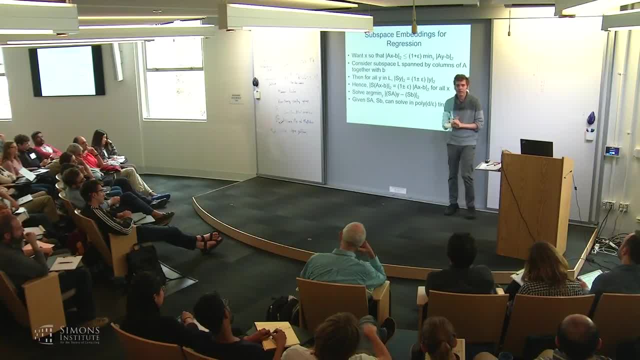 2 to the minus d. Yeah, Any other questions? So given S A and S B. so how do we go from A and B to S A and S B? usually? Okay, so this is so we can take a, we're given A and we're given B and we just sample random Gaussian matrix S. 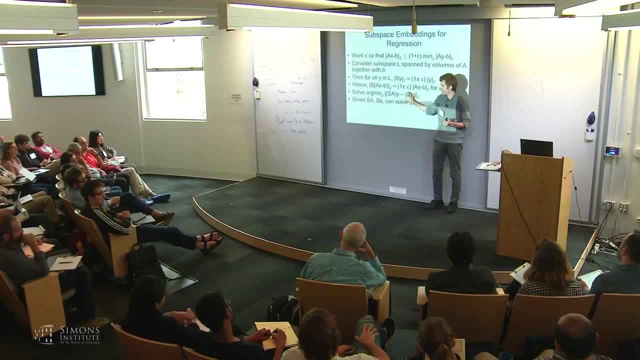 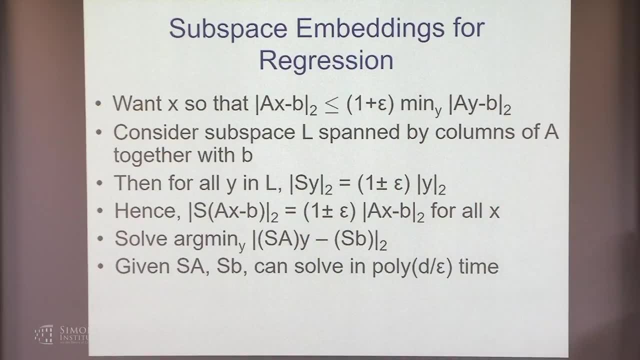 We compute S times A and S times B. We set up this regression problem, We solve it. This solution is d dimensional and we just plug it back in the original regression problem. Did we save a lot between the computation? That's a great question, Yeah. 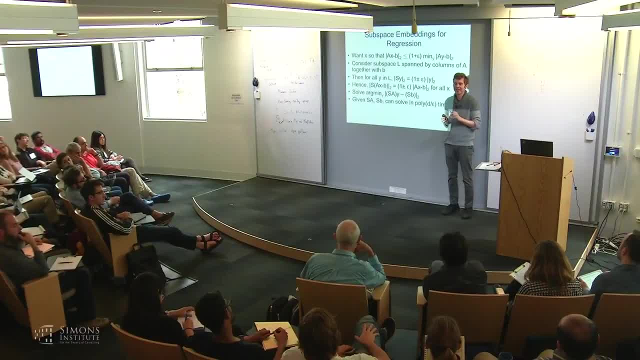 Yeah, so was that your question too? or I'm just wondering if M would be very large or a lot of observations, and S you say it's dense, it's a large. Yeah, perfect, great, You guys are both saying the same thing, yeah. 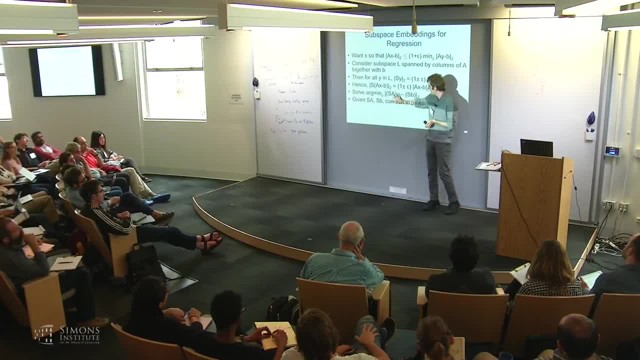 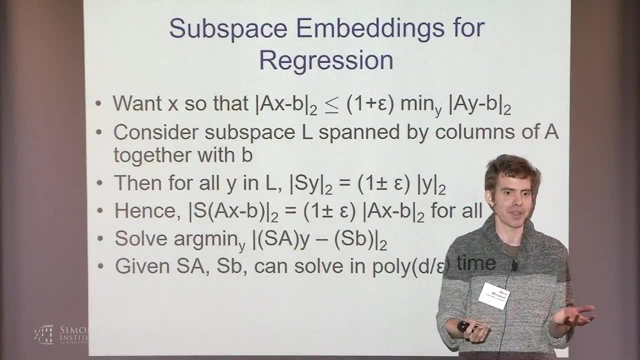 So this doesn't give us a savings at all. right, Like I mean computing S times A. you know S has even more rows than D. We already said, you know we could multiply by A, transpose and solve it exactly in N D squared time. 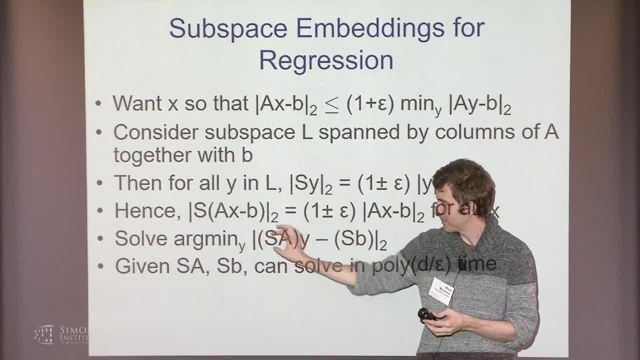 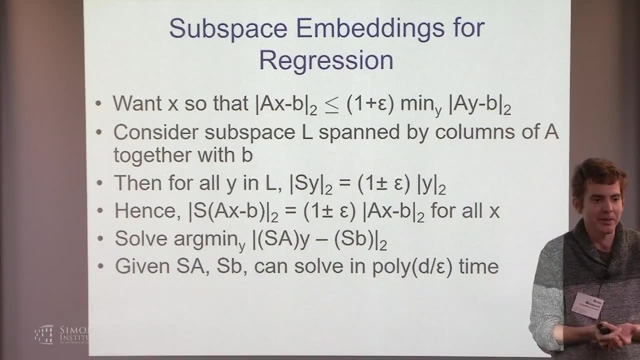 What are we doing now? You know S has D over epsilon squared rows. It's dense Computing. this product is taking even longer than N D squared time and we're just getting an approximate solution and with some probability right. So we haven't really gained anything. 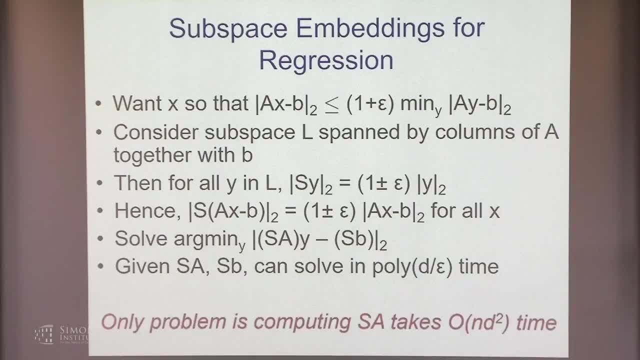 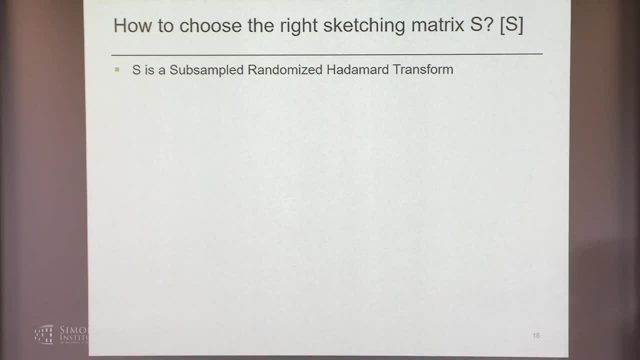 but it's, you know, sort of a proof of concept, And yeah, so, yeah, exactly, this takes too long. Now, the first improvement to this was given by Thomas Sarlos, who observed that you can choose S instead of being from an, you know, matrix. 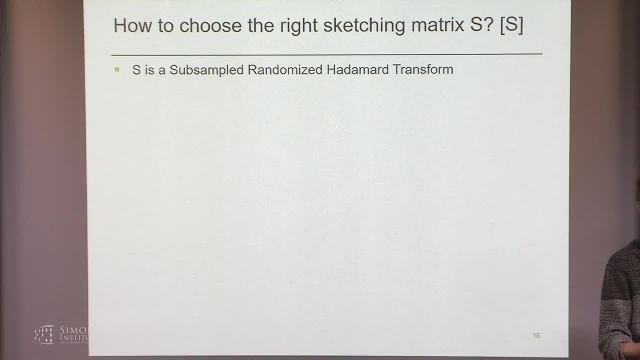 with IAD normal random variables. you can choose it from a much more structured random family of matrices called subsampled randomized Hadamard transforms. So what do these typically look like? They typically can be factored into a product of three matrices: P, H and D. right? 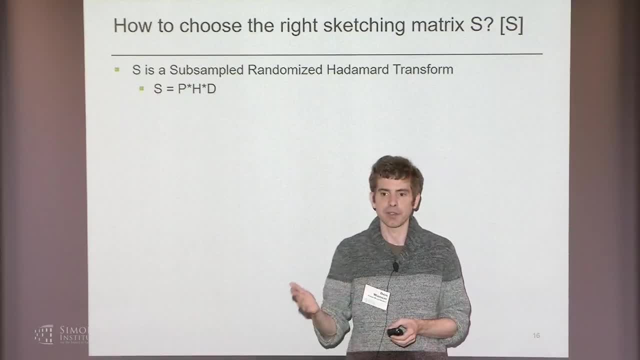 And the point about these factors is that they can all be applied very quickly to a vector. okay, So I just have one slide on this. so Ken tomorrow will elaborate more on this and give a proof, but let me just give you some intuition. 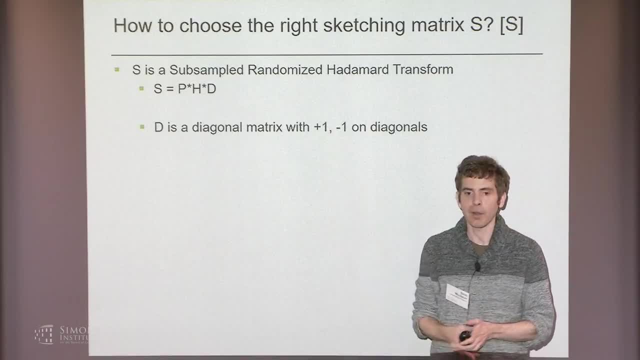 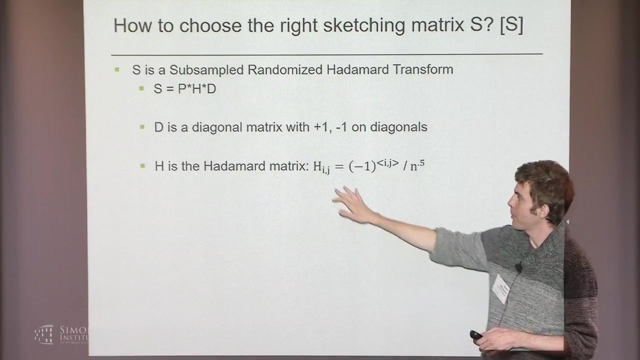 So what are these factors? So D is just a random diagonal matrix, so the entries on the diagonal are chosen independently. Each entry with probably a half is chosen to be one and probably a half is chosen to be minus one. H is just the fixed matrix, the Hadamard matrix. 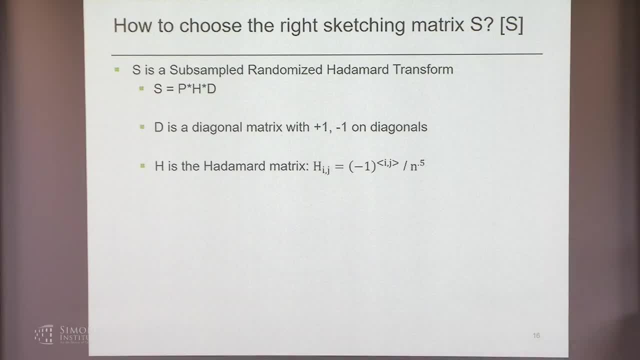 so it's an orthonormal matrix where the entries are all bounded. The nice thing about H is it's a dense matrix, but even though it's dense, there's a very fast matrix vector product associated with it, okay, Which you can do recursively. 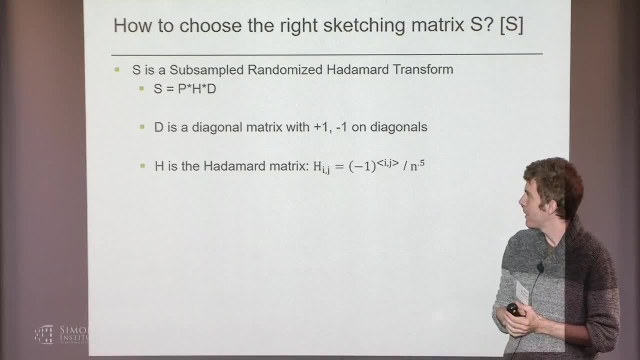 It's similar to like fast Fourier transform The entries of H. they're not so important, but you know they're all plus or minus one over root n And P. well, P is just a sampling matrix, uniform sampling. 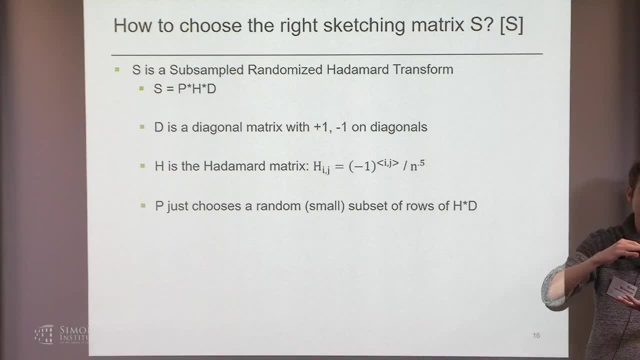 So when I apply it to a vector, I just uniformly sample a subset of coordinates. In this context it's sampling a small subset of rows of H times D. okay, So D and H are both square matrices, You know. they preserve the length. 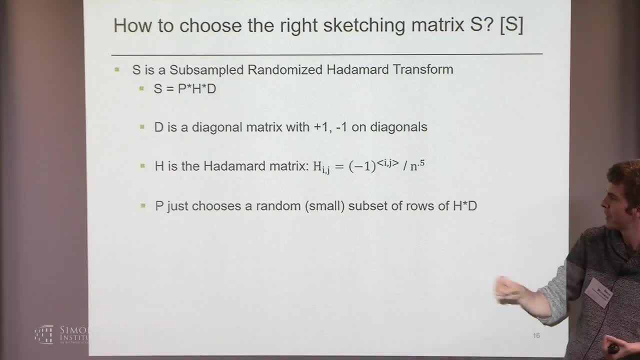 of an n-dimensional I mean. so I have an n-dimensional vector. it's still n-dimensional and P is going to. the number of rows of P tells me how many rows I have in my sketch And the number of rows in P can be chosen to again. 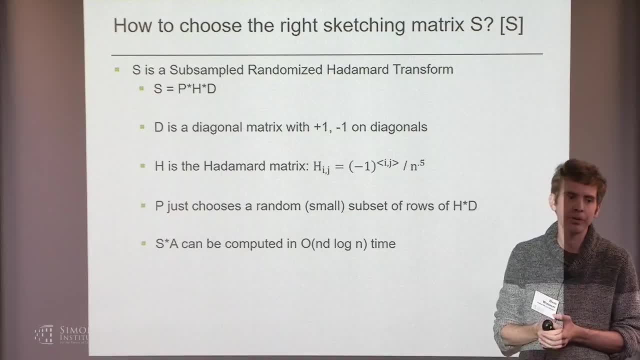 be about D over epsilon, squared, like in the case for Gaussians. but there are additional log factors. Okay, so, importantly, S times A can be computed in nd log n time using this fast Hadamard transform. Okay, the other things. D is order n time. 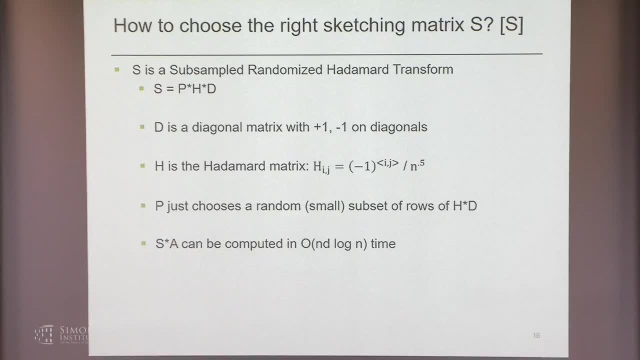 P is, you know, even sublinear time. And you can show that this works, that if P has roughly D over epsilon squared rows, you get a subspace embedding and the same kind of argument goes through. And now, using the connection to regression that I described, 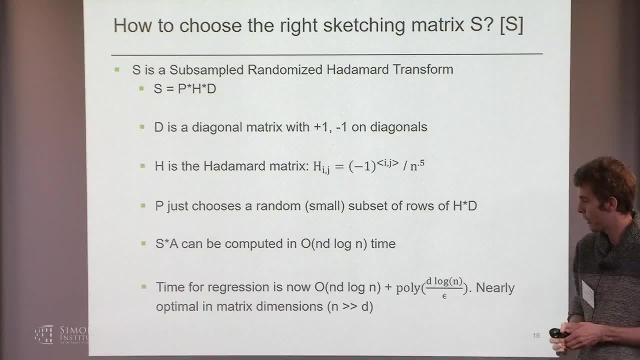 you get a much faster algorithm. Instead of nd squared, you get, you know, roughly nd log n. Yeah, this can be improved a bit using these techniques like nd log d or so, but it's you know, roughly n times D. 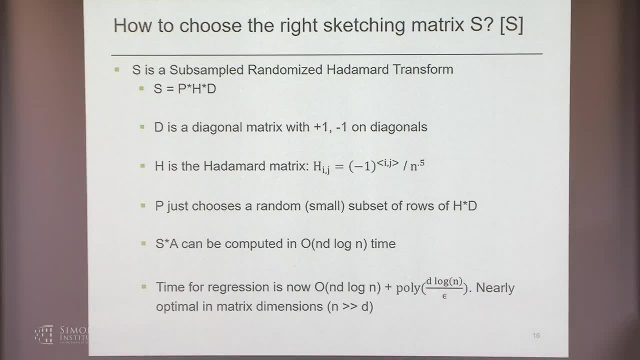 plus, you know, polynomial in the small parameters like D log, n over epsilon. So this is nearly optimal in the matrix dimensions. You know it takes you sort of. you have an n by d matrix. If it's dense you need to spend nd time otherwise you'll miss. 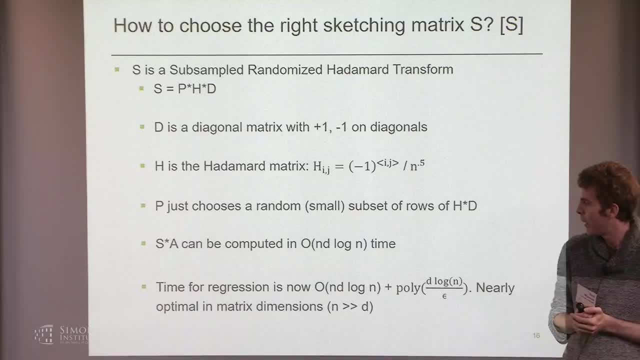 say some, a very large entry, for example. But you know, in many cases your matrix yeah. so the proof: see Ken's talk. In many cases your matrix A is actually a sparse matrix. Okay, So you might want, instead of spending nd time, 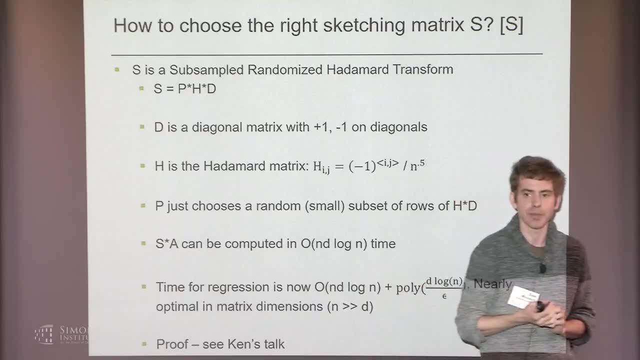 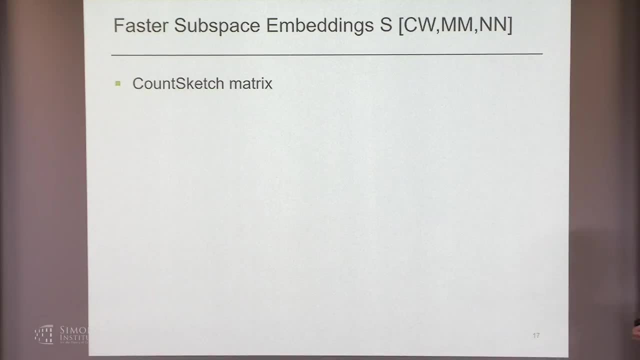 to spend time proportional to the number of non-zeros of your input. matrix A: Okay, So, okay. so this leads to yet another random family of sketching matrices. These are called count-sketch matrices. These matrices are called count-sketch- yeah. 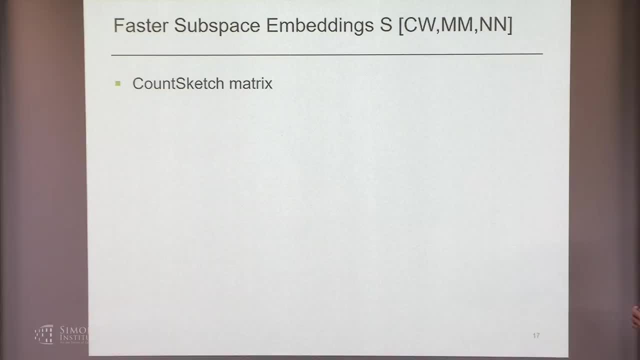 this is originally due to Moses Chen and Frock-Colton, So these were. these originated in sort of a data stream context. This is why they're called count-sketch, I think, because kind of finding frequent items. Correct me if I'm wrong. 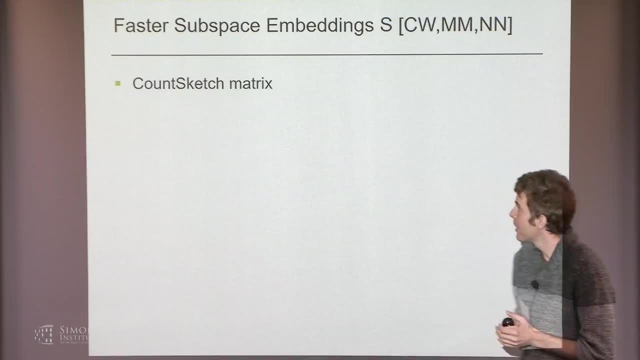 And it's also been used for things like feature hashing. So what are these? So these are again wide-fat matrices with more rows now. So instead of just d over epsilon squared rows, I have roughly d squared over epsilon squared rows. 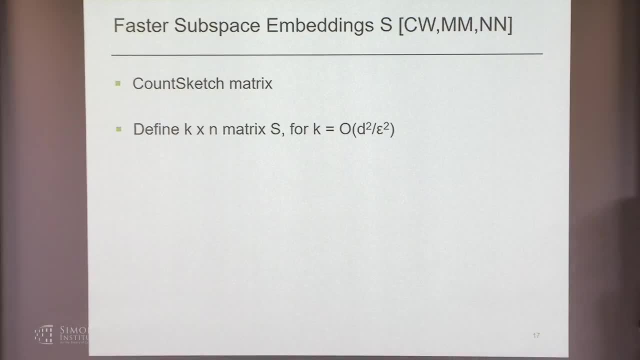 Okay, Still independent of this large dimension. n. The nice thing about these matrices S- if you haven't seen them- is they're extremely sparse, Okay. So what they look like is they just have a single non-zero entry per column, Okay. 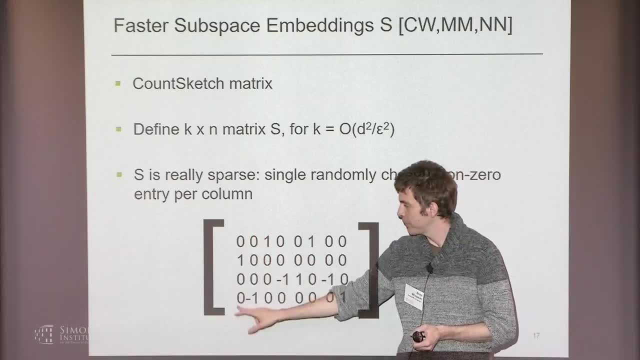 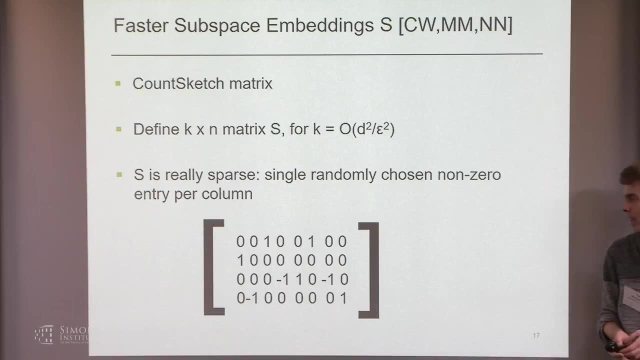 So how do I generate a matrix S? For each column I choose uniformly a position. On that position I put a 1 with probability 1 half and a minus 1 with probability 1 half. I can do that independently for each of the columns. 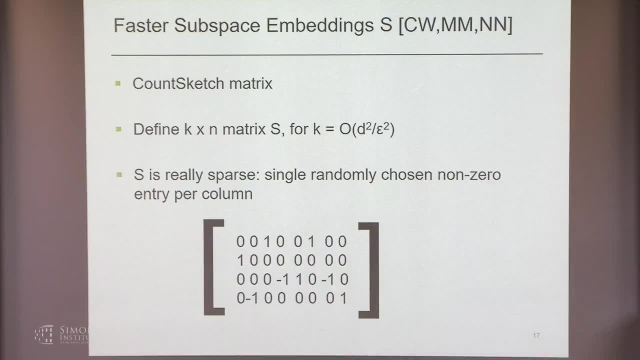 but you can actually show that bounded independence suffices for this as well. They don't have to be fully independent. So the nice thing here is that S times A can be computed in n and z of A time where n and z is the number of non-zero entries of A. 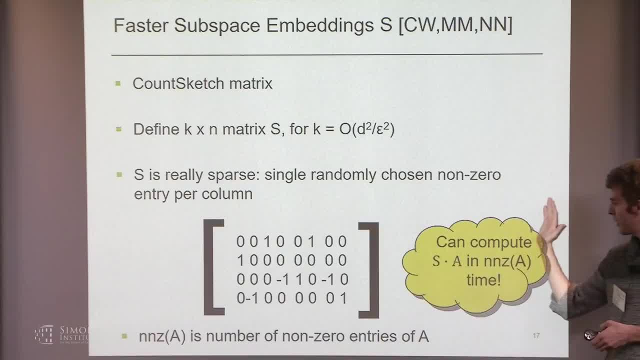 Okay, So why is that? I mean for each column of A, for each non-zero entry. I look up the corresponding column in S and there's only a single non-zero entry there. So I can update my matrix product in constant time per column. 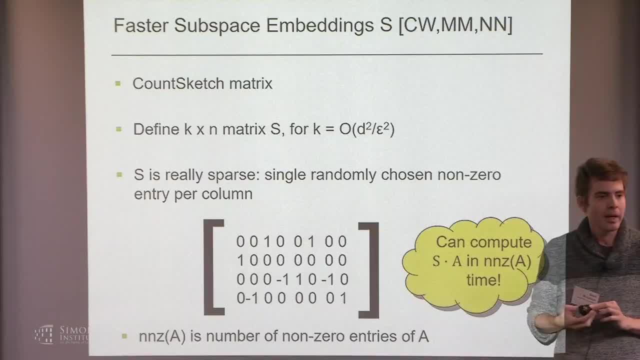 Okay, And the nice thing is that this actually works with these parameters: d squared over, epsilon squared being your number of rows, And yeah. so using the connection to regression, you get an overall algorithm which runs in time. number of non-zero entries of A. 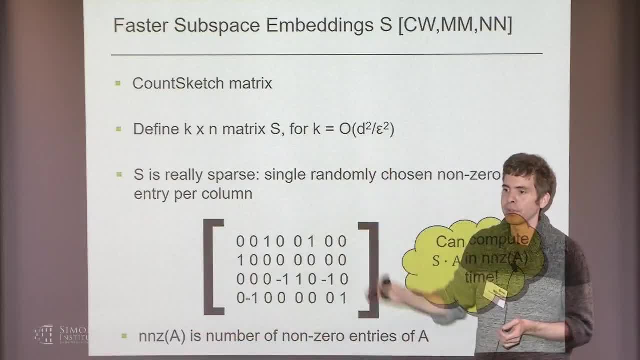 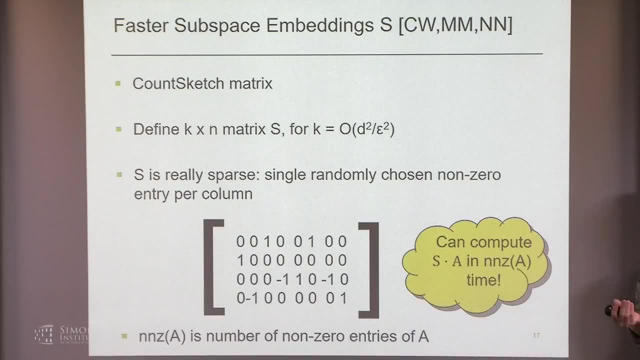 plus a polynomial in d over epsilon. So I'm going to focus on this one and give you a proof of why this one works. The other two families of matrices I didn't give prior to this, but I'm going to give you a proof of why this one works. 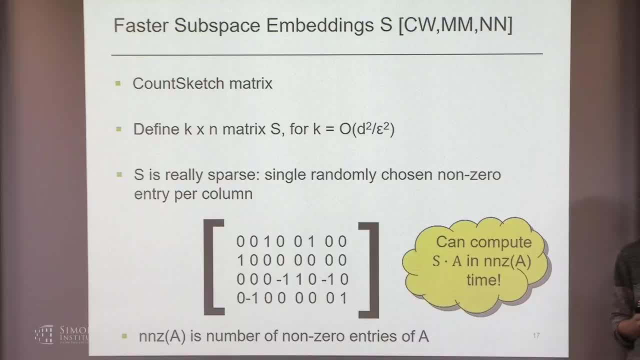 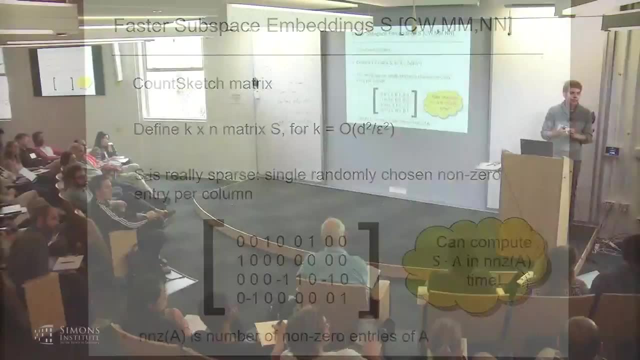 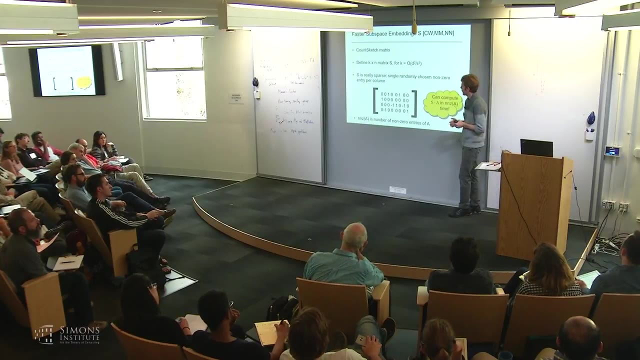 Any questions so far? Yeah, So you said that this works with a high probability and I would assume that would be a form 1 minus theta, right, Yeah, So for count sketch the probability is not very high. Like what we'll see is there'll be a linear dependence on delta here. 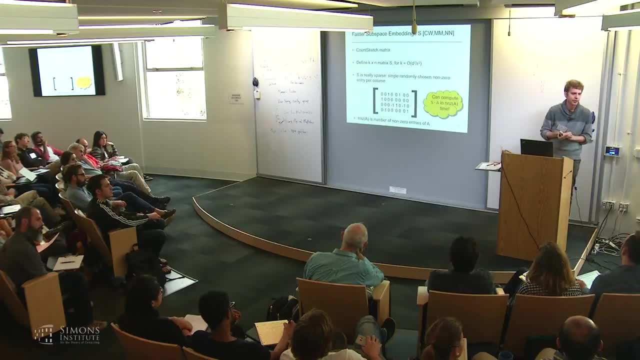 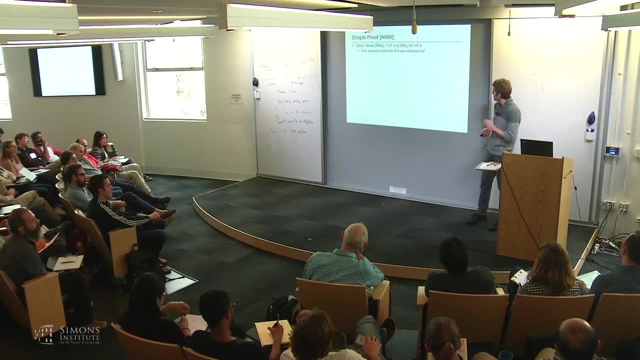 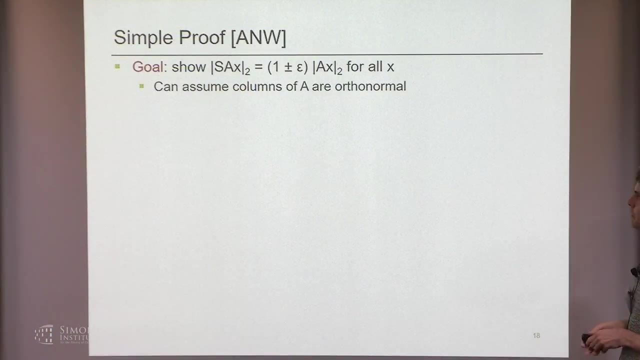 Yeah, Unlike for Gaussians, where we had sort of exponential failure probability. Yeah, Any other questions? Okay, Okay, so here's a simple proof. So yeah, due to In a paper of Avron Nguyen and I. 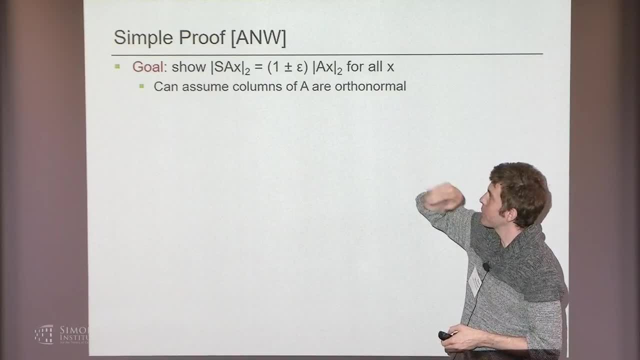 So what we had is What we want to do is show the following: We'd like to show that the norm of S AX is 1 plus or minus epsilon, the norm of AX for all X. We just have this subspace embedding property. we'd like to show: 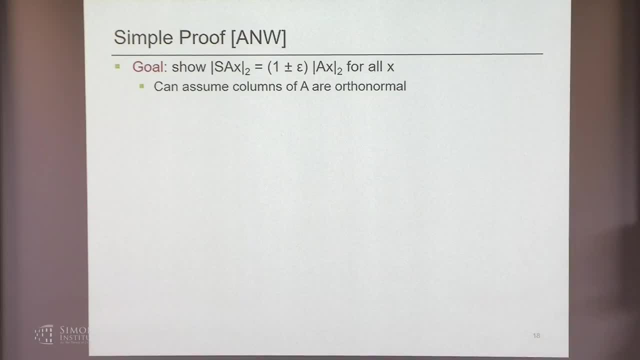 Um, The first observation is: you can assume that the columns of A are orthonormal. Now, why is that? Well, you're going to be proving this statement for all vectors, X, right? So as I range over all X, you know I'm ranging over all AX. 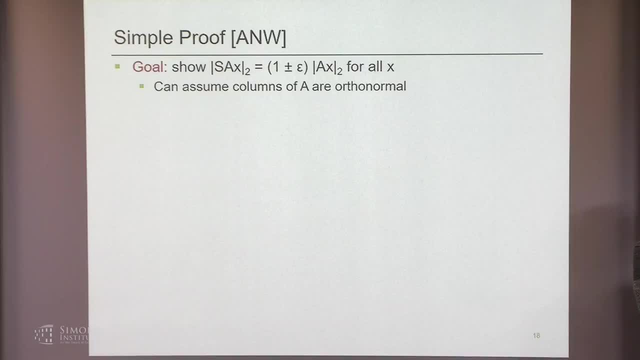 I'm ranging over all vectors in my column space. It doesn't really matter which basis I range over, So I might as well range over a basis where A has orthonormal columns. Okay, This is the first observation. Um, The second observation is that this is a linear map. 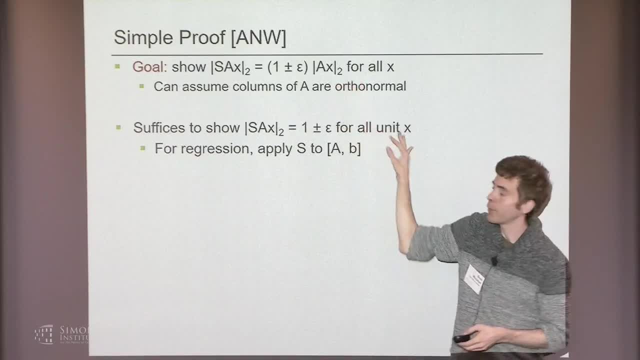 Right. So I might as well just prove this statement for unit vectors X. If I prove it for all unit vectors X, and therefore AX is also a unit vector. since A has orthonormal columns, then it holds for all X by linearity. 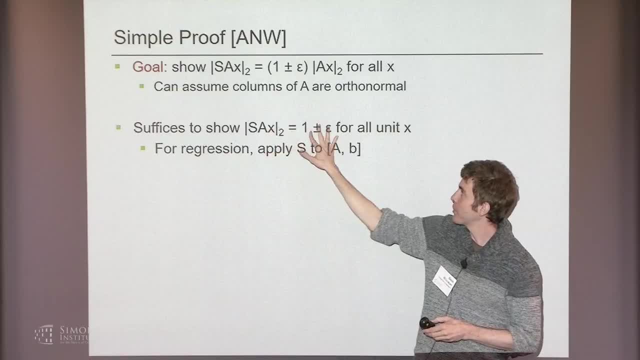 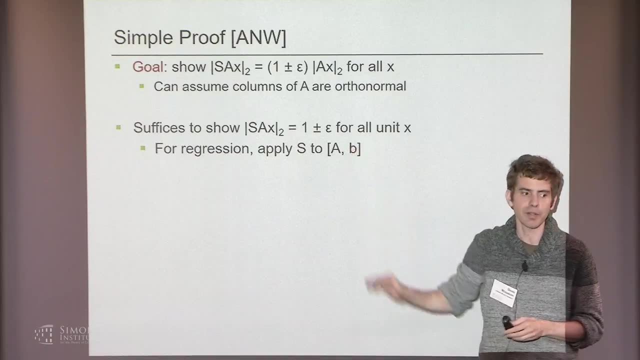 So really I just need to prove that the norm of S AX is 1 plus or minus epsilon for all unit X, And again, after we've shown a subspace embedding guarantee, then we immediately get the application to regression, just by applying it to A comma B. 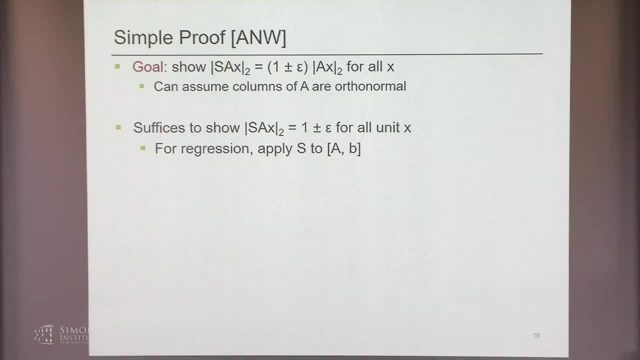 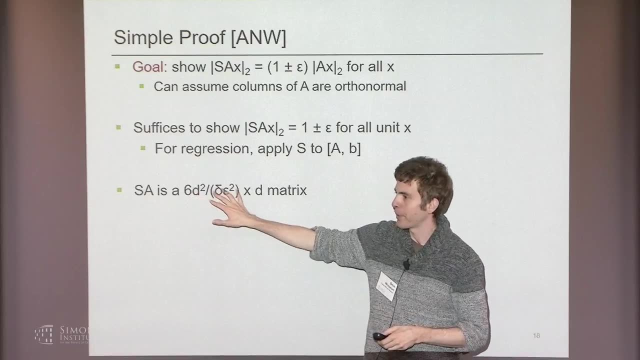 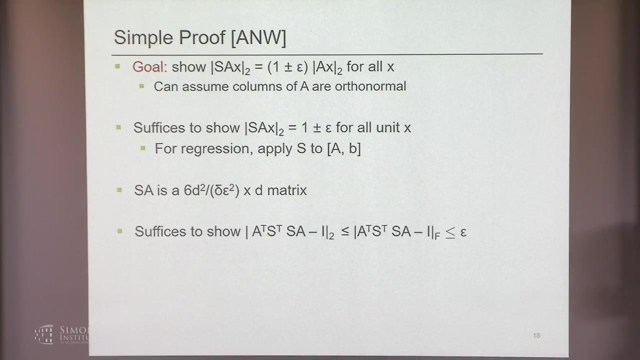 Okay, Okay. so here is the argument: Um. So let me instantiate the number of rows of S to be 6D squared over delta epsilon squared. As I said, it's roughly D squared over epsilon squared. Um, Okay, so here is the sort of a key observation. 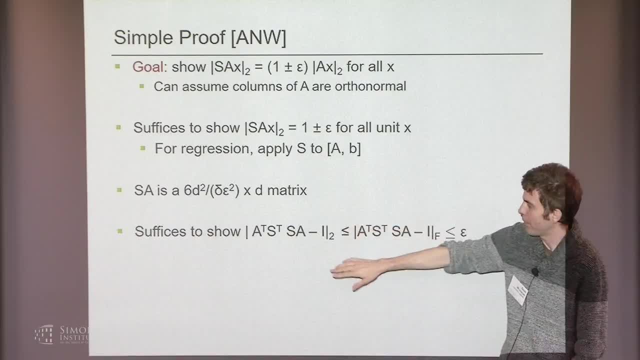 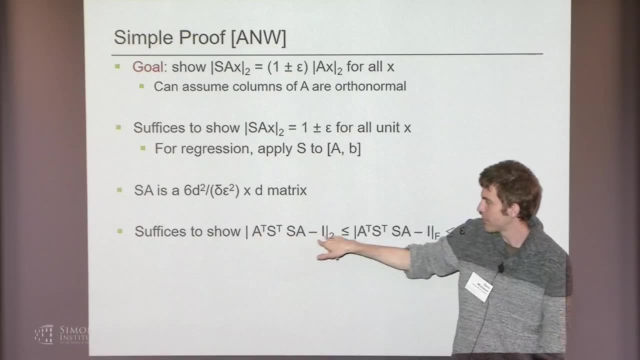 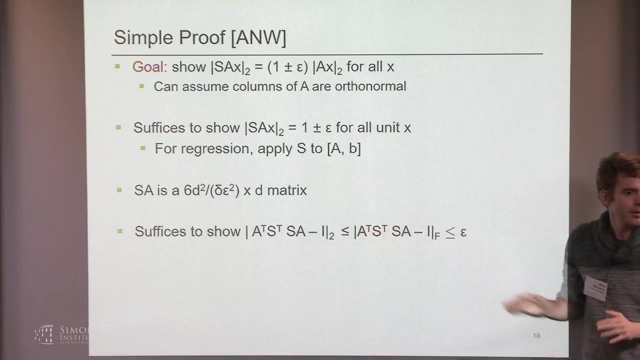 Um, Let's look at the operator norm of A transpose S, transpose S, A minus the identity. Okay, This is a D by D matrix, This is a D by D identity. And suppose, Just ignore this middle norm. Suppose we show that this operator norm is, at most, epsilon. 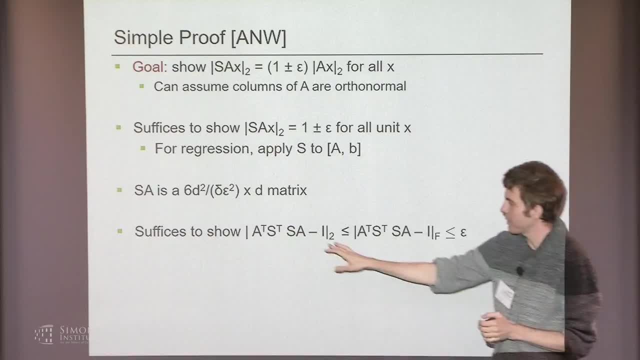 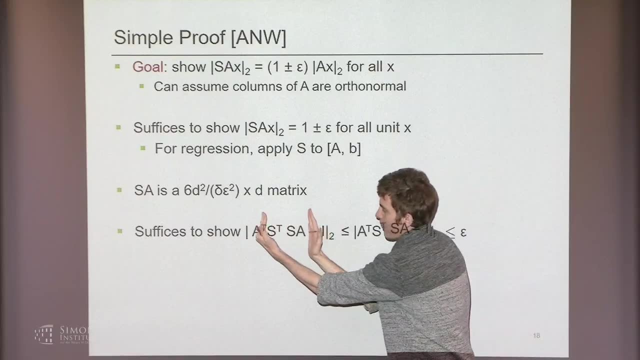 Then we're all set right. Why is that? Because then if I apply S A to any vector X and I apply X transpose X- any unit vector, then this will become the norm of S- AX squared X transpose X. that's just going to become 1.. 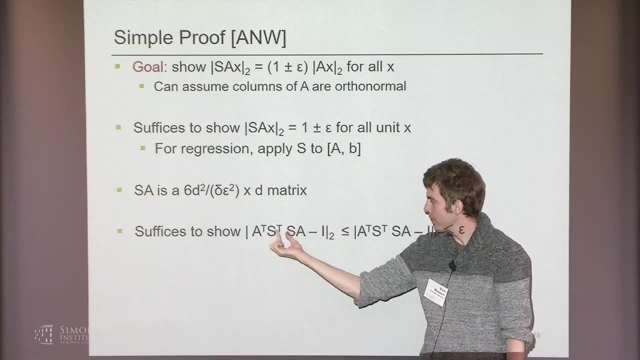 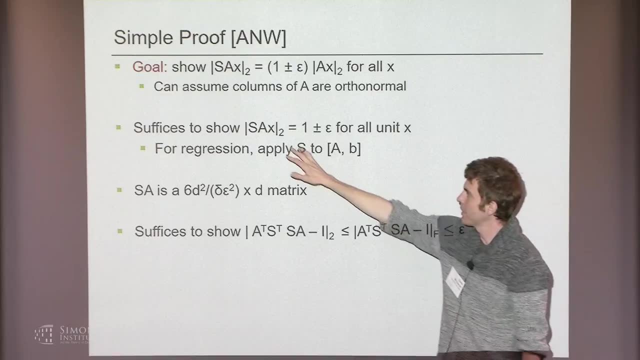 It's a unit vector, And so I'm saying the norm of S? AX squared minus 1 is at most epsilon. That's the same thing as saying that, you know, for all vectors X, the norm of S? AX is 1 plus or minus epsilon. 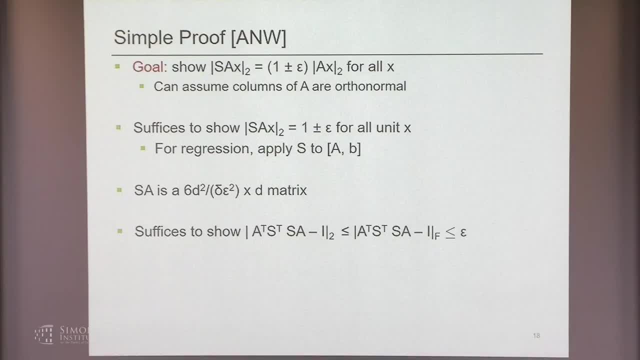 Okay, so this operator norm captures, you know, sort of all vectors. Is that clear? Okay So, um, it's hard to bound an operator norm directly, So instead of bounding the operator norm, I'm going to upper bound the operator norm. 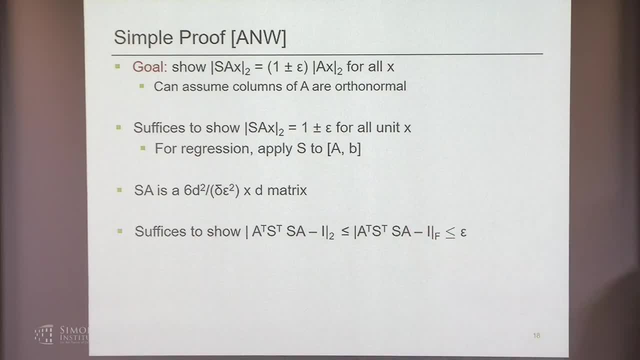 by the Frobenius norm. And I said I'm just going to show that the Frobenius norm of A transpose S, transpose S, A minus the identity is at most epsilon. Okay, remember Frobenius norm, just sum of squares of entries to the 1 half. 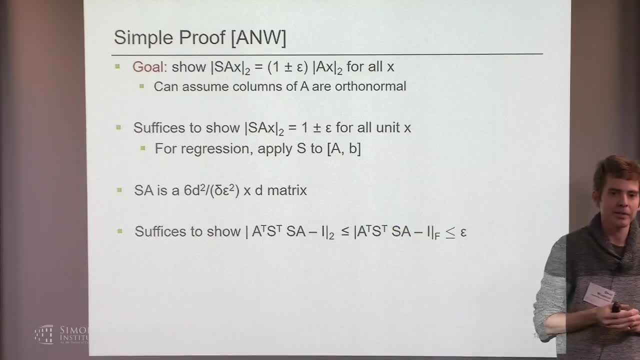 And Frobenius norm is something that I understand much better. Right, just sum of squares of entries. So you know we have a form for S. We can imagine just trying to compute this directly, And that's what we do. 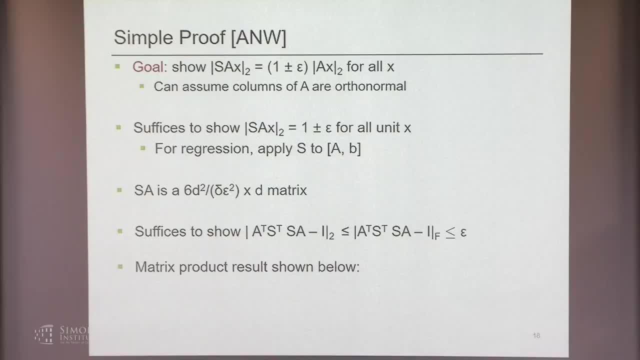 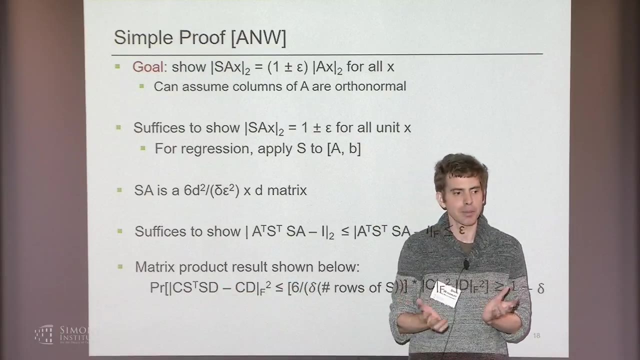 Um, okay, So what we'll show below is that the matrix, the following matrix product result, which is that you give me any two fixed matrices, C and D. if I sample one of these random count sketch matrices S, then I can approximate the matrix product C times D. 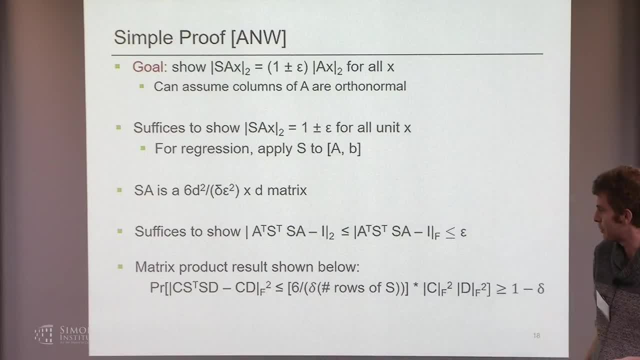 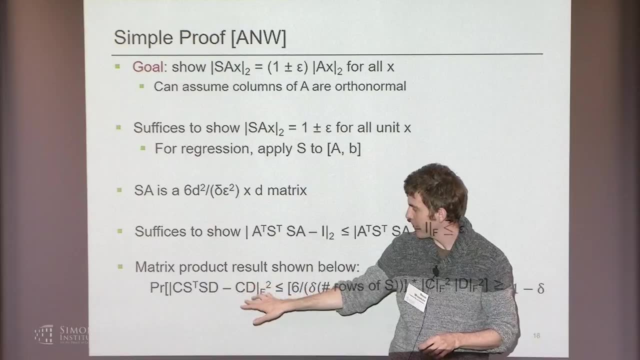 So suppose you know C? the number of columns of C is the same as the number of rows of D, so that these can be multiplied. Instead of computing C times D, I'm going to compute C times S. transpose times S times D. 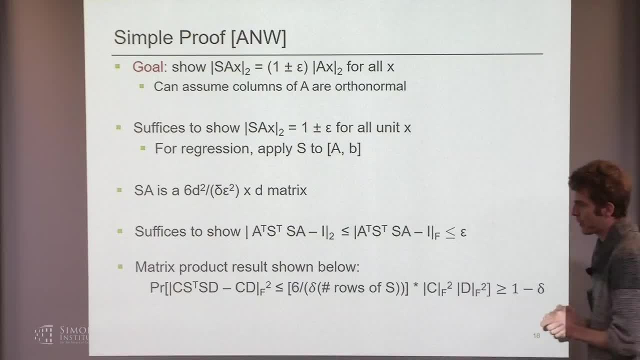 And what I'd like is this matrix product result, which is that the norm of the difference of my approximation and the actual product, or the squared norm, is at most, um, you know something, that's you know, roughly one over the number of rows of my sketch S. 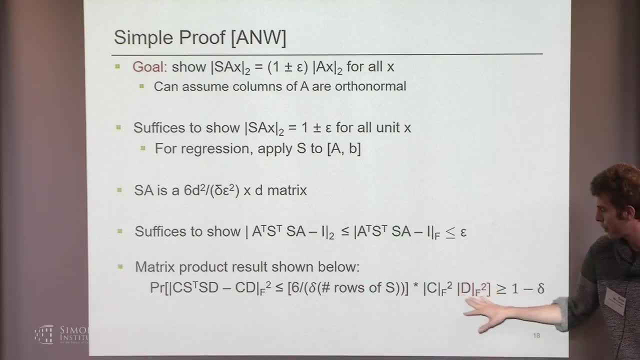 times the squared Frobenius norm of C, times the squared Frobenius norm of D, with some good probability. Okay, so it's sort of you know. my approximation is getting better as I increase my number of rows of my sketching matrix. 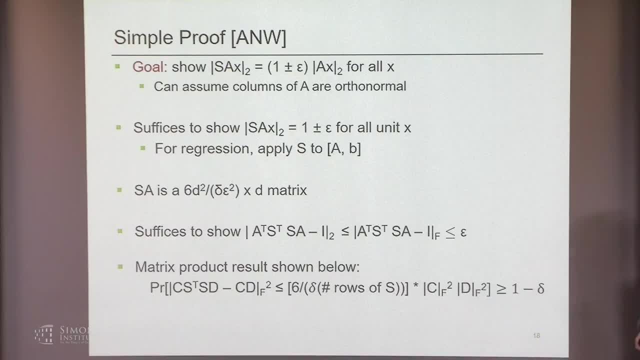 And it's going down, sort of the error is going down linearly And that, um, yeah, So any questions about this? So this is what we're going to show, But I just want to say that once we have this property, 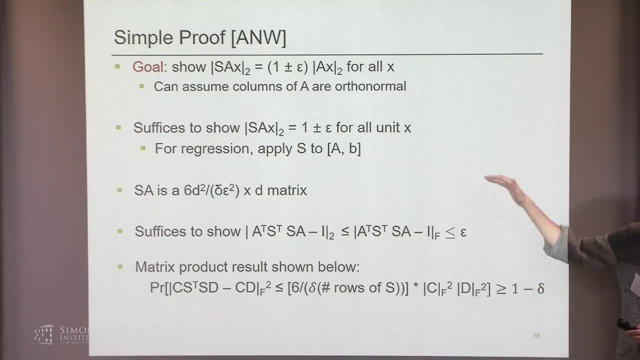 this approximate matrix product. we immediately get a proof of this statement, this subspace embedding, which I'll just give on the next line. Okay, so here is the proof. So all we do is, if we have this matrix product, result. 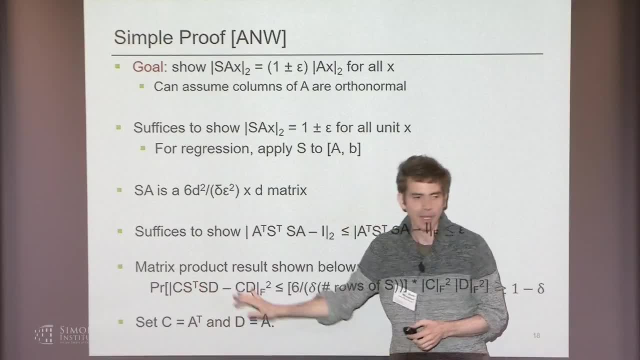 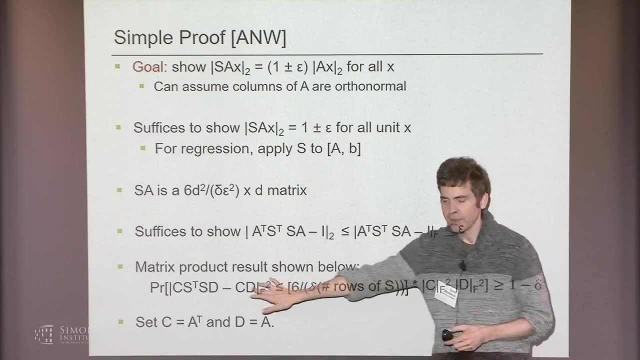 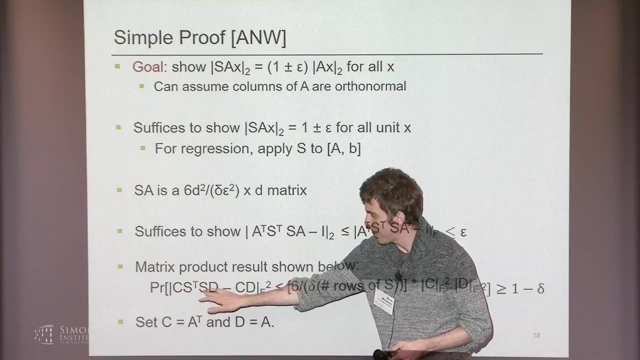 set C to be A transpose and D to be A. Now, remember, A has orthonormal columns, So what is C times D? That's just the identity. And you know what do we get? We get A transpose S transpose S times A. 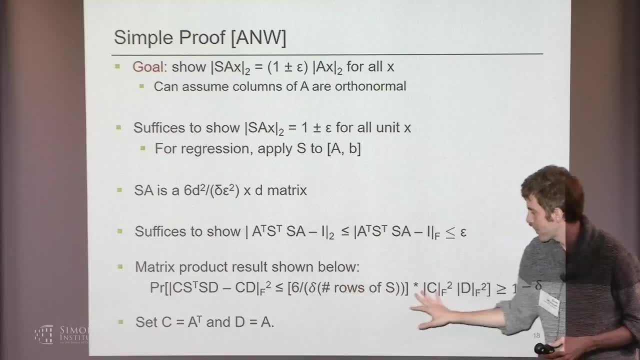 minus the identity Frobenius norm. squared is at most something That's exactly, you know, of the form that we would like to show a subspace embedding. And so how many? the question is, just how many rows of S do I need to choose? 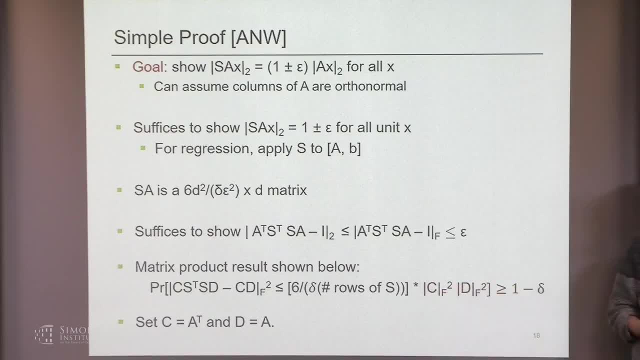 Well, what is the squared Frobenius norm Of A? Well, it's a matrix with orthonormal columns. Right, It has D columns. So the squared Frobenius norm of that matrix is D. The squared Frobenius norm of D, which is just A transpose: 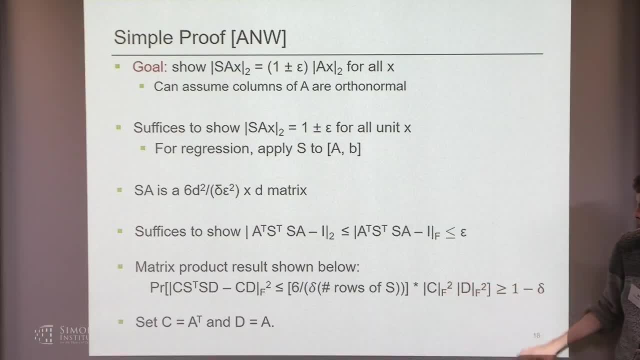 is also D. So I get a D squared here And I just need to set my number of rows to be roughly D squared to cancel this D squared. Okay, so more precisely, if I set my number of rows to be 6D squared over delta epsilon squared? 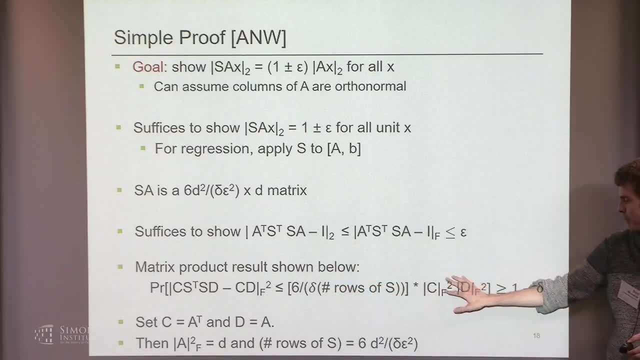 the D squareds cancel, this delta cancels and I'm left with an epsilon squared here And after taking square roots, I get back this epsilon that I asked for. Yeah question Fred: Does this imply that this D squared is sort of an artificial? 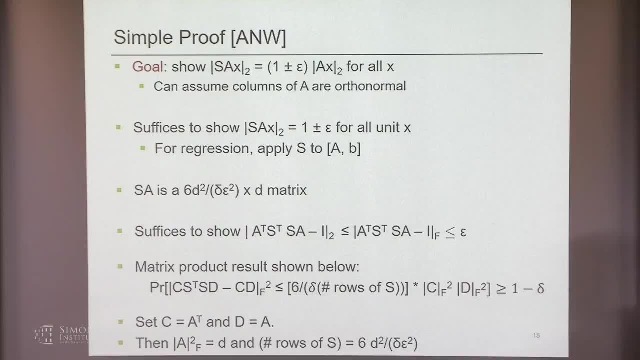 No, so actually for the count sketch matrix, D squared is actually tight. One way to look at that is to look at the identity matrix. So one way of viewing the count sketch matrix is by caching rows into buckets And if you have fewer than D squared rows in your sketch, 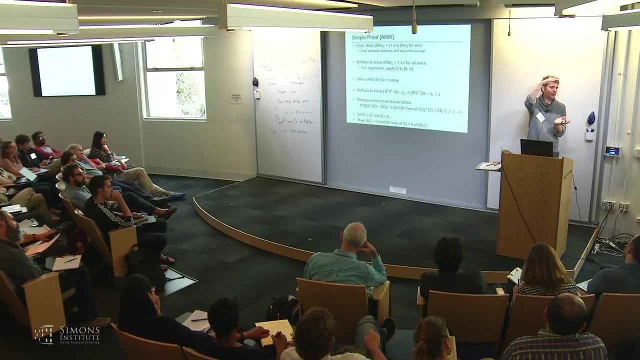 then you'll get a collision And so your rank will go down from D to something like D minus 1, so it can't be a subspace embedding. So actually this turns out to be a tight analysis for count sketch, But you can apply the same analysis. 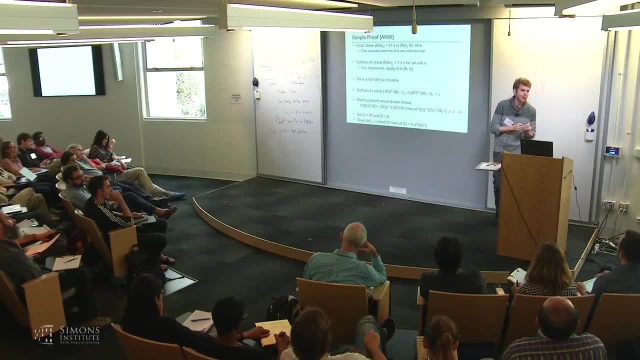 to those earlier sketching matrices like Gaussians and subsampled randomized Hadamard, And for those it's not tight as we saw. Yeah, Any other questions? Yeah, If you have anything with more than D squared, does D squared also work? 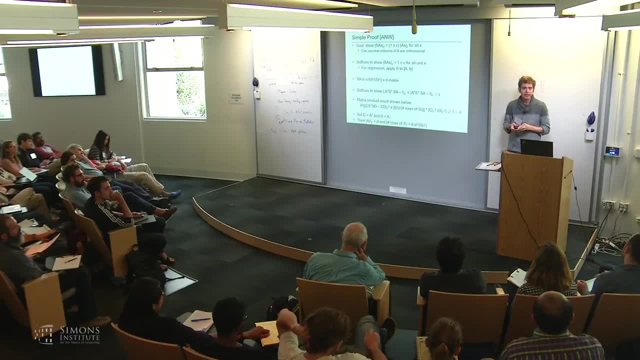 It doesn't affect your computation, right? Yeah, you can use more than D squared here. yeah, Still in the order of non-zero entries. Yeah, it's still like n and z of a number of non-zero entries of a. 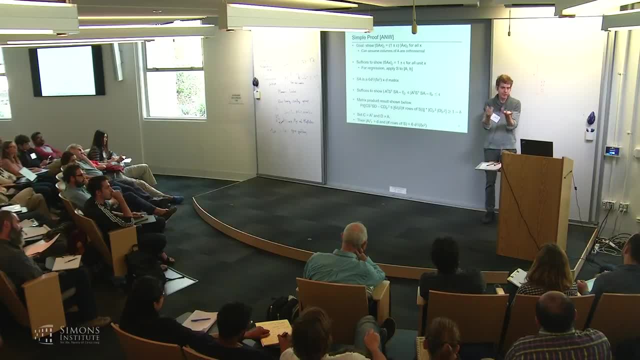 time to reduce it to this problem. And then now, if you use more rows, you have to spend more time on the smaller problem. And, by the way, one other thing I did want to mention is that, going back to Fred's question, 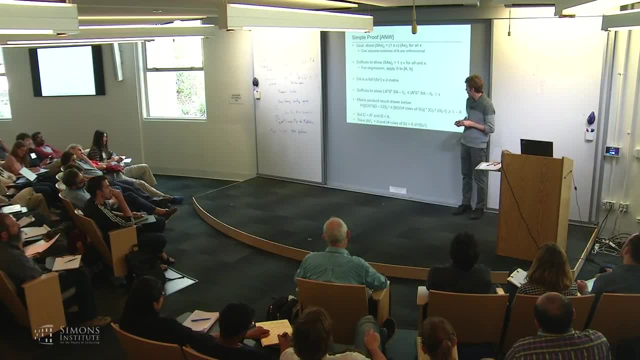 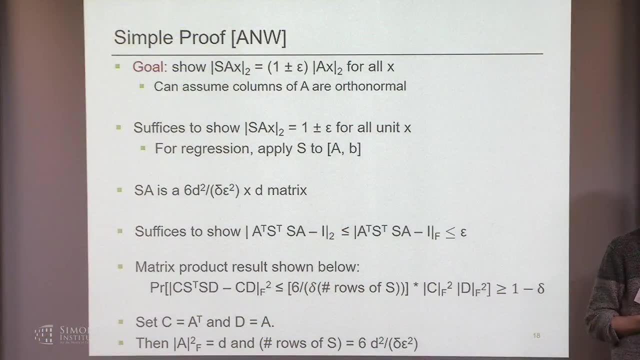 is, you can get better bounds if you have some assumptions on a. For example, if the so-called leverage scores, which we'll see later in this workshop, if they're all small inside of your matrix A, then actually count. sketch can. 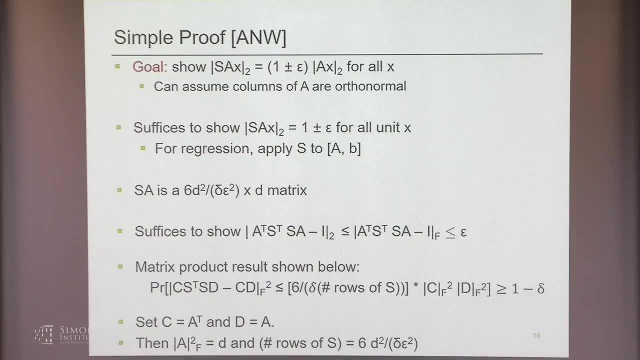 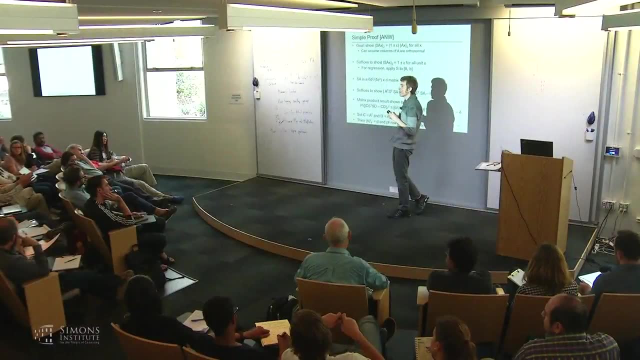 this can be shown to work with only roughly D rows. Yeah, But under no assumptions. this is tight Yeah Question. So, in general, you're saying that this gap of this extra factor of D is necessary if you want to have a sparse matrix? 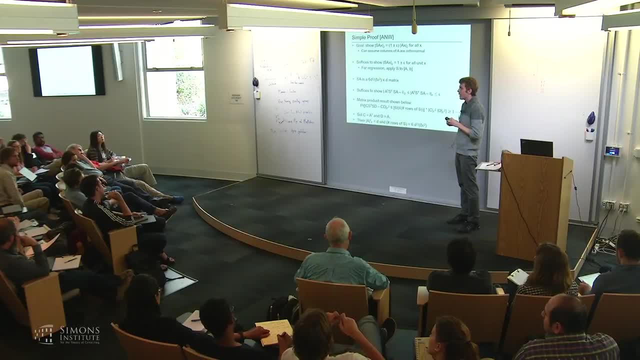 sort of bound guarantee of n and z of a In general, Like for a count sketch for one sparse yeah. So there are very nice trade-offs of Nelson and Nguyen which showed a trade-off between the sparsity in the number of non-zero entries in each column of S. 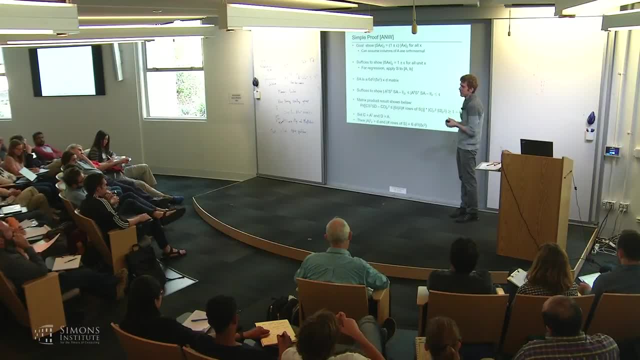 and the number of rows you need in your sketching matrix. So if I allow for like 100 non-zero entries per column of S, then I can reduce, you know, the number of rows of S times A to something like D to the 1.1.. 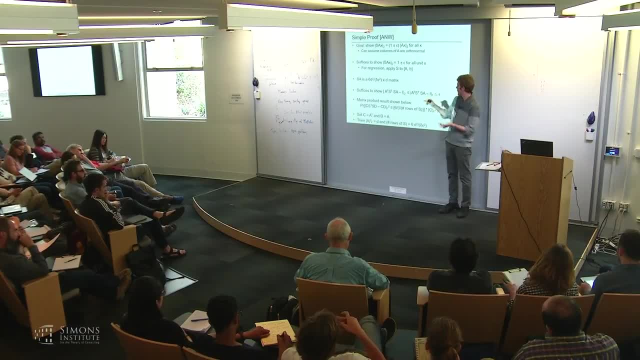 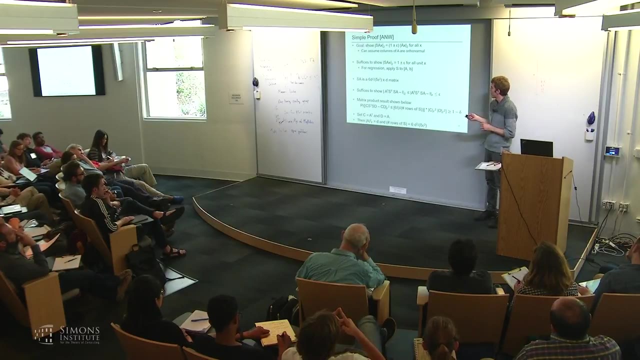 In general, like, if I allow, like poly log D, I can reduce this down to D poly log D rows. I think the latest result is due to Michael Cohen on this. Yeah, Any questions? Okay, Okay, so you know. it remains to complete this proof. 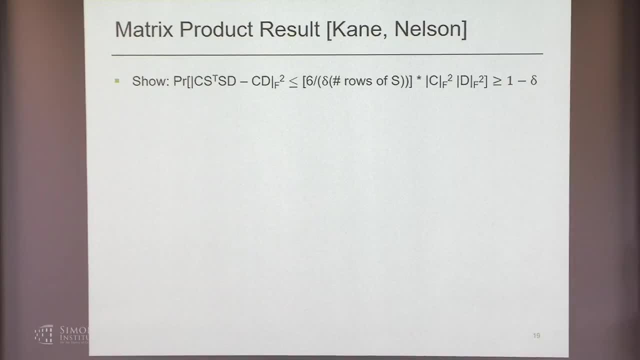 to give this matrix product result. You know, I just sort of claimed this. So why is it true? Yeah, we want to show that the squared norm of C- S transpose S D minus C D is small. Okay, so to prove this. 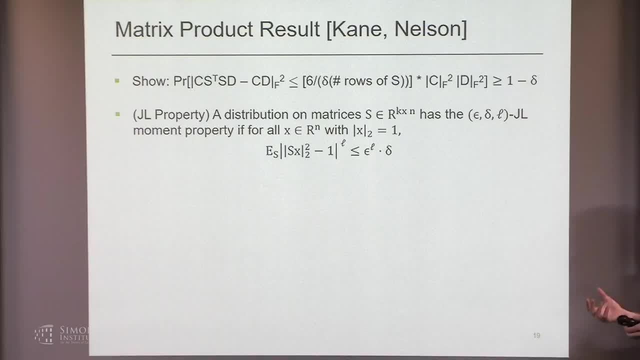 so there are many ways of proving this. We're going to do a very slick way due to Kane and Nelson, which is the following. Let's say, a distribution on matrices S has the J? L property, Johnson-Lindenstrauss property. More precisely, it has the epsilon delta L, J L moment property. 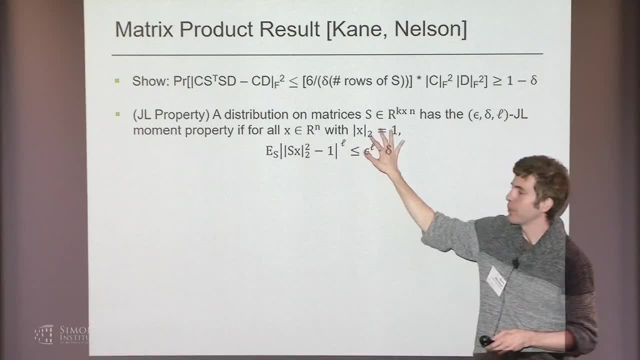 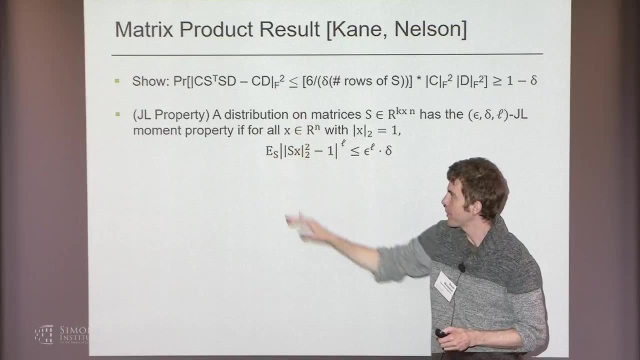 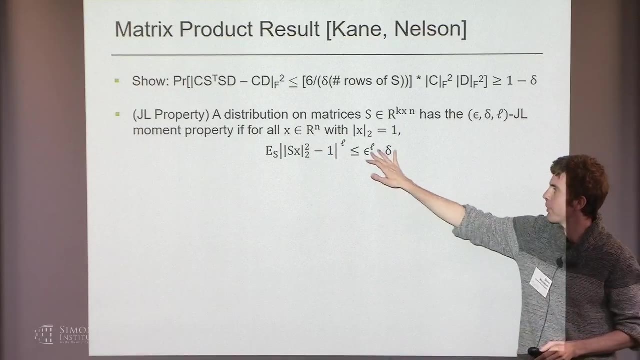 If, for any given vector X with unit norm we have the following property: It has the expectation, over a random matrix S. from this distribution of the Lth moment of the squared norm of S. X minus one is at most epsilon to the L times delta. 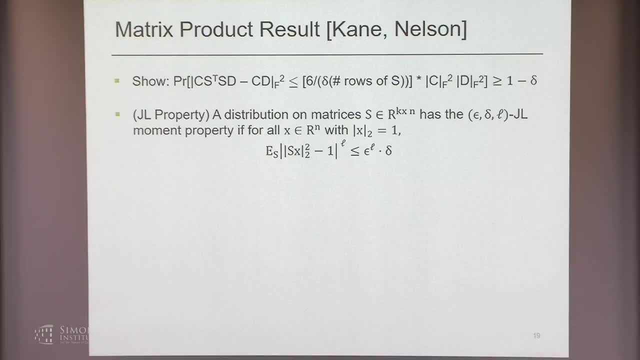 Okay, so this is giving us some control over the higher order moments of, you know, length preservation. So you know, similar to you know. so Ravi was talking about some of this earlier. So yeah, so it has epsilon delta L, J, L, moment property. 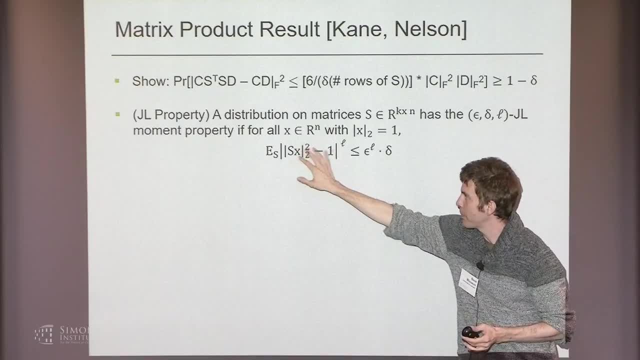 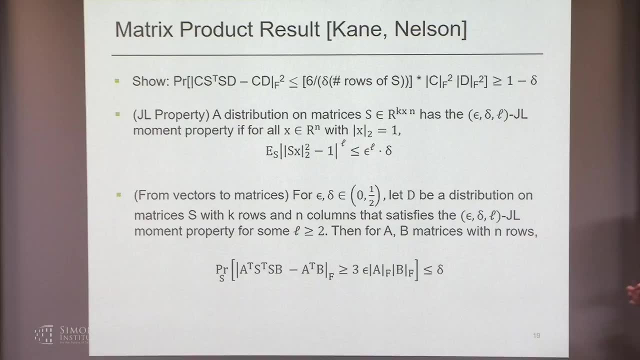 If the Lth moment of S, X squared minus one, this is small okay, And so this is just a statement about distributions of matrices applied to vectors X, And we'd like to go from this statement to this approximate matrix product statement that I said. 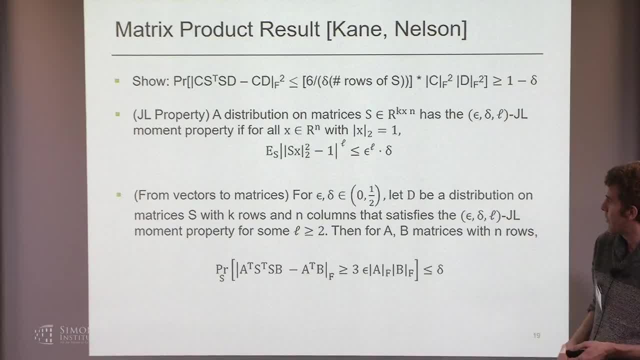 So the transition is the following: So let D be a distribution on matrices S with K rows and N columns that has the epsilon delta L, J, L moment property for some L, at least two. Then for any fixed matrices A and B with N rows, so you can multiply them. 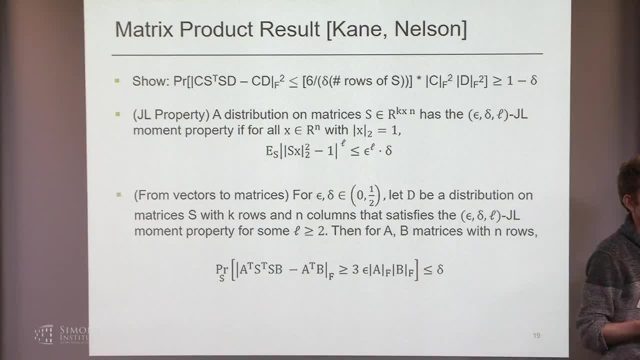 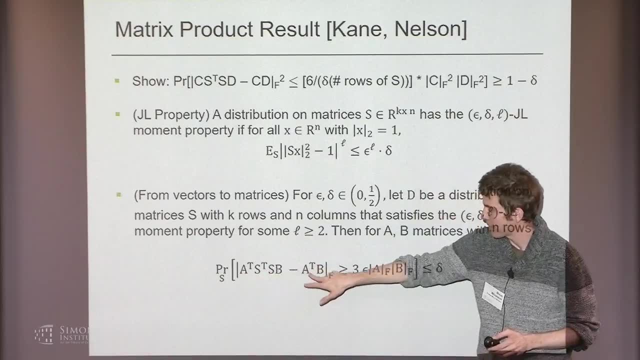 you get this approximate matrix product. guarantee that, namely the probability over S, that the norm of your approximate matrix product- A transpose S, transpose S, B minus A transpose B- the probability that it's large is small. Okay, So it's the same number of rows. 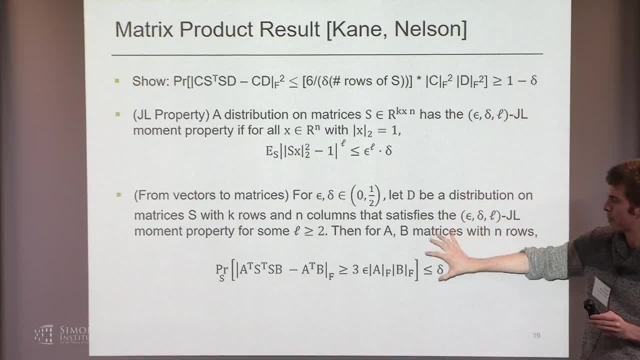 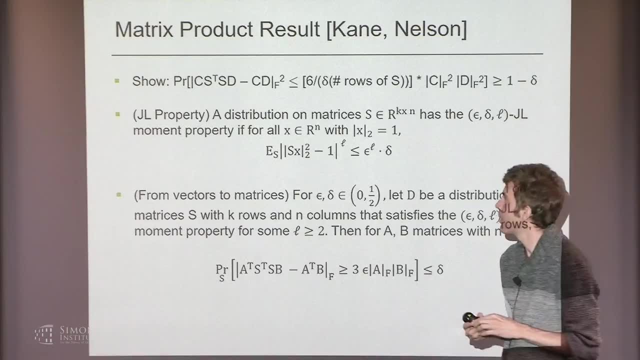 that you use in your J L moment property and you just directly apply it to matrices and you get this statement about matrices. Good question, Yeah here. How is that different than the what you need to show? Are they the same statement? 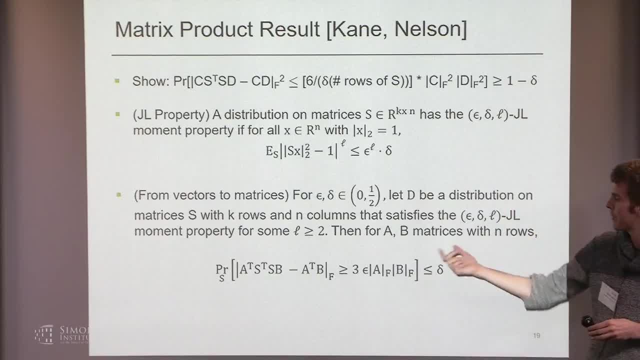 Yeah, these are the same statement. I've just written it slightly differently here. So if you rearrange things here, you know, put less than here, put greater than one minus delta, et cetera, you'll get back the same statement. yeah. 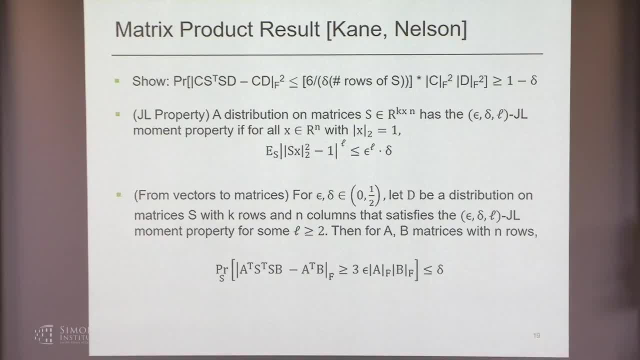 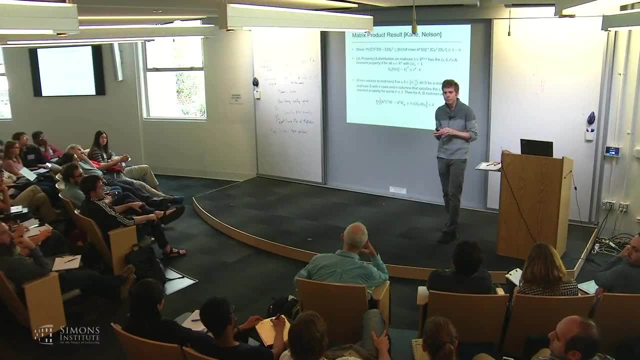 I'll mention that more later. yeah, Any other questions In the problem that you started with? B is A right Meaning, so it's more structured. Could we do better? I mean, Oh, can you do better if, like, A and B are equal? 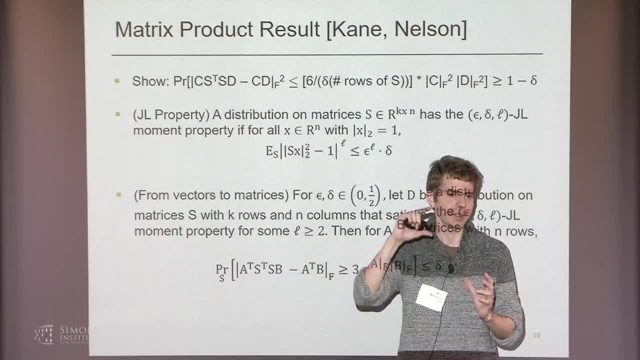 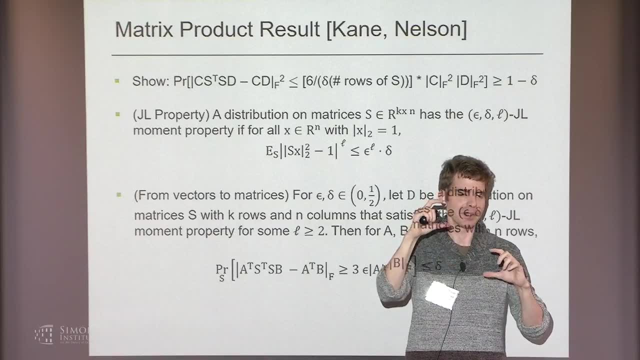 Yeah, Yeah, I don't think so. I mean not asymptotically, because you can kind of: yeah, I mean maybe look at a block matrix where A is inside and B is inside, and so I'm not sure. I don't think you can't do better asymptotically. 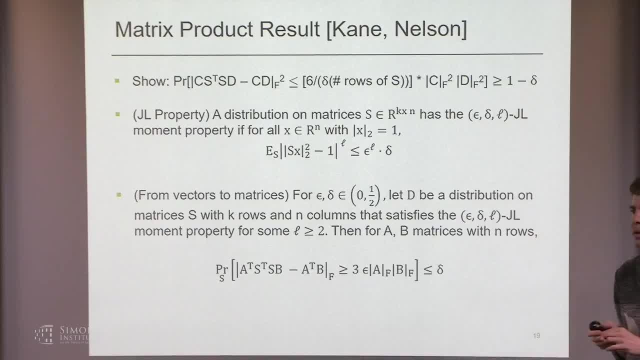 You might be able to do better in constant factors. yeah, Okay, Any other questions? Okay, Sorry, one other comment. Wouldn't the analogous statement there be about inner products of unit naught? You're just saying from vectors to matrices. 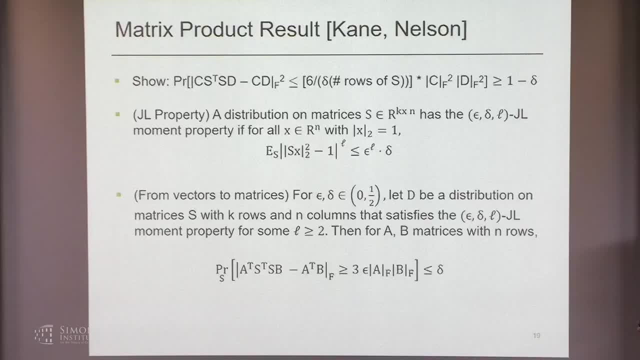 Yeah, so this, you know, this product is really a collection of inner products. you know, between the rows of A, transpose and B and the columns of B, and that's you know how we're going to prove this. 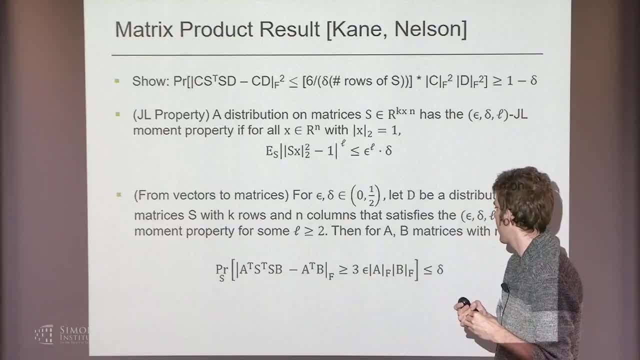 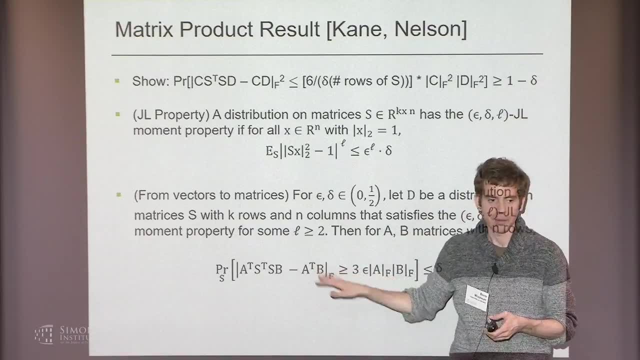 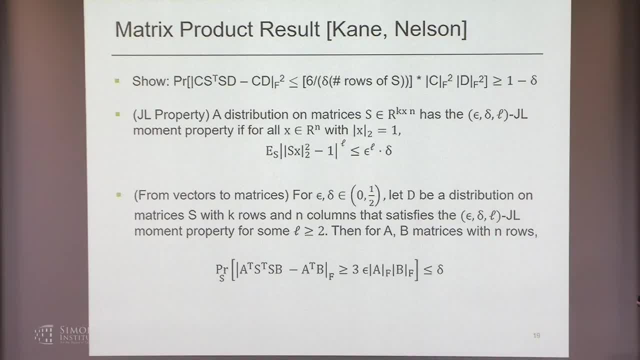 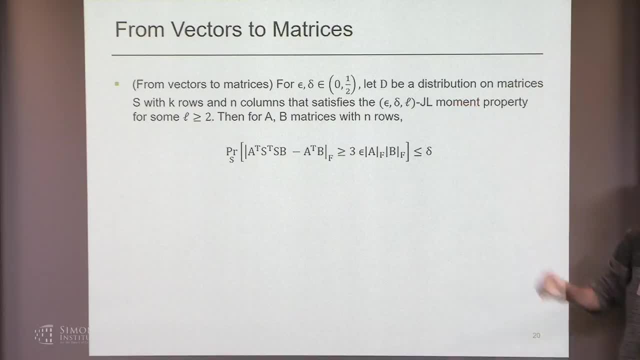 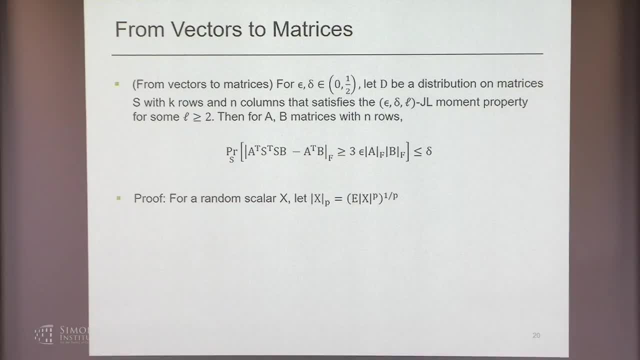 has the JL moment property. Okay, So how do we prove this? Okay, So let's set up some notation For random variable X, a scalar random variable. let's define the P norm. I didn't say why it's a norm, yet. 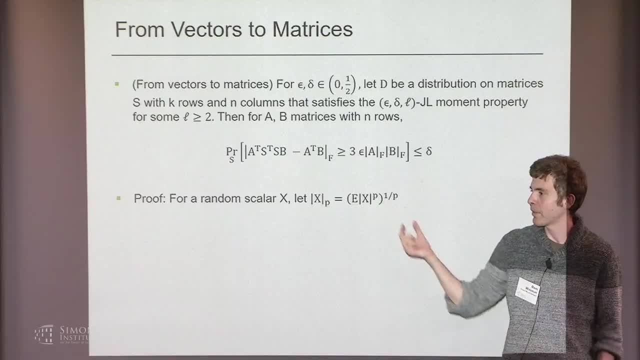 The P norm of X to be the expectation of the absolute value of X to the P right, Raised to the one over P. Okay, And you know how are we going to apply this? Well, in our proof, sometimes, this scalar X will be. 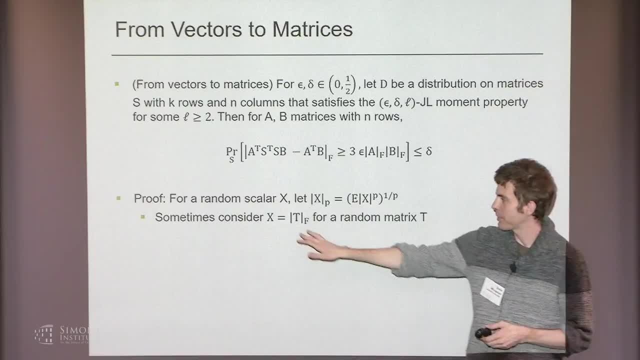 the Frobenius norm of a random matrix, T for example. Okay, So, right. So, and then you would just get that the P norm of the Frobenius norm of T is the expected value of the Frobenius norm of T. 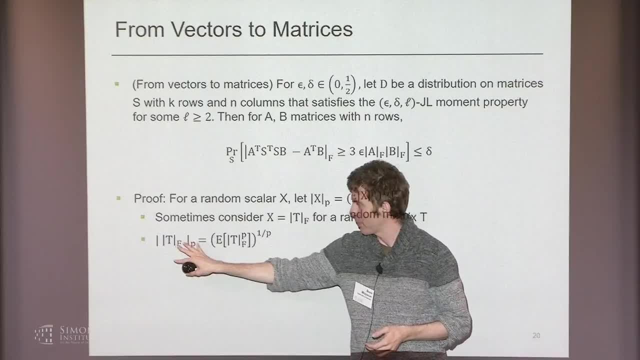 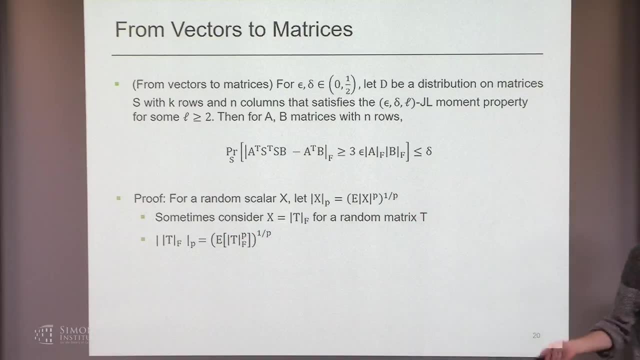 to the P raised to the one over P. Okay, Now you can see that the P norm of X is the expected value of the Frobenius norm of T to the P raised to the one over P. Okay, Now you can show. 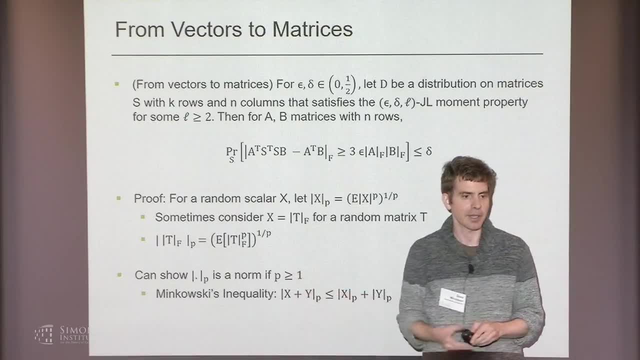 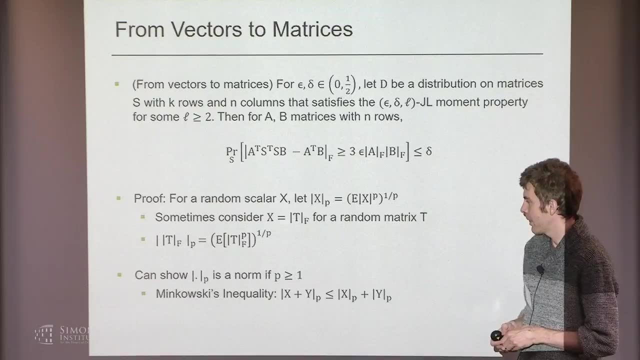 that this P norm is actually a norm for any P, at least one. Okay, So it you know. it's zero at zero. The main thing to show here is the triangle inequality, And the triangle inequality turns out just to be. 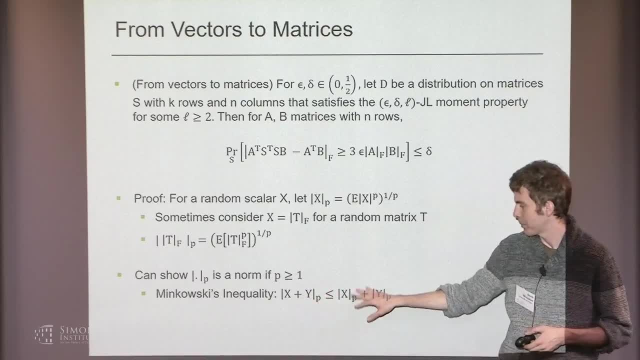 Minkowski's inequality. Okay, That the the P norm of X plus Y is at most the P norm of X plus the P norm of Y. This is Minkowski's inequality, and it basically comes down to Holder's inequality in the proof. 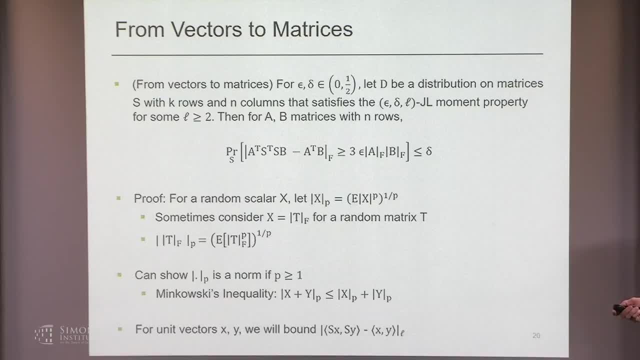 I won't, I won't prove that here. Um, okay, So all right. So let's, let's look at unit vectors X and Y And let's bound the L norm of the difference in inner products between the sketch. 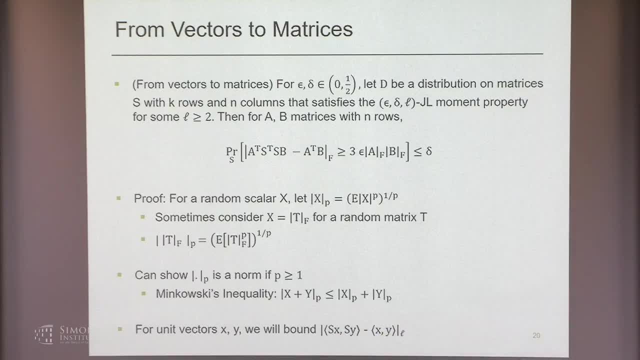 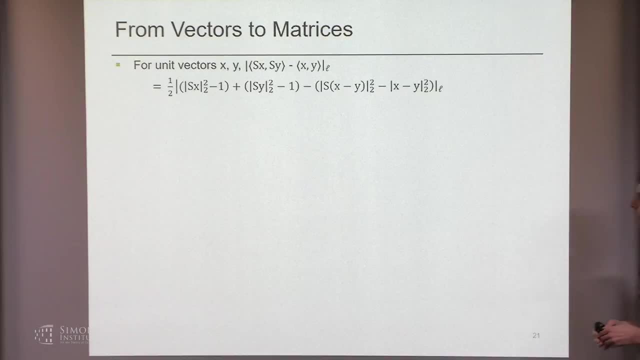 you know SX, SY, that inner product, and the actual inner product, XY. Okay, So this will be a useful primitive to have. Okay, So what is the expression for this difference? Well, one way of writing this is: 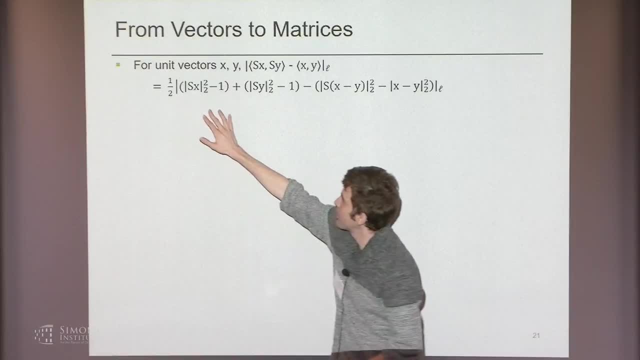 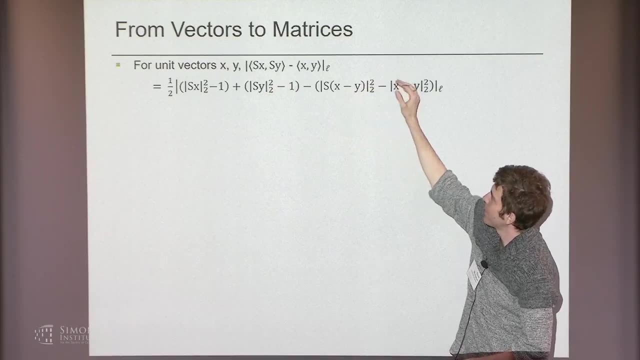 I claim is the following: So it's one half times the squared norm of SX minus one plus the squared norm of SY minus one, uh, minus, uh. the squared norm of SX minus Y, minus the squared norm of X minus Y. 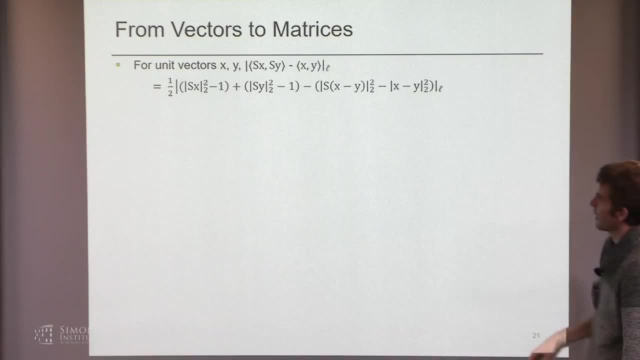 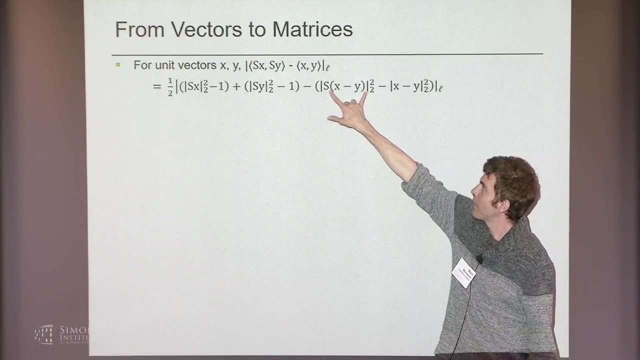 What's going on here? All that's going on here is: I'm taking, uh, you know one of these expressions and I'm just expanding it. So the squared norm of SX, of S times X minus Y, is the squared norm. 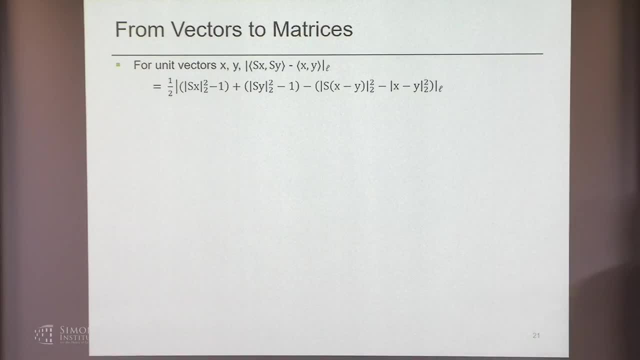 of SX plus the squared norm of SY, minus twice the inner product of SX and SY. All right, That's all that's happening. So the squared norm of SX here will cancel this squared norm of SX. The squared norm of SY will cancel. 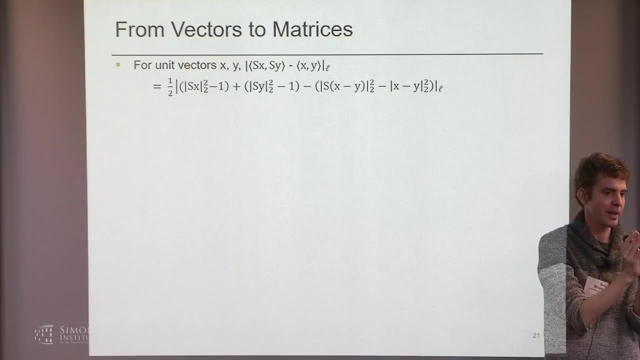 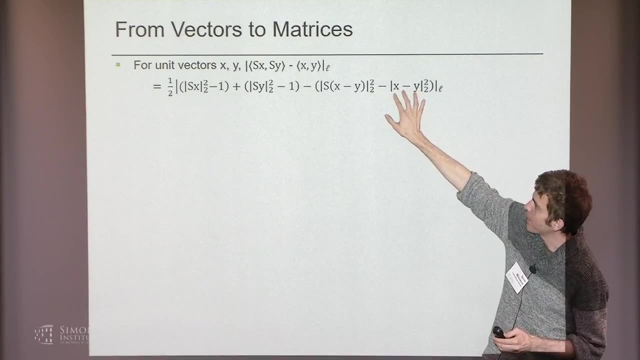 this squared norm of SY, Um and uh. I also do the expansion for the squared norm of SX. These are unit vectors. So the squared norm of X, the squared norm of Y, those are both one. Those will cancel. 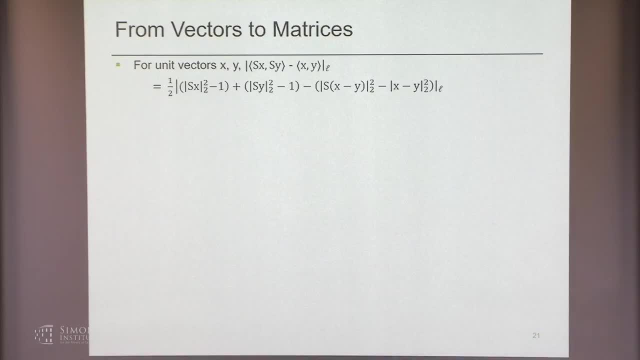 these ones, And so you know, I'll get twice this difference and I have a one half in front. Okay, So that's all I've done, Okay. Now I'm looking at the L norm of this quantity And 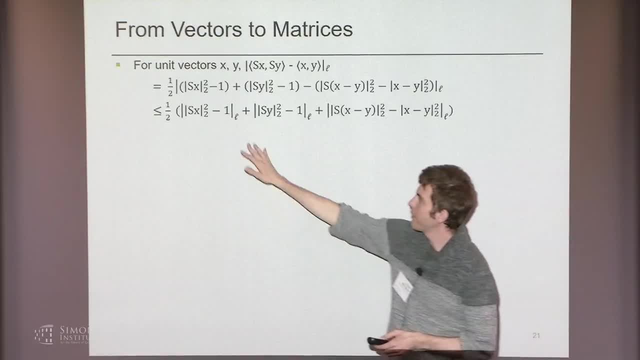 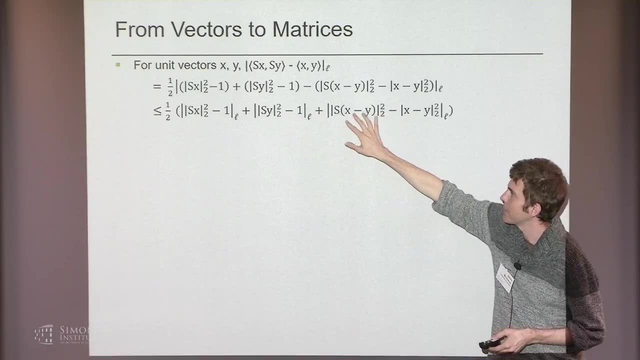 what do we know about the L norm? Well, we know it's a norm. So in particular, I can apply: L norm plus the L norm of SY squared minus one, plus the L norm of SX minus Y squared, minus X minus Y squared. 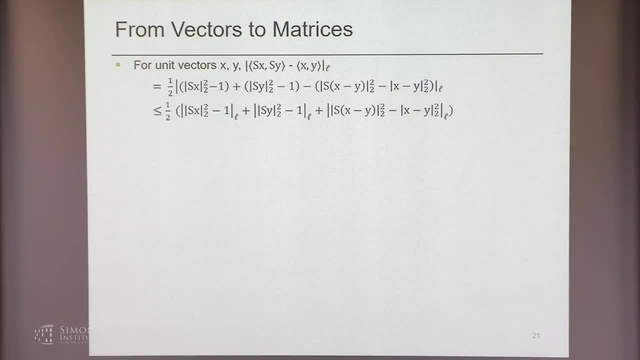 Okay, Everyone is with me. Okay, Okay, And uh, what do we know about each of these things here? I mean? so remember this transition statement We're trying to prove: if S has the JL moment property, then it satisfies something. 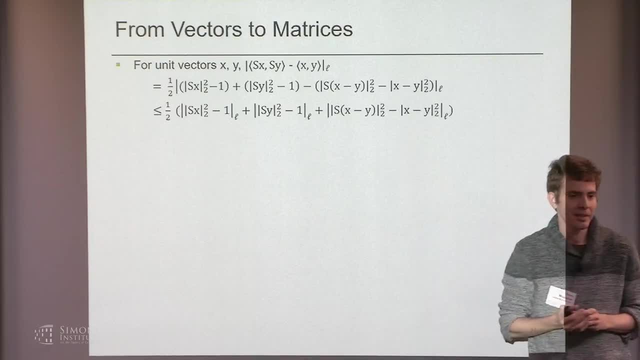 about approximate matrix product. So what does the JL moment property tell us? I mean, it tells us how to bound each one of these terms right. X is a unit vector, Y is a unit vector. X minus Y is not a unit vector. 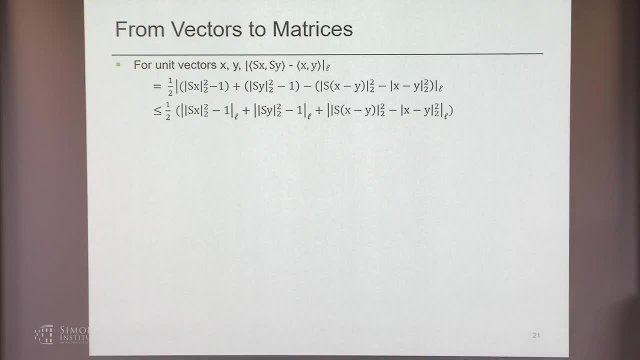 but I can just, you know, factor out the norm of X minus Y. So just directly applying the JL moment property, I get that this L norm is at most epsilon times delta to the one over L. This L norm is at most 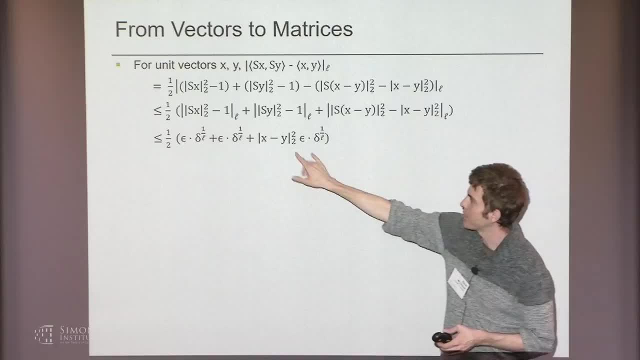 epsilon times delta to the one over L, And the last thing I get is at most the norm of X minus Y squared times. epsilon times epsilon to the delta times. epsilon times delta to the one over L. Okay, Now the norm of X minus Y squared. 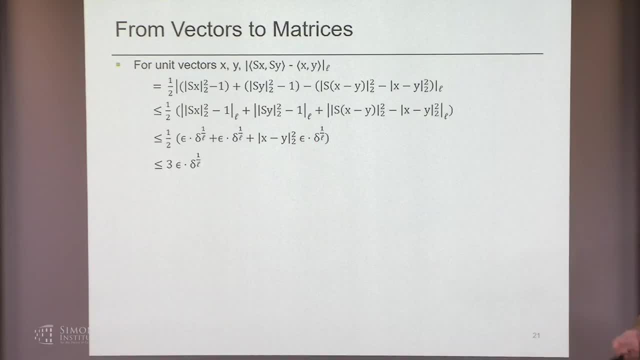 you know, is at most four. X and Y are unit vectors, So this is at most, say, three times epsilon, times delta, to the one over L. Okay, So this is just some statement about differences of inner products. So 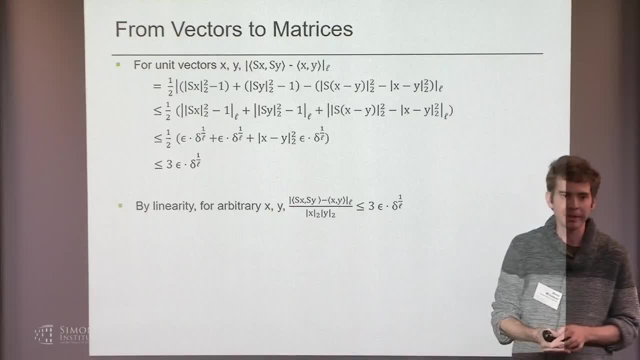 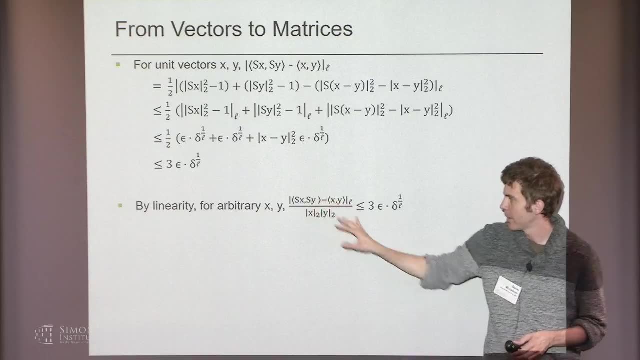 by linearity- this was for unit vectors- but by linearity for arbitrary X and Y. so I can divide out by the norm of X and the norm of Y and I get that for arbitrary X and Y. you know this inner product. 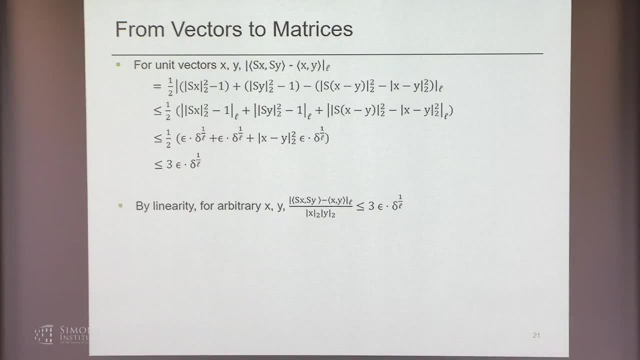 divided by the norms now is at most, say, three epsilon delta to the one over L. Okay, Clear, Okay Good. So now, why are we doing this? So, ultimately, we want to say something about matrix product. 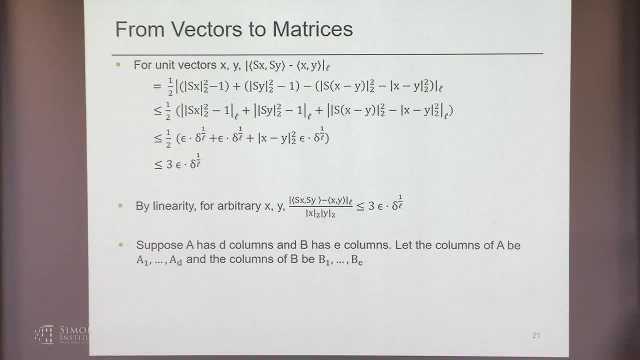 So now let's look at a matrix product. And let's look at a matrix product, So let the columns of A be A1 through AD and let the columns of B be B1 through BE. say, Let's define: 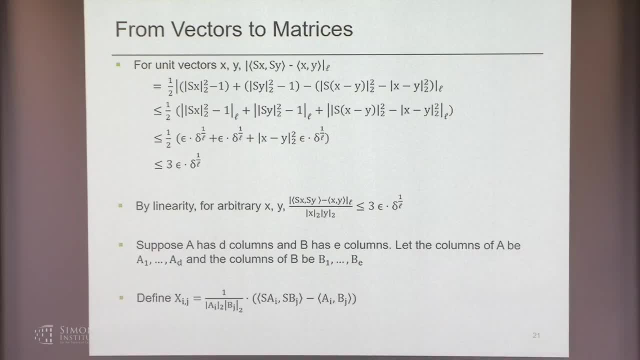 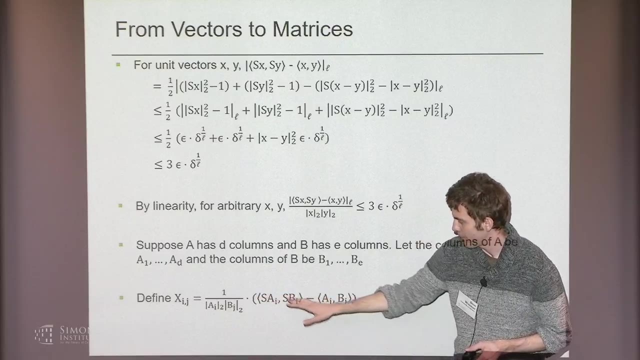 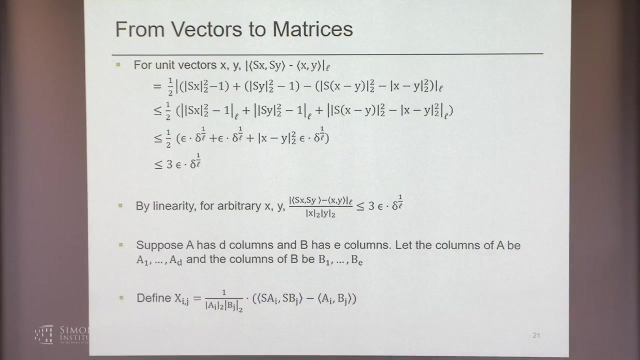 XIJ to be the following quantity: It's one over the norm of AI times, the norm of BJ times. the difference of you know, of SAI inner product to SBJ is one over the norm of AI times. AI inner product BJ. Why do we do that? 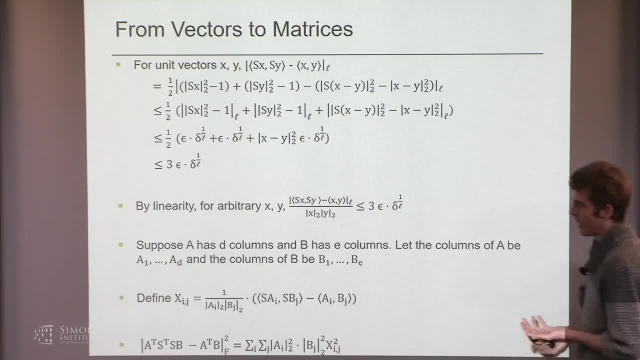 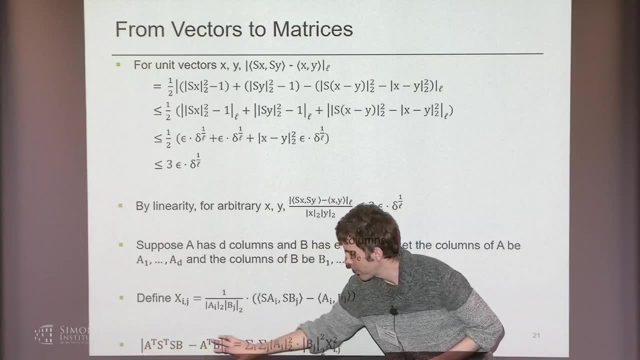 Well, that's exactly the entry in the matrix product. A transpose B. Okay, So what do we have here? We have that this squared norm of this approximate matrix product that we care about is equal to the sum over all entries I and J. 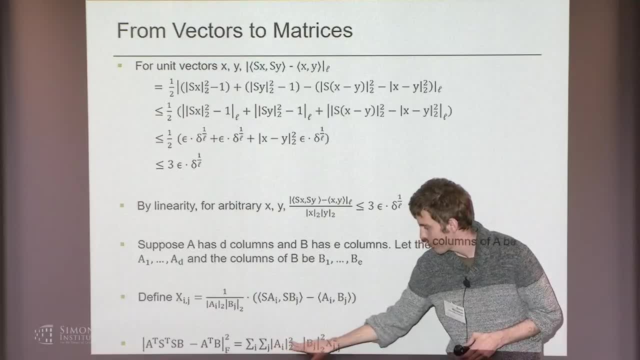 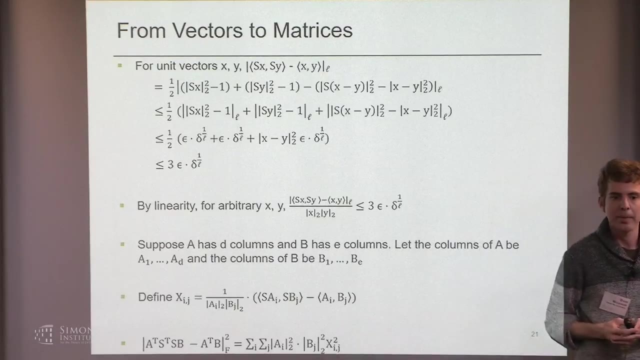 of XIJ squared times, the squared norm of AI times, the squared norm of BJ. Okay, So we're just going to bring it up like this: Is that clear, everyone? Okay, Okay, So now we just want to bound. 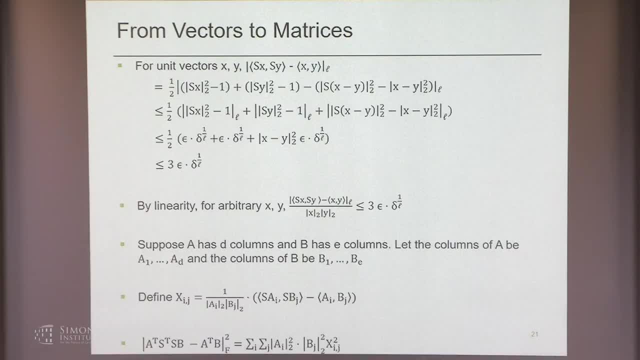 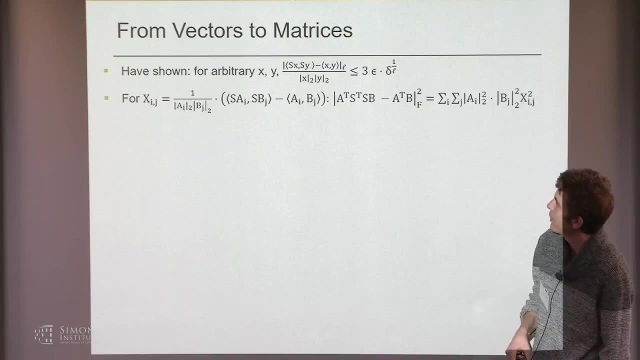 this quantity, Okay, So let's do that, Okay, Good. So what have we shown so far? We've just shown this statement for arbitrary vectors X and Y. You know, we have some bound on the difference of inner products. 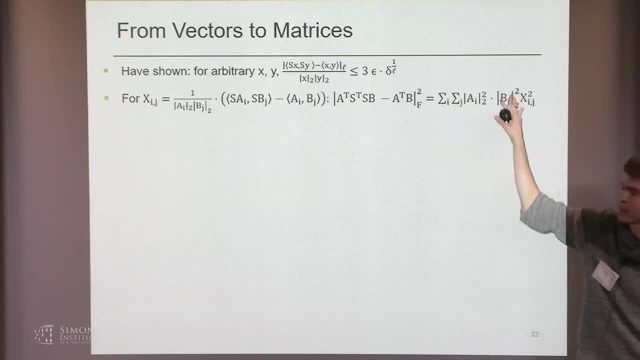 over the norms We've shown for these XIJs and we showed our matrix product can be written in terms of those XIJs. Okay, So let's look at the following quantity and it'll be clear why we're looking at this in a second. 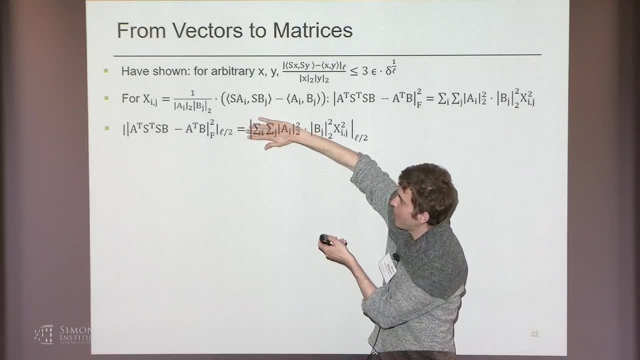 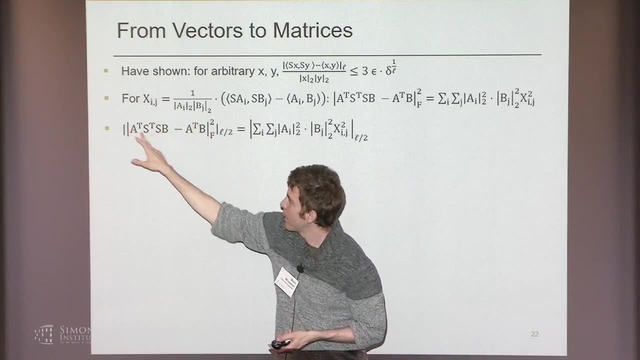 So I want to look at a norm, you know. so I'm going to look at the L over 2 norm of the Frobenius norm, or rather squared Frobenius norm, of this matrix A, transpose S, transpose B. And we just said: 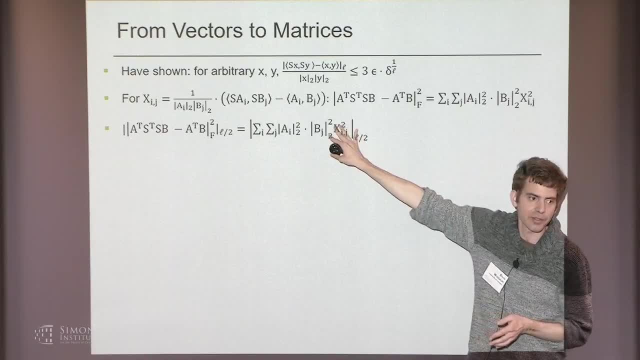 that we can write this matrix using this expression in terms of the XIJs. Okay, so that's all I've done there. I just substituted in the definition. Okay, So what can we do with this expression? Any thoughts? if people are with me, 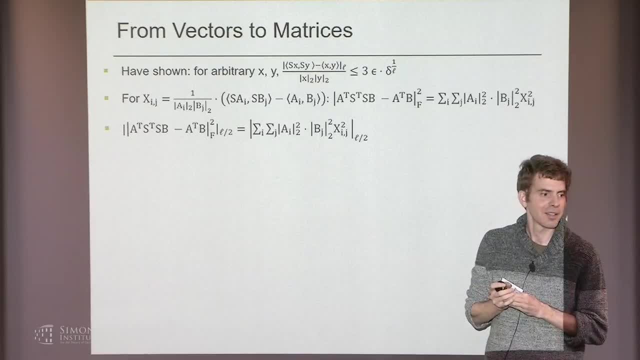 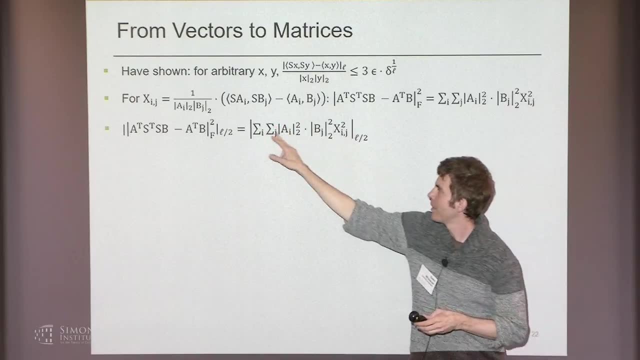 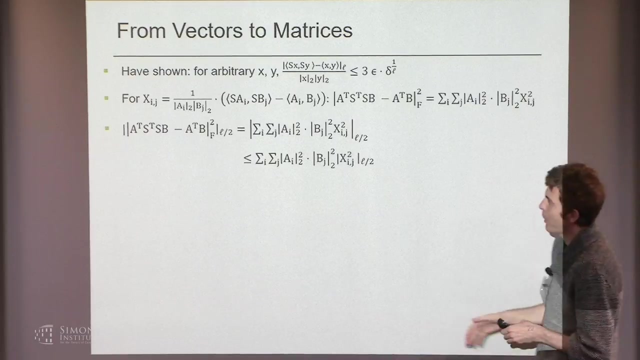 What should the first thing and what is one thing we can do with this expression? So it's the L over 2 norm of the norm of the sum of a bunch of stuff, Triangle, Triangle, Triangle, inequality, Great, Thank you. 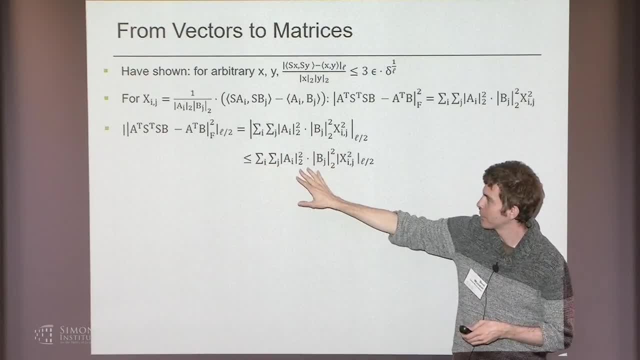 So by triangle inequality. this is at most the sum, you know, of the norms of all that stuff. So the sum over all I and J squared norm of A, I squared norm of B, J times the L over 2 norm. 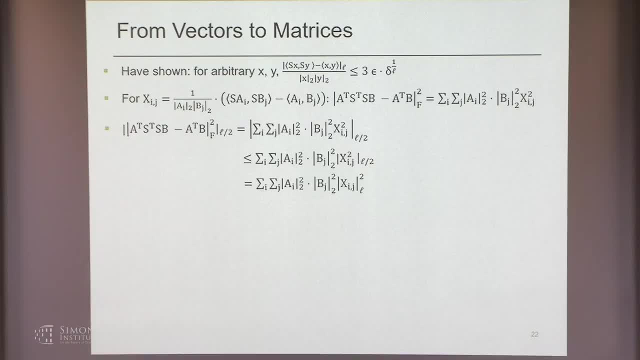 of XIJ squared Right. That's the only random variable in the equation. So now this next line. all I'm doing is I'm playing with the definition of the L over 2 norm. Remember the L over 2 norm. 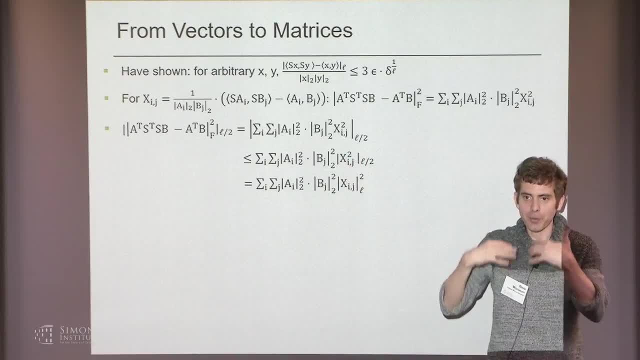 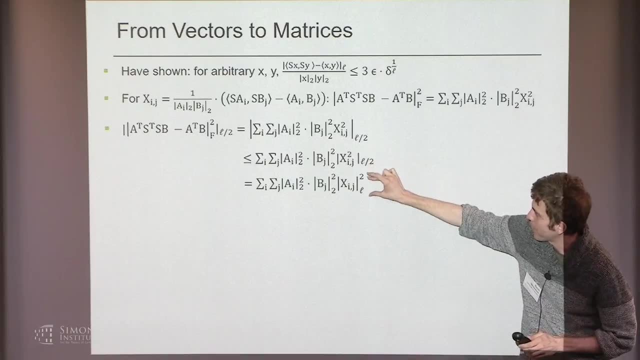 of some quantity is like that quantity to the L over 2, you know the expectation of that quantity, the expectation of the absolute value of that quantity to the L over 2, raised to the 2 over L. So this is just. 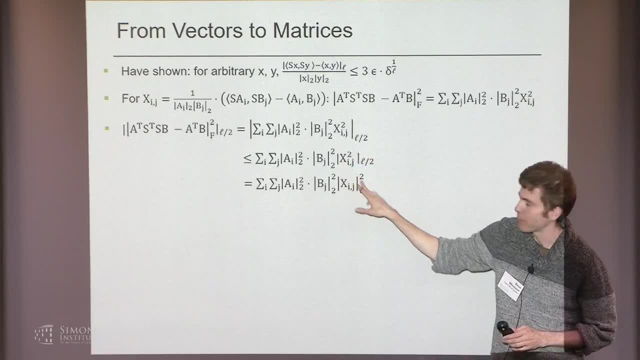 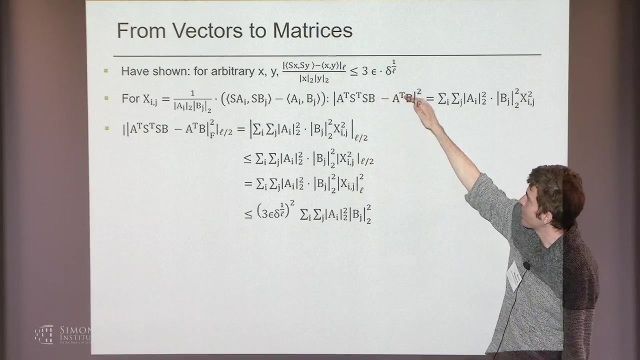 a definitional statement, right, Because when I raise XIJ squared, it's just a definitional statement, Okay. Okay, Now what do we know from you? know this statement that we have up here. Well, the XIJs had this form: 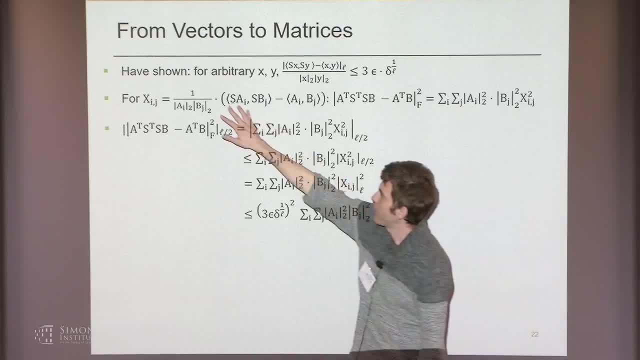 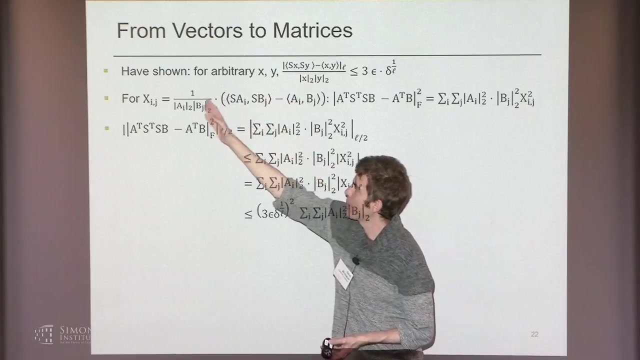 and this form is exactly what we know. we can apply this JL moment property to Right. I mean, if I look at what the XIJs, they have the form of a different L over 2 norm, of a difference of inner products, and I'm normalizing. 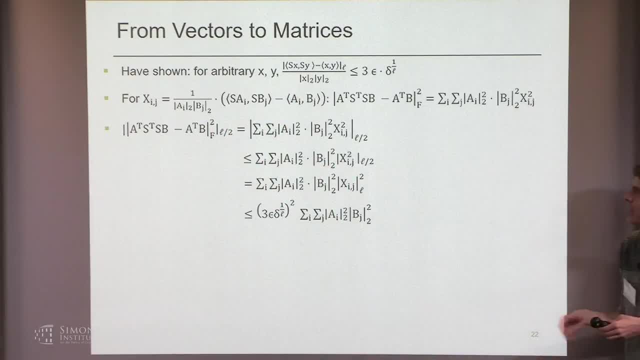 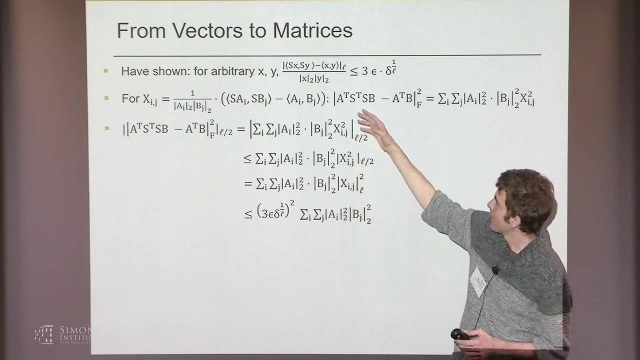 by the norms. That's exactly what we can apply, this statement that we had for arbitrary vectors X and Y. So just plugging in that statement, we upper bound this squared L norm as this value squared Okay, And I just factored that out. 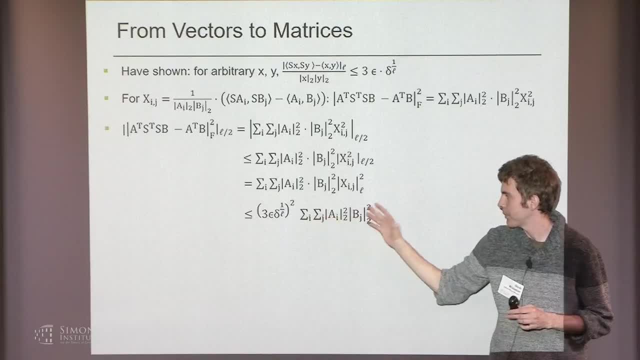 And inside I have you know the sum of squares of, you know AI squared, sum over all IJ of norm of AI squared and norm of BJ squared. And what is this quantity, Product of Frobenius, norm squared: Yeah, 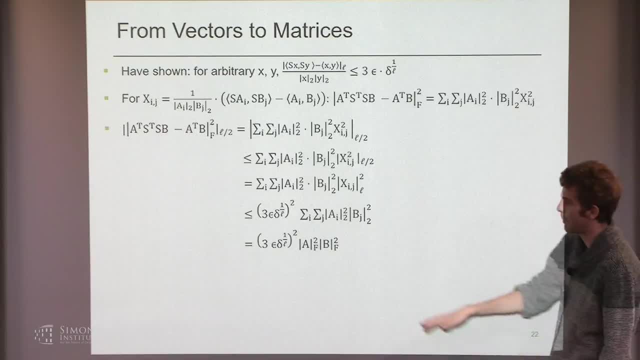 It's just the product of Frobenius norms, squared Frobenius norms. So this is just three epsilon delta to the one over L squared times, the product of squared Frobenius norms. Okay, We're almost done, We'll finish this up. 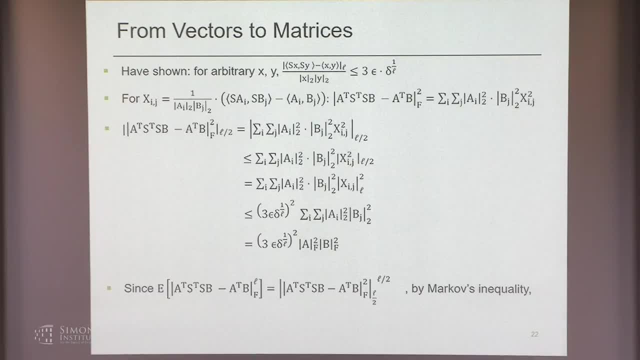 Okay. So why do we look at this quantity? Well, we're just going to apply Markov bound on a higher order moment, just like Ravi did in his talk. So let's look at the expected value of the. you know. 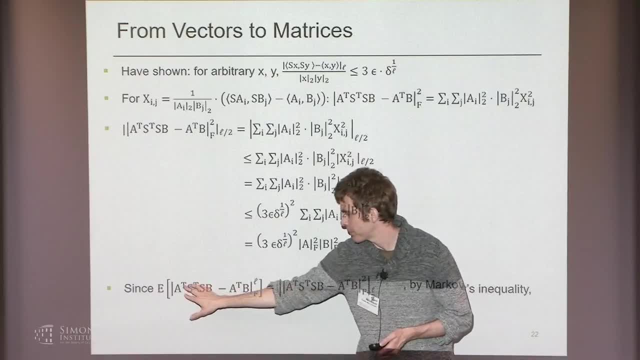 L power of the Frobenius norm of our approximate matrix product: A transpose S transpose S, B. minus A transpose B. Okay, The claim is that L over 2 to this expression that we had up here raised to the L over 2 power. 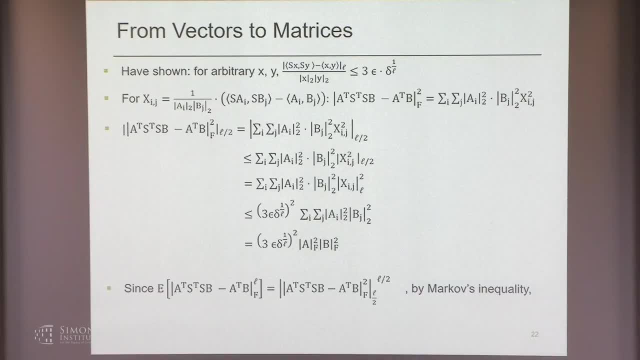 Okay, That's again just a definitional statement. Okay, So, like what is the L over 2 norm of this? Well, it's the expected value of this raised to the L over 2.. So I'll get. 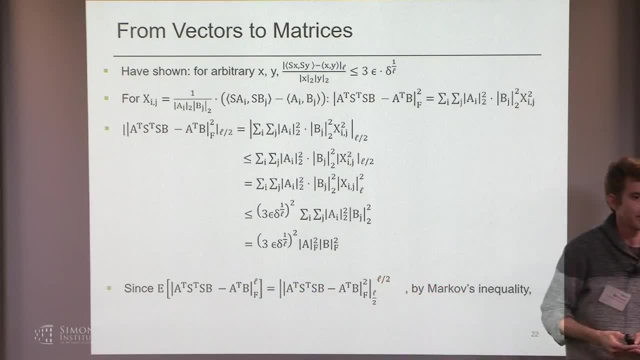 the L power here, which is exactly what's over here, all raised to the 2 over L, and that will cancel this L over 2.. Okay, But we just bounded this quantity here, So now we're going to apply Markov's inequality. 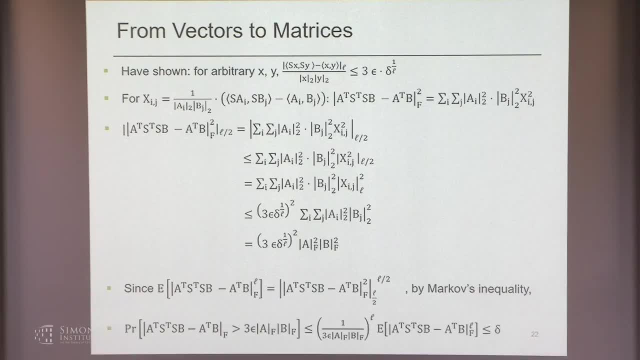 and complete the proof. So the probability that the Frobenius norm of our difference exceeds some amount. well, I can raise both sides to the L power, Right? So I raise this side to the L power. I raise this side to the L power. 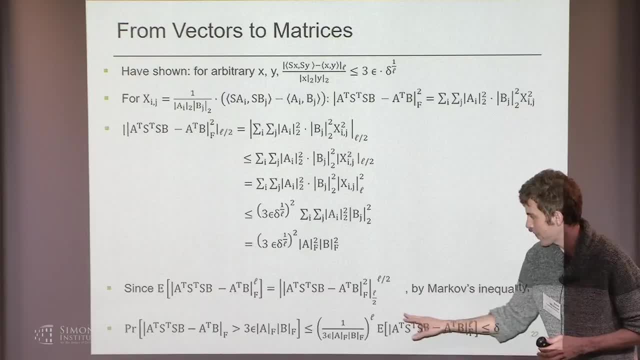 and then I just bound, So it's at most, you know, the expectation of this quantity divided by this quantity to the L power. So I get exactly this expression. And finally, you know, I just plug in the bound that we just 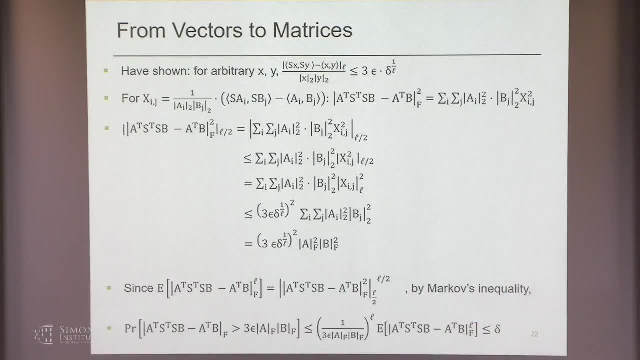 proved for this expectation. Okay, So we just showed that this expectation here is this quantity, which is the L over 2, the L over 2th power of this quantity. Right, So you know? so what happens here? I raise: 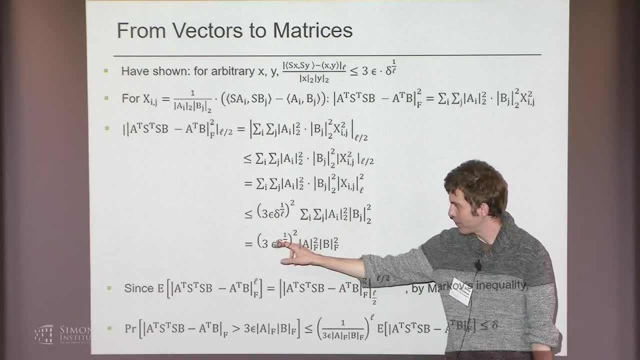 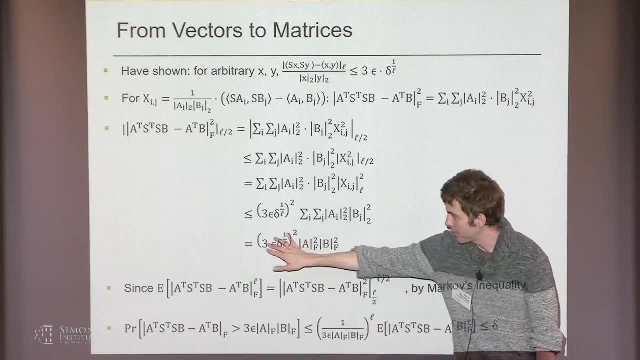 this quantity to the L over 2.. Let's just look at epsilon, for example. So I get epsilon squared to the L over 2.. I get epsilon to the L. That cancels this epsilon to the L. You know, I get 3 to the L. 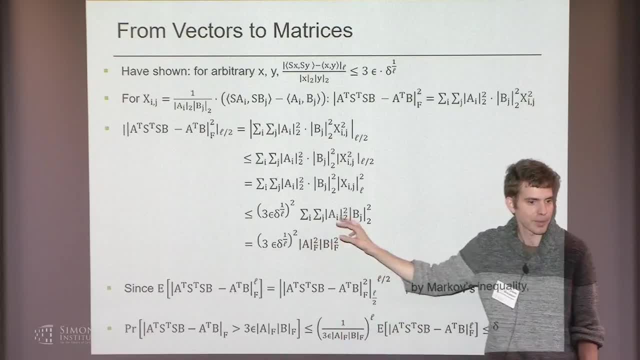 That cancels this 3 to the L, etc. Right, I get all that stuff cancels, I'm just left with delta. That's the whole argument. Okay, Is it clear? Okay, So we showed that if we have the JL property, 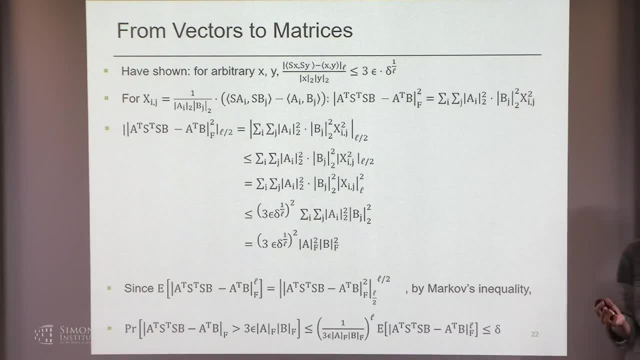 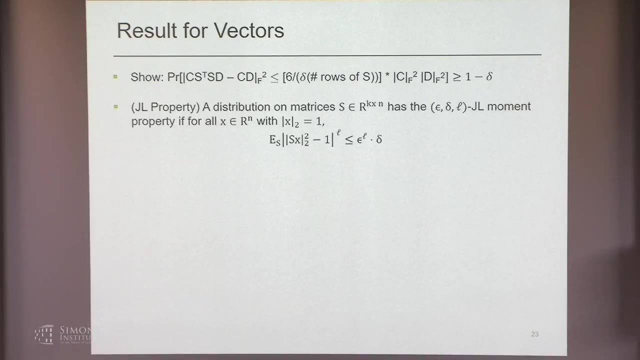 for vectors. then we get the approximate matrix product property that we wanted. Okay, So, yeah. So just recall, this is the approximate matrix product property that we wanted. We started by saying that our matrix S is drawn from a distribution which has this: 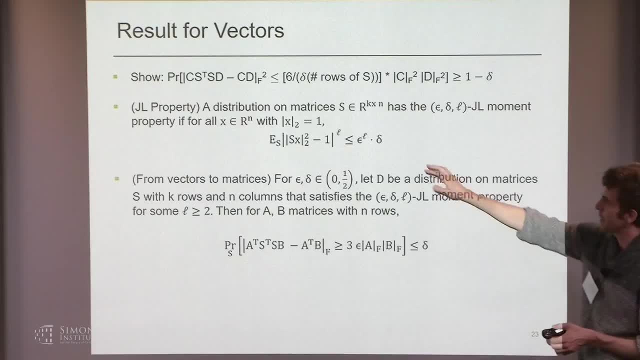 JL moment property And we said, well, if we take the same matrix S with the same number of rows, then it satisfies this approximate matrix product property. Yeah, Question, It actually doesn't depend on L at all If you satisfy it for any L. 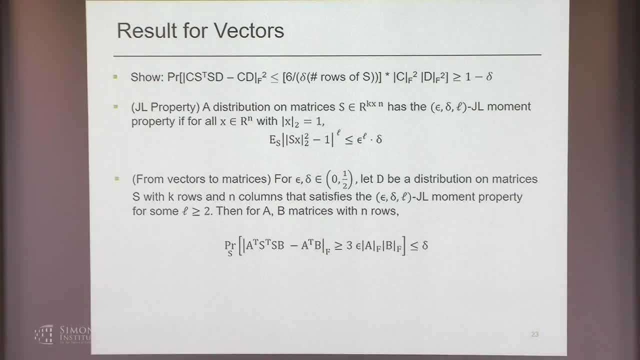 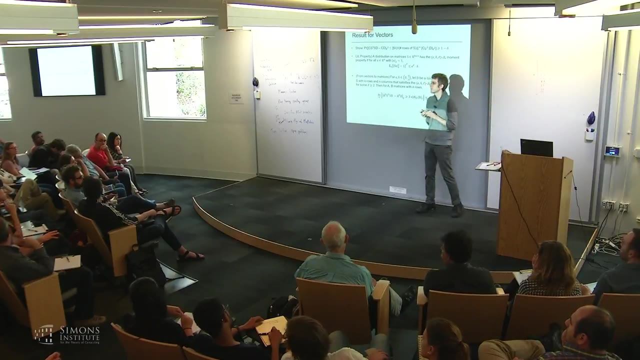 you get the same. Yeah, This is all we're going to use. Yeah, Are there natural examples for which you have to use like a strange L in some context? Yeah, So I think, Jerem, do you have? 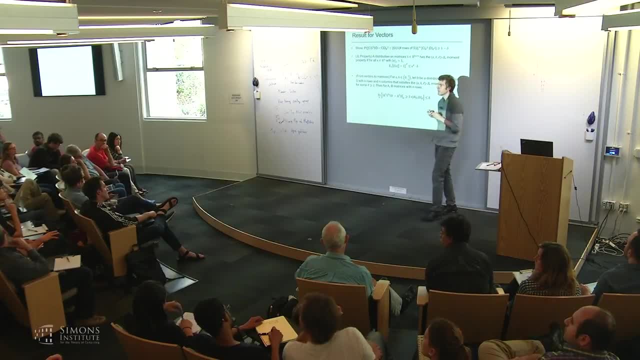 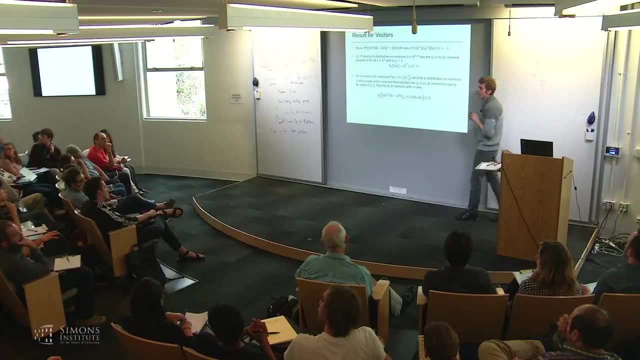 some work on this recently with Cohen and Gilani right Using other values of L for these kinds of proofs. No, not for this case. You don't need the higher. Yeah, I mean so for us, we're just going. 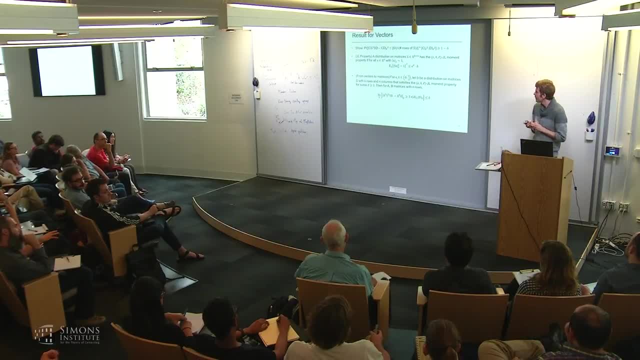 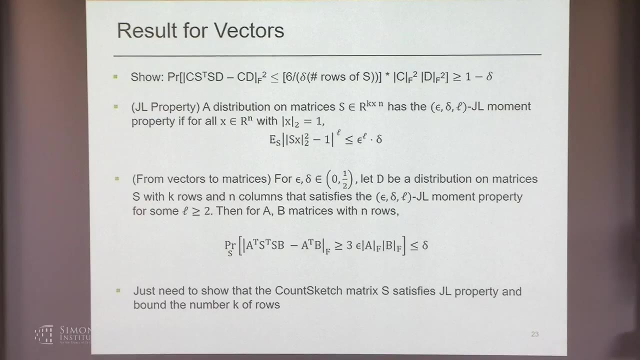 to get like 1 over delta dependence. This is all that's going to matter, and we're not going to use this kind of proof for the other families of matrices that we look at here. Okay, Okay, So we just need. 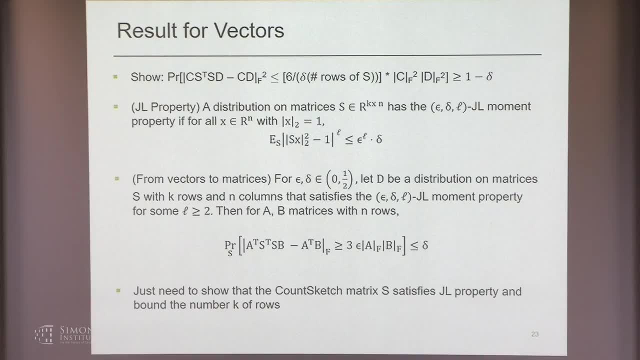 this to be at most half? Question: Yeah, Why do you need epsilon and delta to be at most half? Oh, um, let's see, Do we actually need this to be at most half? Um, I don't think this is. 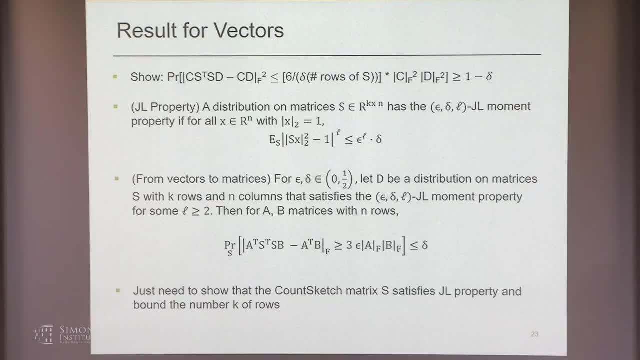 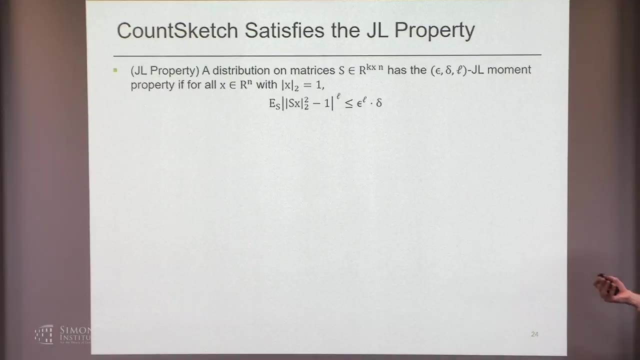 I think this is arbitrary. Yeah, this is somewhat arbitrary. Yeah, I might have been hiding some constants, but uh, okay, Um, okay, so count. sketch satisfies the JL property. This is just a, you know, a statement. 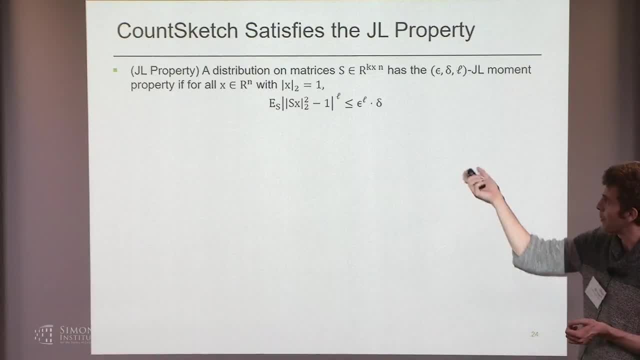 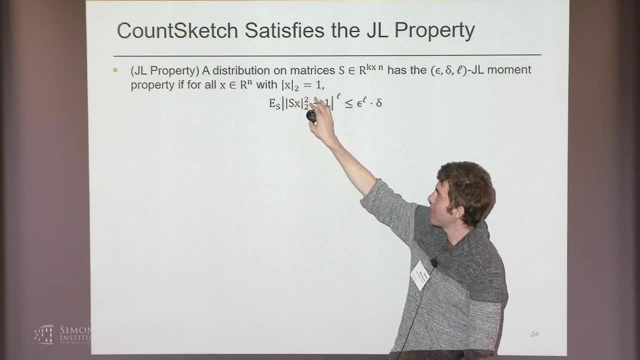 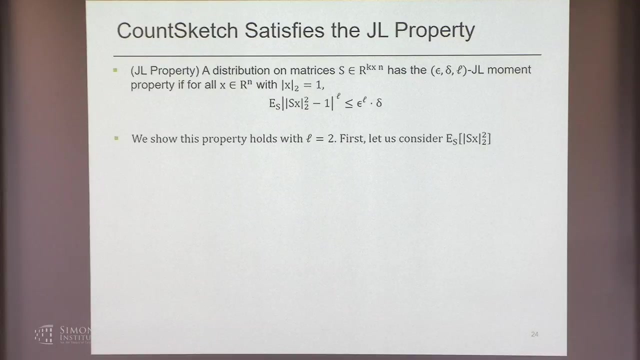 about applying count sketch to a vector. Um, you know we want to bound. we're going to prove this, for L equals 2, so we just want to bound the expected value, you know, of the square number of SX. Let's just 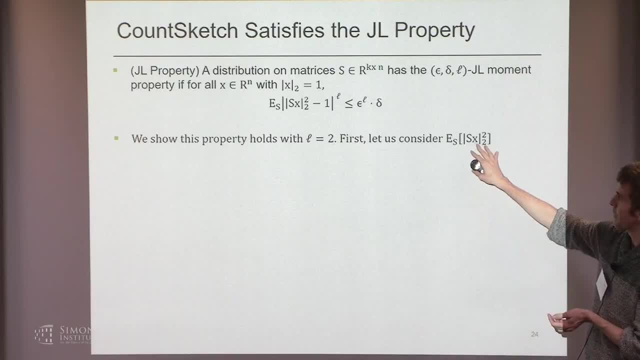 uh, go through this very quickly. so, um, let's first just consider the expectation of the square number of SX. Is it unbiased? So we want this to be 1, right, Um? so for count sketch matrix S. 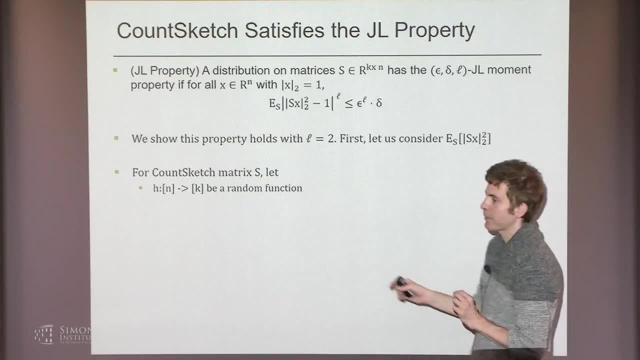 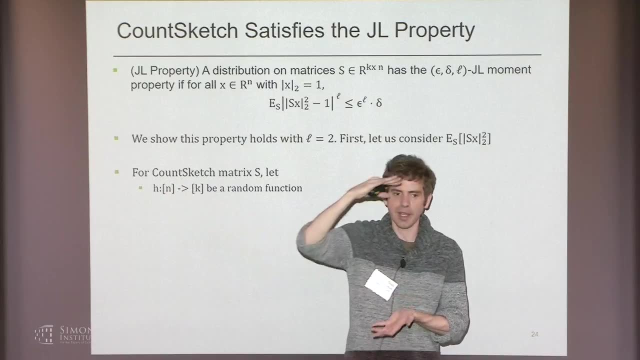 it's convenient to parameterize it in terms of two things. One is a hash function, H, which specifies for each column where the non-zero entry is. Okay, so it's telling me where each non-zero entry is, And there's also a sine. 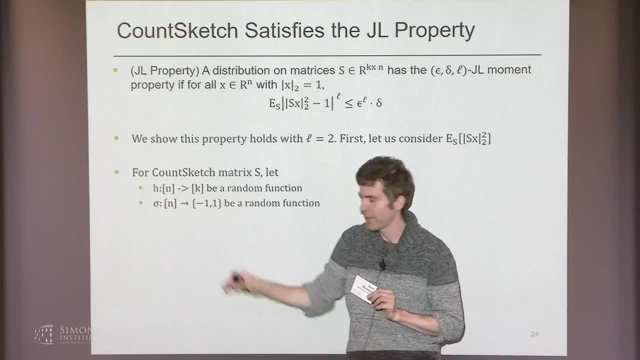 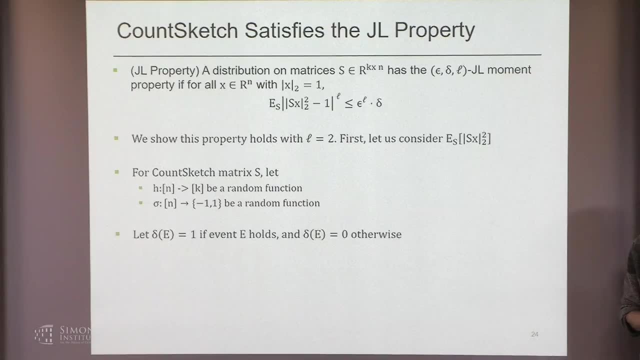 function. So for each column, the sine function sigma tells me the value on that non-zero entry. Is it 1 or is it minus 1?? Okay And uh, let's just let delta of E be 1, if some probabilistic 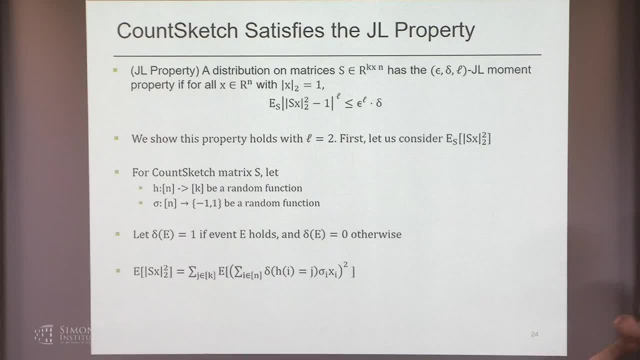 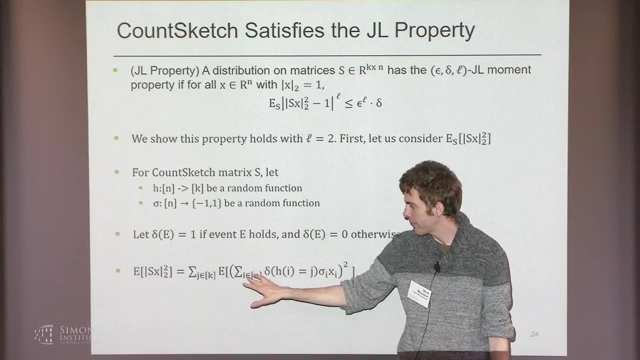 event E holds um straightforward. So the expected squared norm of Sx? well, it's the sum over the k coordinates of Sx of the squared value on that on the coordinates. So what is the squared value on the coordinate? 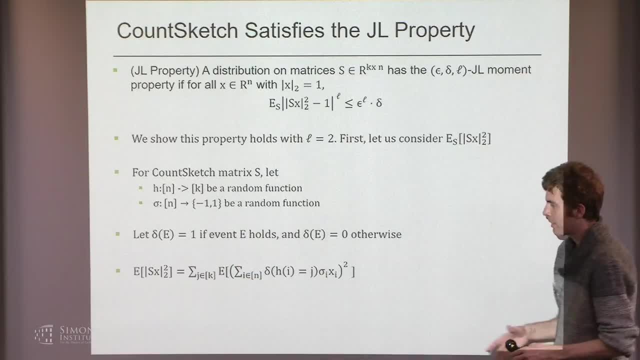 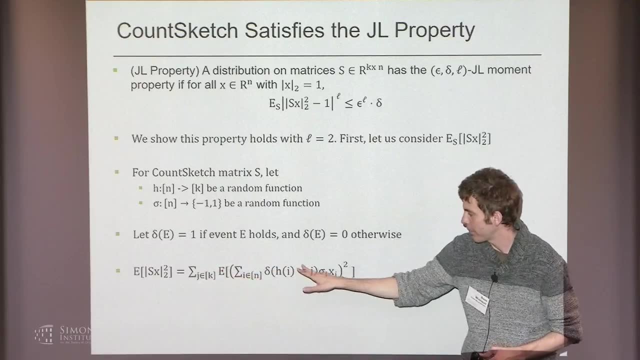 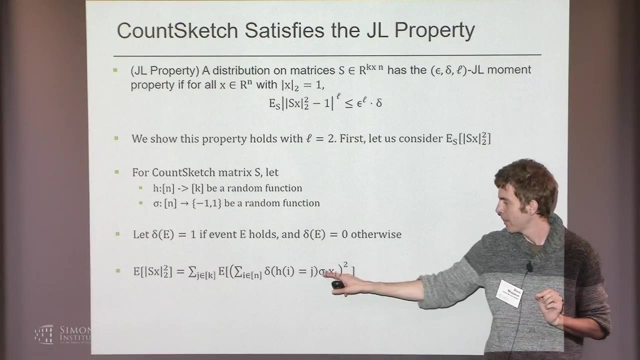 Well, it's the sum over all indices i between 1 and n. First I need an event that actually the uh, the ith column had its non-zero entry. Then I multiply by the sign associated with that non-zero entry, sigma i. 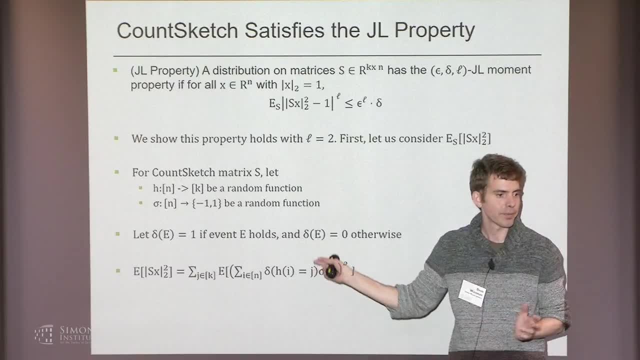 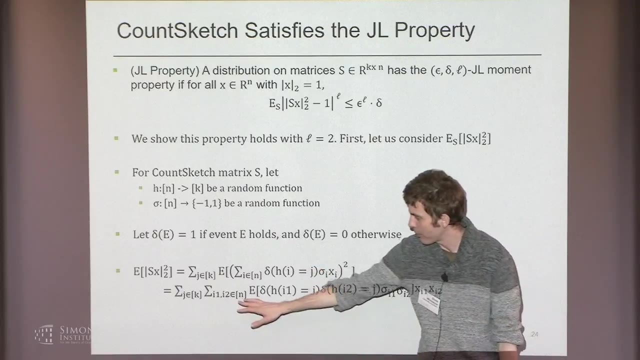 times the actual value xi, And since I'm computing the squared norm, I'm taking the square of this. Okay, So let's just expand the square on the next line. So all I did now is I expanded this and I have a. 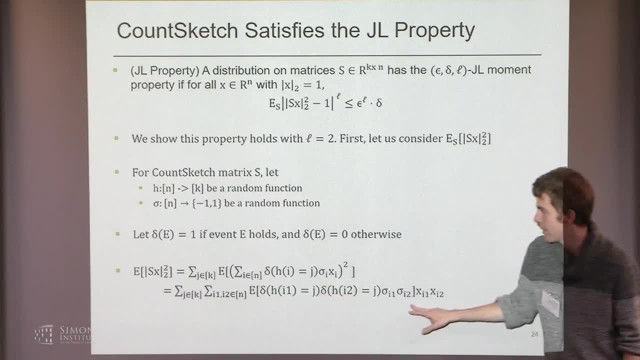 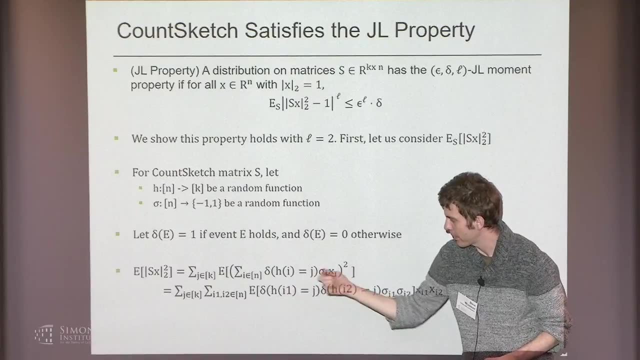 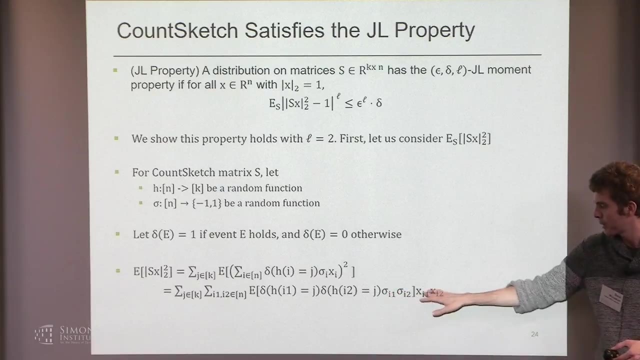 sum over all pairs of indices i and a squared running xico. So I have this expectation, you know, of the product. uh, you know, I have two of these things now. So indicator that the i one coordinate hashes to the jth. 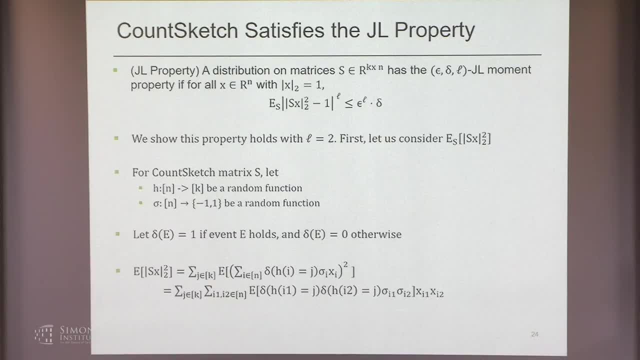 bucket and the i two coordinate hashes to the jth bucket times: sigma i one, sigma i two times. then what is the expectation of this quantity here? Zero right, Because these are random signs. i1 is not equal to i2.. It's at least pairwise independent. 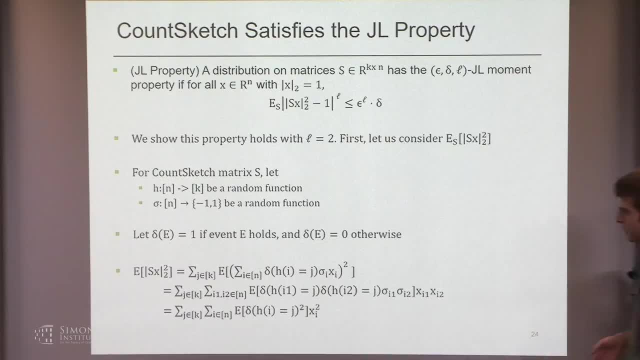 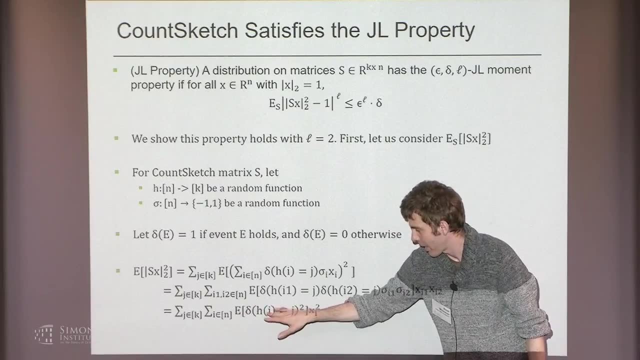 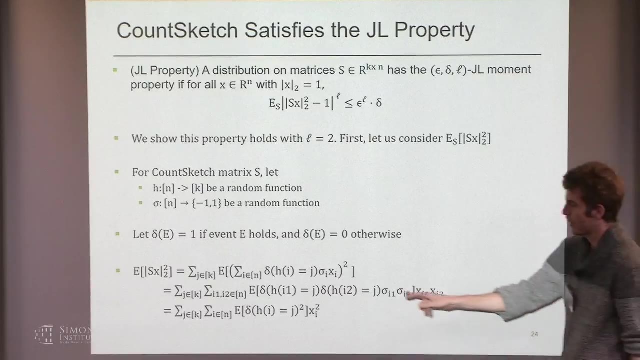 The expectation is zero. So instead you just get a sum over all indices i of the expectation that this indicator squared. you know that the ith entry gets hashed to the jth bucket times xi squared. What is the expectation of this? What is this expectation? 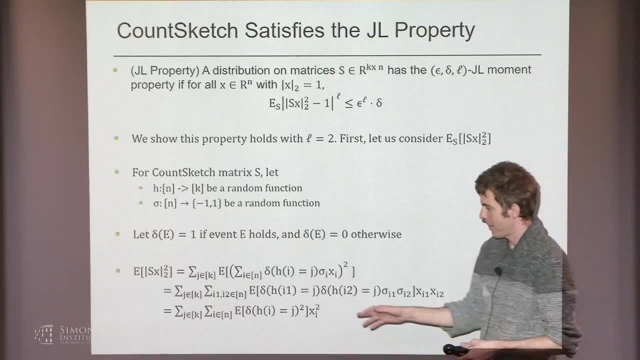 It's just the probability that the ith coordinate, you know the ith column, has its non-zero entry in the jth row. What is that probability? 1 over k, the number of rows, right. So this is 1 over k. 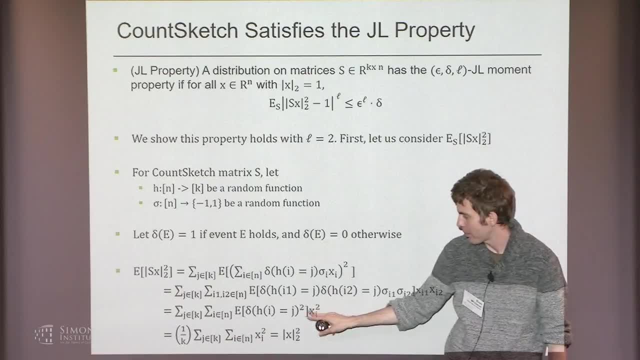 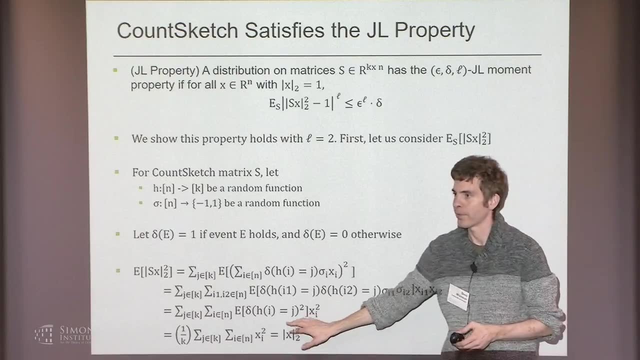 And I'm summing over k things Each one of them. I'm getting the sum of squares of all the entries, So I get an unbiased estimator right. The squared norm of sx is the squared norm of x. Okay, So okay. 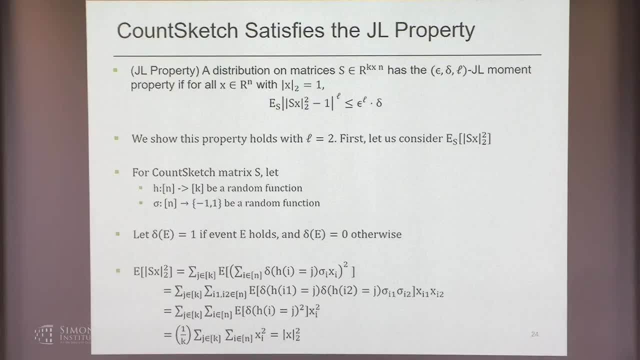 So it's 3 o'clock now. Yeah, why don't we take a break for half an hour and I'll you know when we come back. we'll conclude with showing that count sketch has the jlmoment property and then we'll start looking at other problems. Thank you.